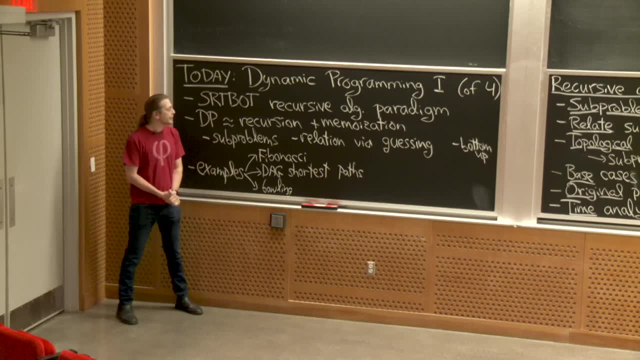 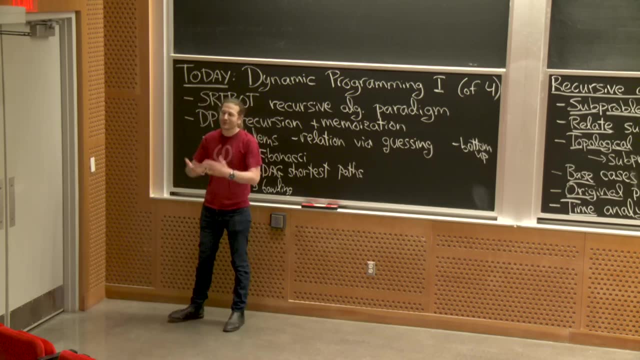 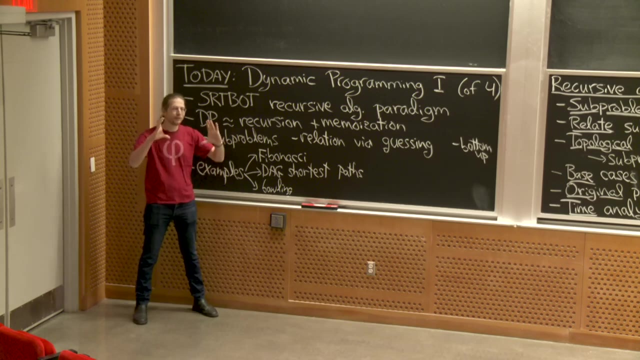 very general, can solve lots of problems. It's a particular type of recursive algorithm design And, in general, this class, all of algorithms, is about recursive algorithm design at some level, because we want to write constant size pieces of code that solve problems of arbitrary. 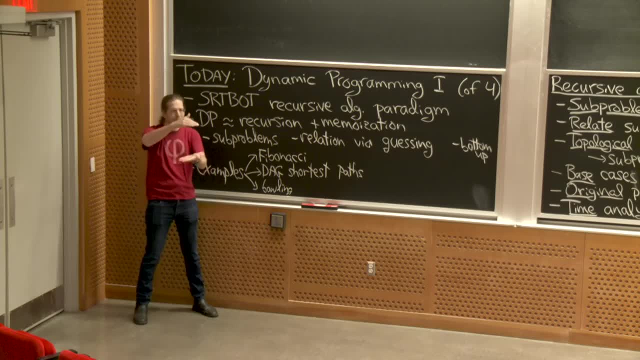 size. We have some problem size n and we're trying to write, you know, 100 lines of code or whatever, some constant amount that doesn't depend on the problem size. We have one algorithm that solves all instances of the problem, And so we have to write code that is recursive. 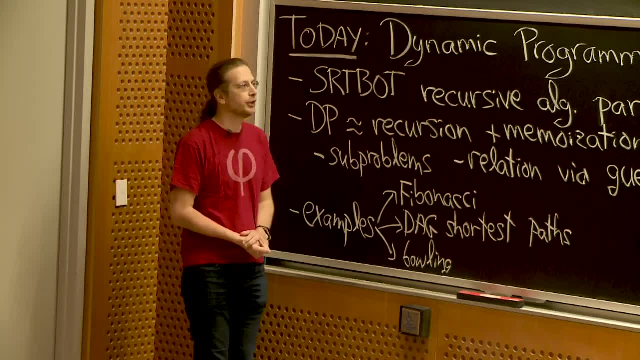 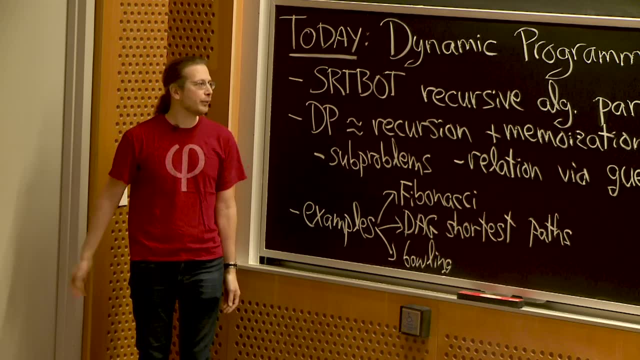 or uses loops or somehow reuses the instructions that we give the computer. And you may know, you can convert any algorithm based on loops into an algorithm using recursion, And we're going to take the recursive view today, in particular because it fits very well with 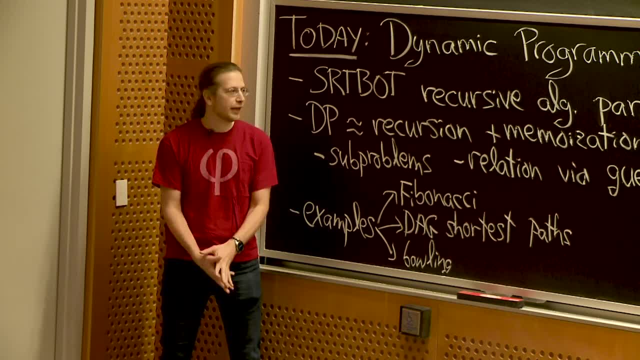 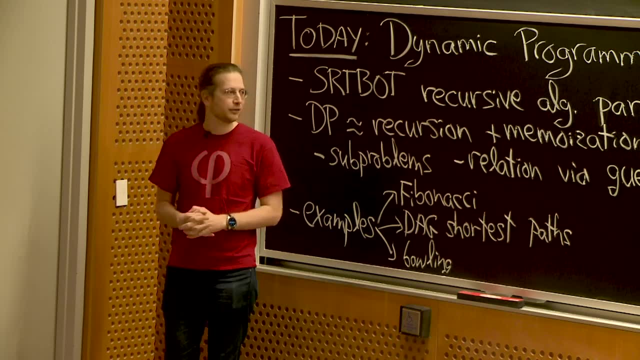 our algorithm. It fits very well with our proof by induction technique, which we've used throughout this class, but also because it gives us some structure on how different subproblems relate in something called a subproblem graph that we'll be talking about today, And so we're going to start out. 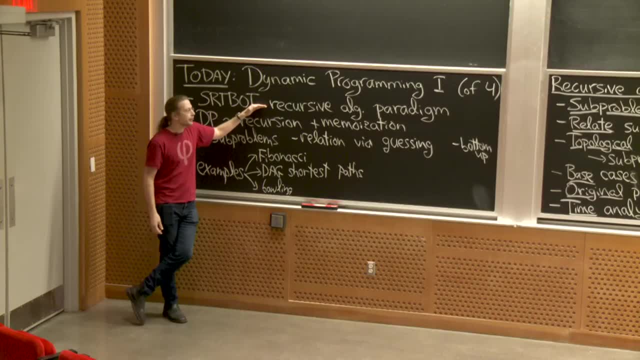 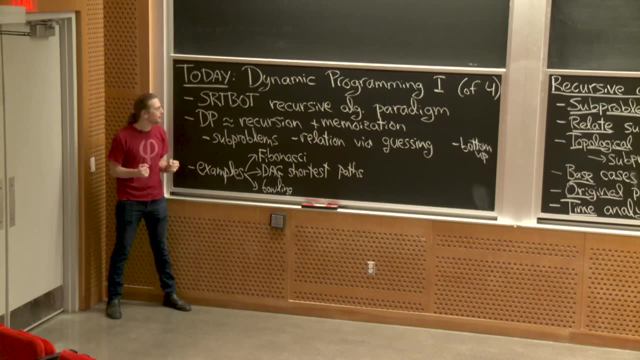 with in general. how do we design recursive algorithms? That's sort of the overall encompassing everything. We have thought very hard to come up with a cool acronym for this paradigm, which we invented, called SORTBOT. Thanks, Jason. And so it's not actually for sorting, It's just an acronym for subproblems. 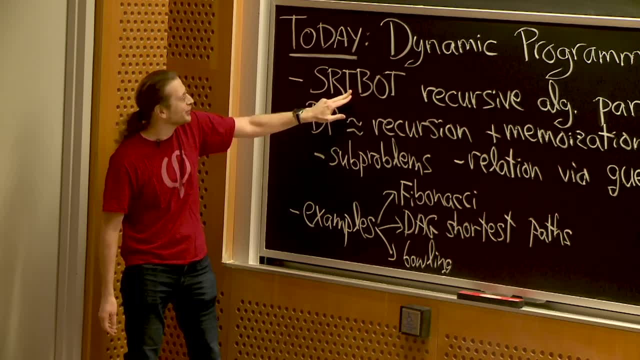 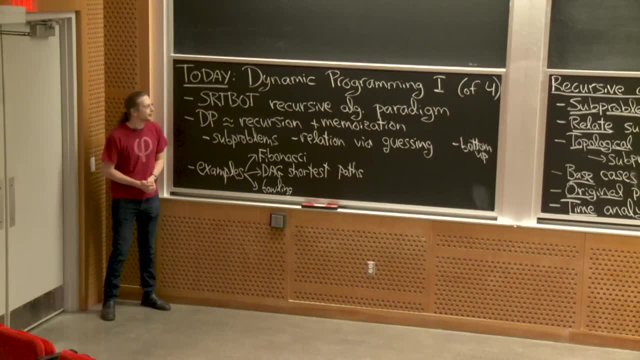 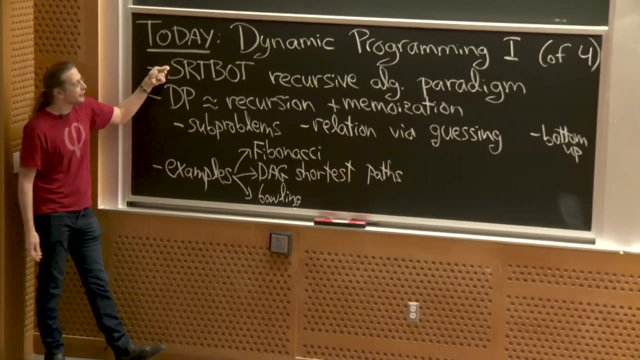 relations: topological order: base, case, original problem and time, But it's an acronym that will help you remember all the steps you need in order to specify a recursive algorithm, And dynamic programming is going to build on this template by adding one new idea called 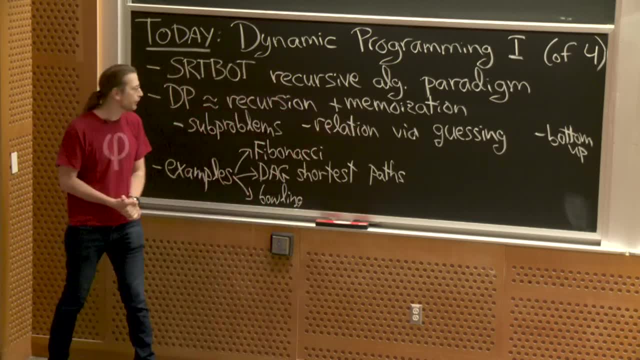 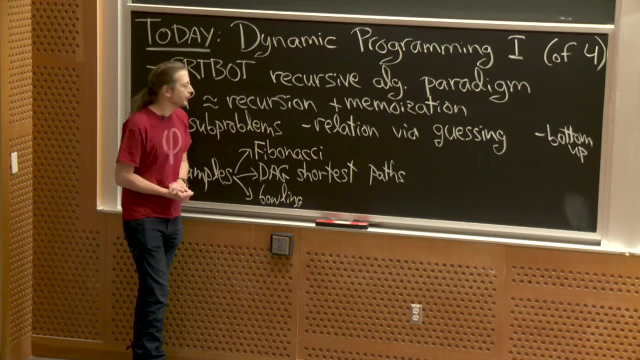 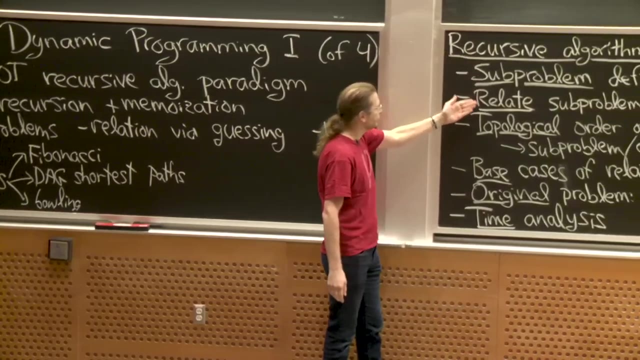 memoization, Which is just the idea of reusing work that you've done before And that's going to let us solve tons of problems And let's see, Let's get into it. So we'll start out today with SORTBOT. So here is SORTBOT, down the column, here This. 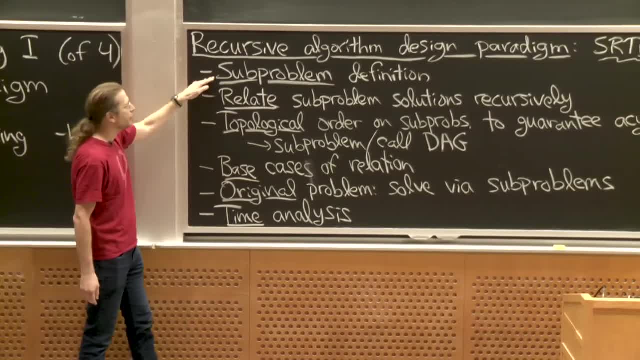 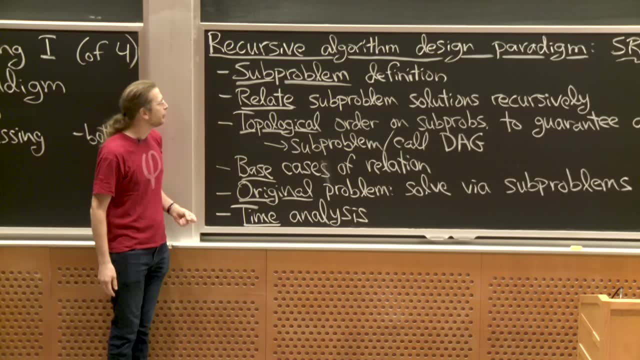 is a recursive algorithm design paradigm And, in general, what we're going to do is take the problem that we actually want to solve and split it up into lots of possible problems, And so the first part is to define what the heck are the subproblems In general. 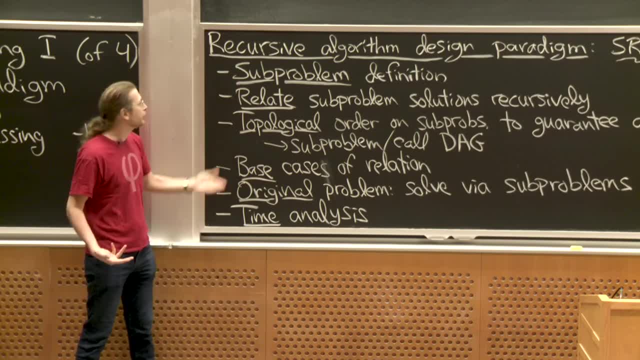 we'll want some polynomial number of them, But it's pretty open-ended what these look like, And the hardest part usually in defining a recursive algorithm is figuring out what the subproblems should be. Usually they're related to the problem you want to solve. 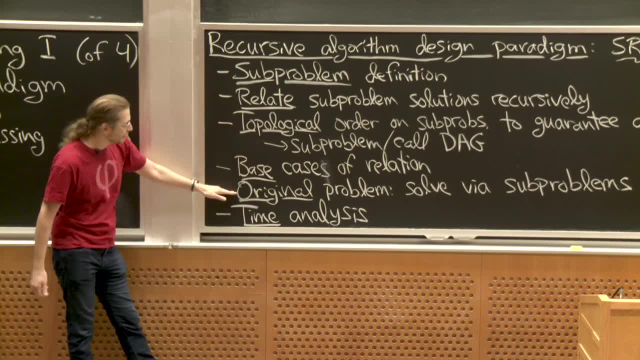 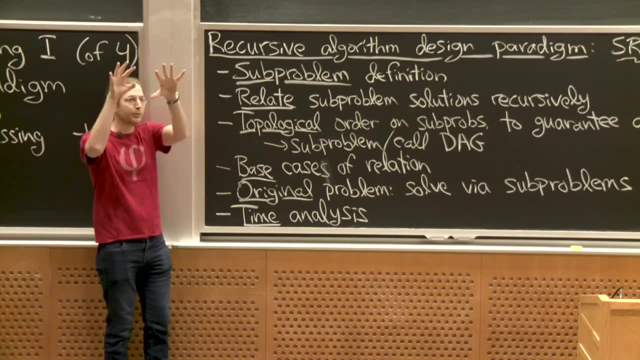 Often the problem you want to solve this is actually near the last step. the original problem you're trying to solve is often one of these subproblems, And then you use the smaller subproblems And then you sort of build up the final original problem. But sometimes at the end you need 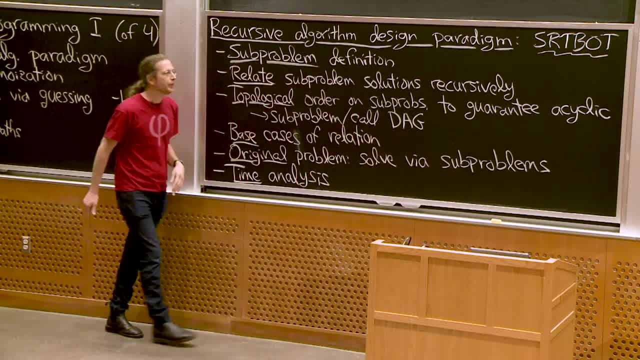 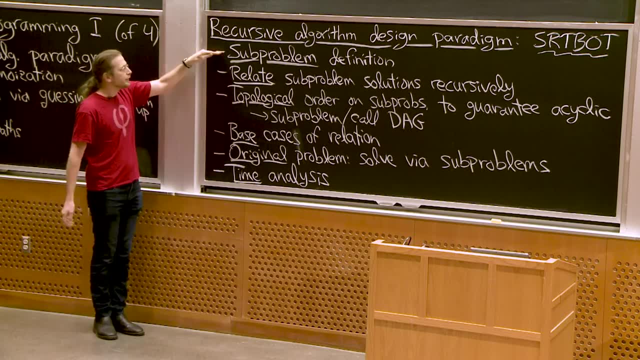 to take a bunch of subproblems and combine it into your original problem. One analogy you can think of here is divide-and-conquer algorithms, which also had this kind of style. But more generally we're going to relate different subproblem solutions with some recursive. 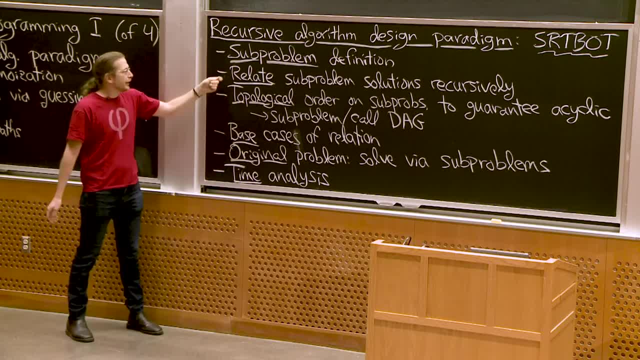 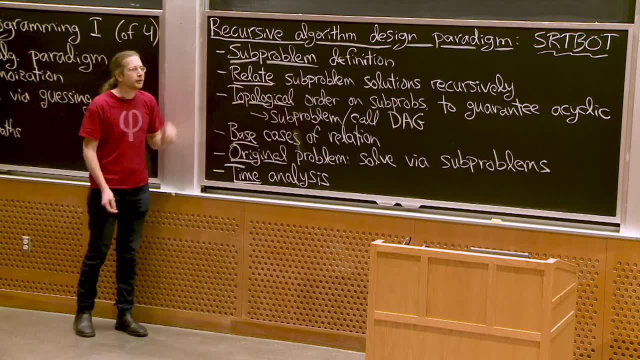 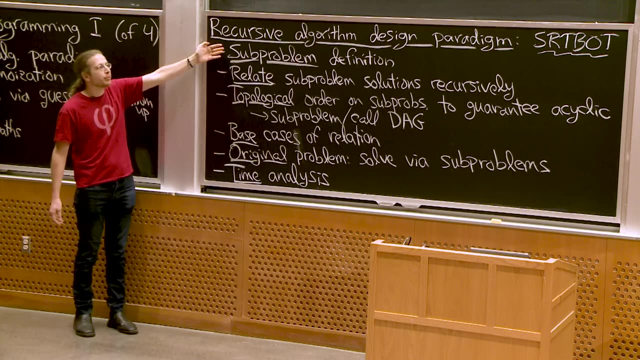 structure, some recurrence relation. This is just a recursive algorithm that defines how to solve. So we're going to look at one problem in terms of smaller subproblems, for some notion of smaller, And this is given by the topological order. So if we think of the subproblems as a graph, 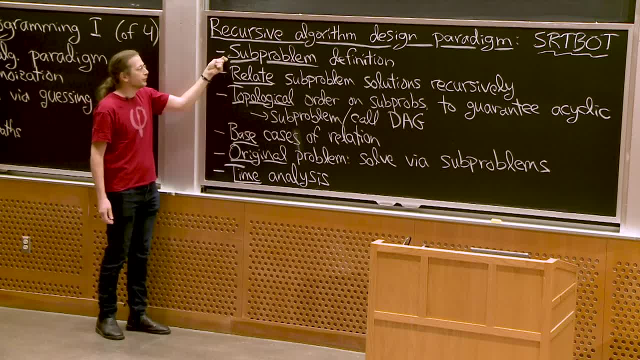 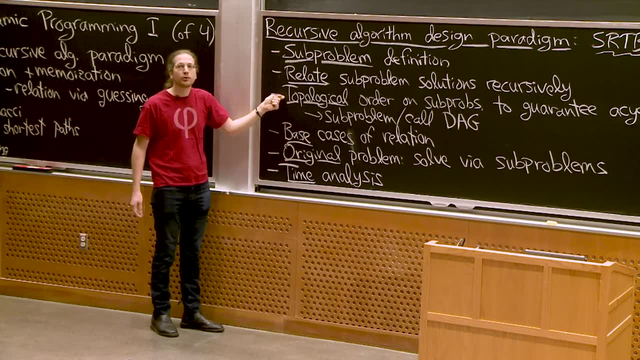 and we draw an edge between. so the vertices of the graph are subproblems, The edges are the dependencies between those subproblems. Then what we'd like is the topological ordering, the topological sort problem we talked about in the context of DFS or DAG: shortest paths. 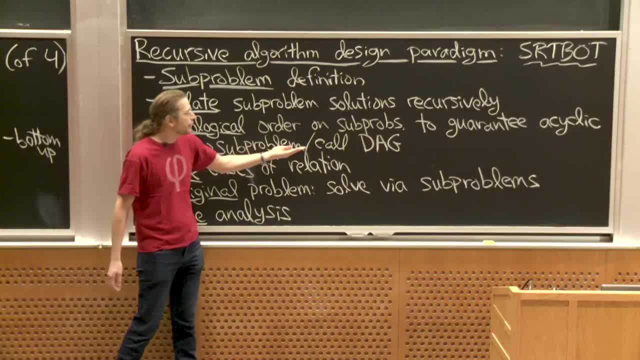 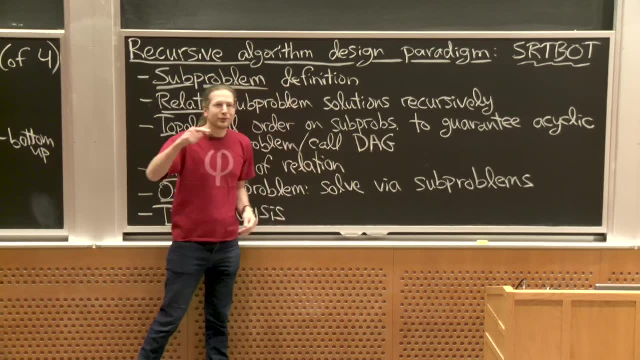 What we would like is that this And that's all about, And then we would like to draw a sequence of these subproblems. So, in today's analysis, these subproblems and the calls, the recursive calls between them, in this recursive relation forms a DAG. 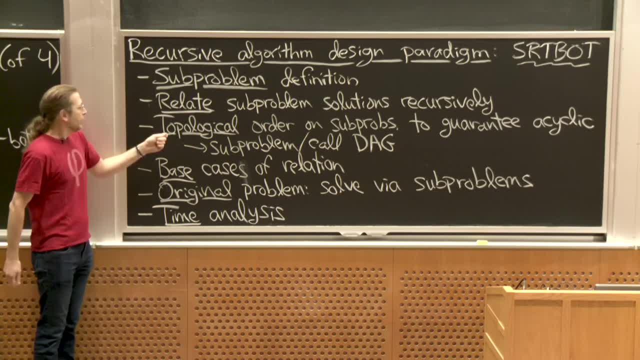 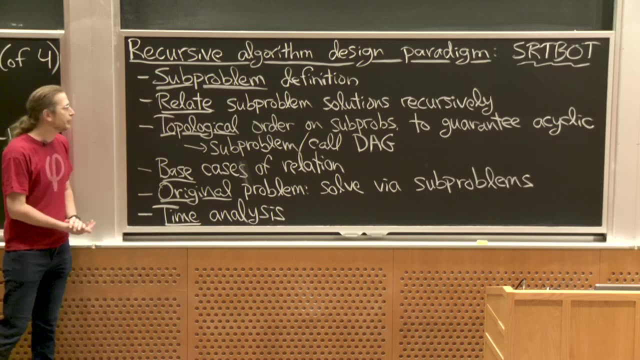 We want it to be acyclic, otherwise you have an infinite loop in your recursive calls. If you have a cycle, you'll never terminate, And so, to make sure that these dependencies between subproblems given by this recurrence relation is acyclic, one way to do that is to specify a topological order. 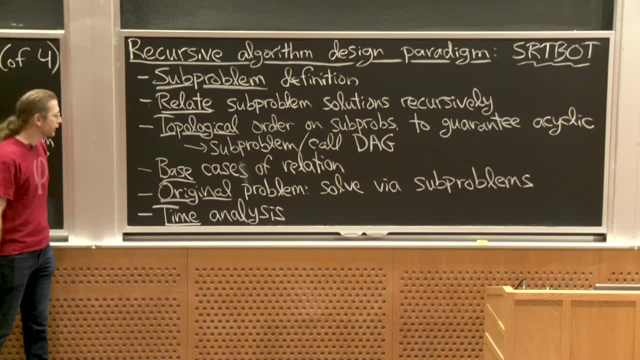 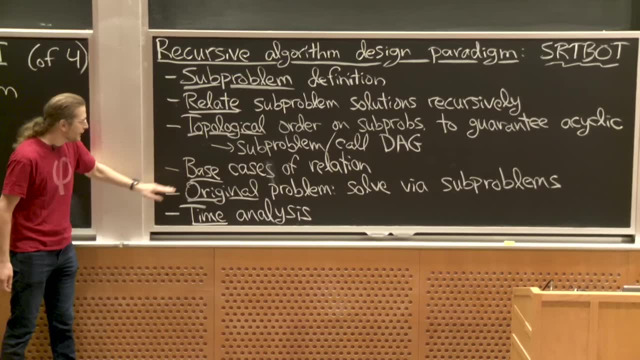 is just a for loop to say: just do it in this order. Then, of course, any recursive structure needs base cases. So that's a useful step not to forget. We want to solve the original problem using these subproblems, And then we analyze our running time at the end. 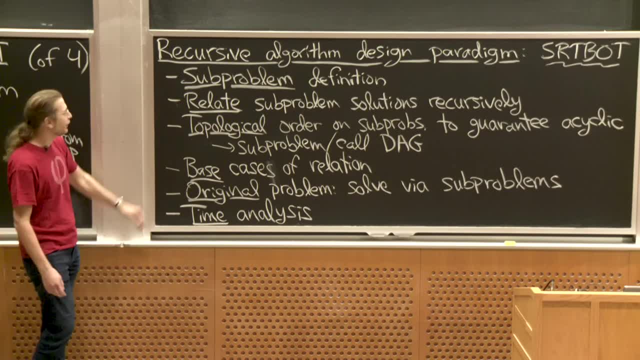 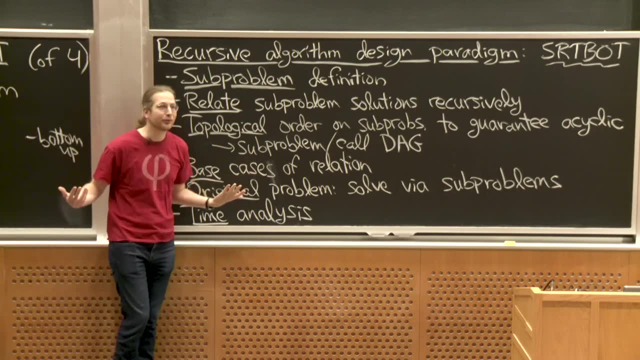 So six easy steps. Actually, the hardest ones are these two, which are interrelated, And what we're going to see over the next four lectures- this is the first of four lectures on dynamic programming- is lots of examples of applying this paradigm over and over. 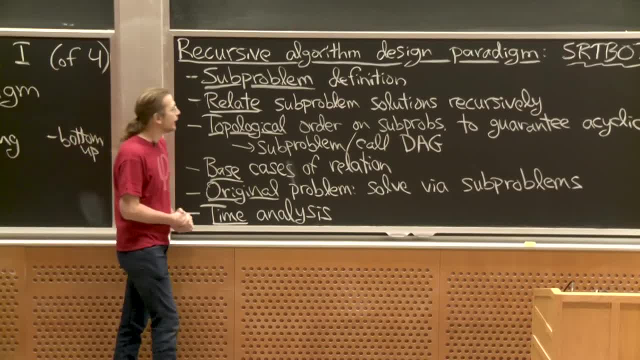 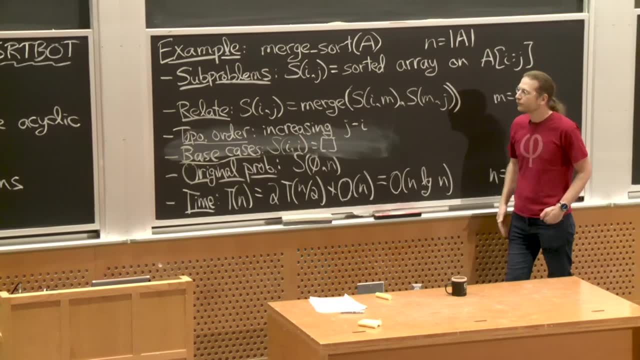 together with the memoization idea which we'll get to soon. Let's see an example, first, of an algorithm we've already seen which is merge sort, so a divide and conquer algorithm phrased with this structure of sort bot, So for the subproblems, so our original problem. 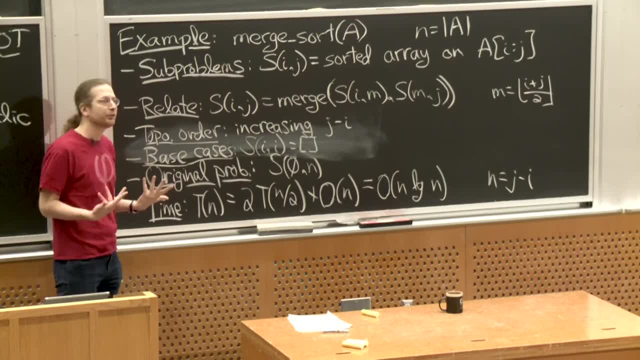 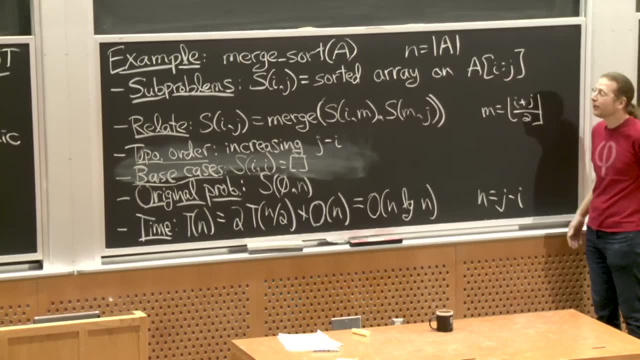 is to sort the elements of A, And some subproblems that we solve along the way are sorting different subarrays of A. So for every- well, not for every- i and j, but for some i and j's, we sort the items from i up to j minus 1.. 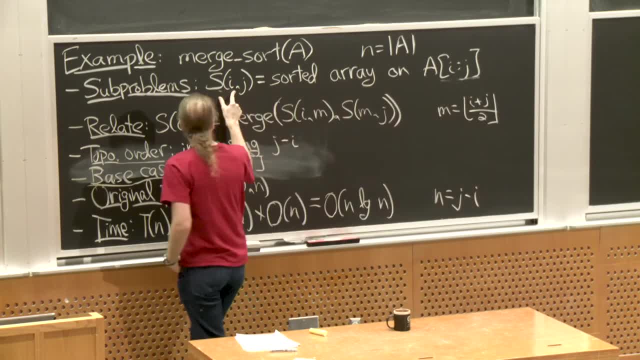 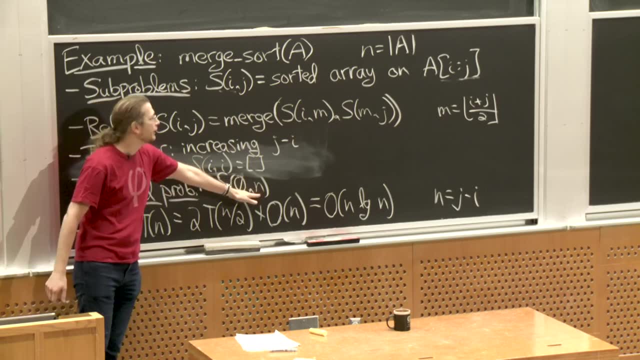 So I'm going to define that subproblem to be s of ij. So this is something that I might want to solve. The original problem that I want to solve is s of 0 comma n, where n is the length of the array. 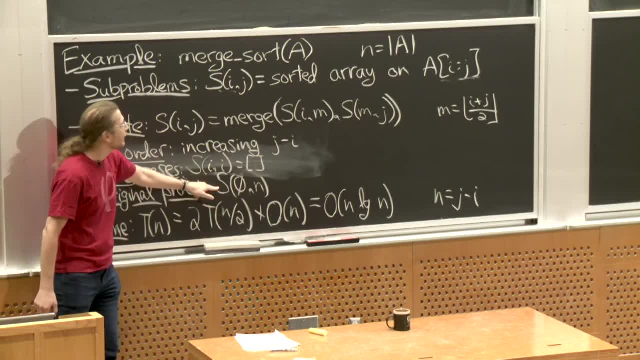 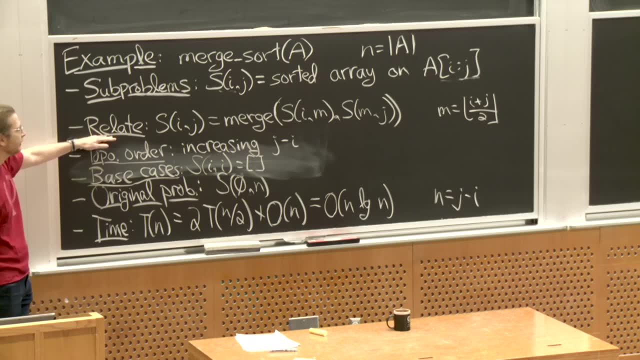 So that's what I actually care about in the end, But we're going to solve that by writing it recursively, in terms of sorting different subarrays as follows: This is the recurrence relation. I've written it very simply here. Of course, there's a merge algorithm. 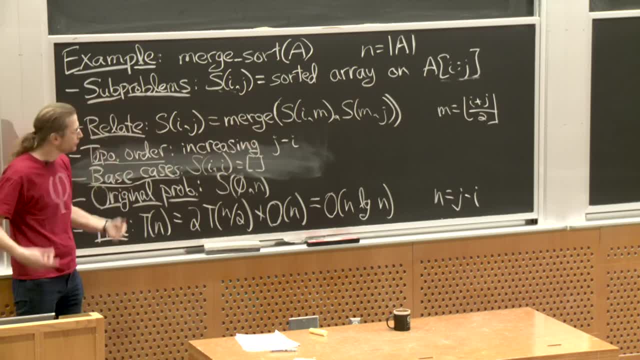 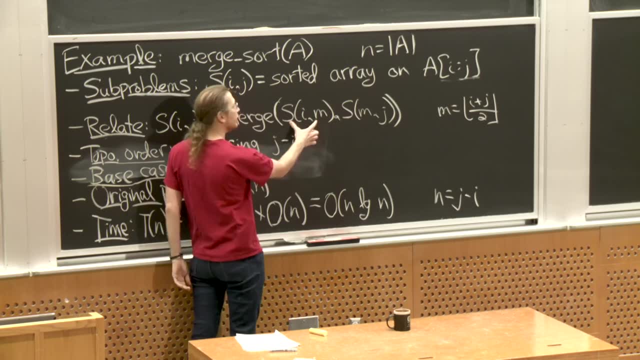 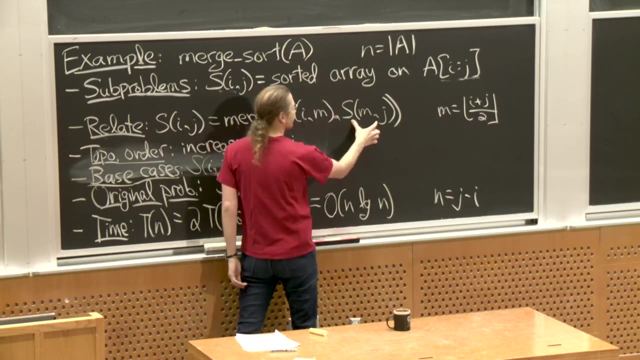 which is somewhat complicated, But we saw the two-finger linear time merge algorithm given two sorted arrays. So this is supposed to be the sorted array version of the items i through m. m is the middle element between i and j And the sorted array of the items from m up to j. 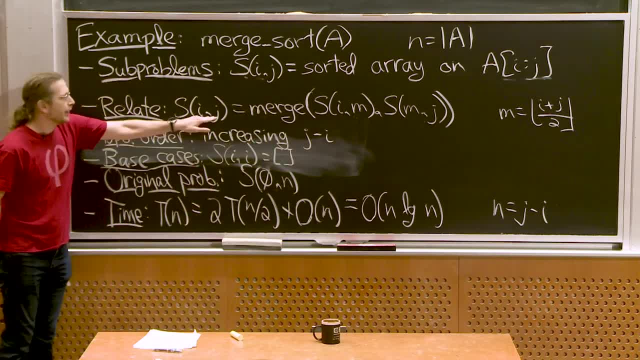 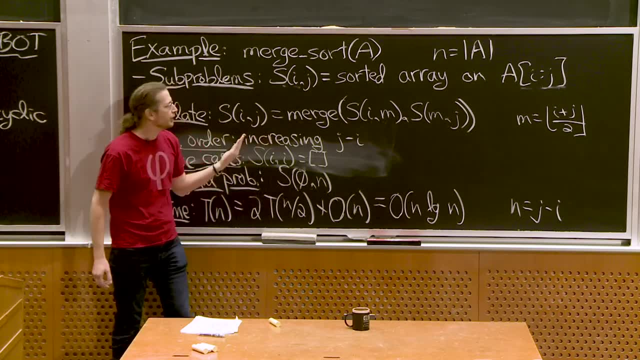 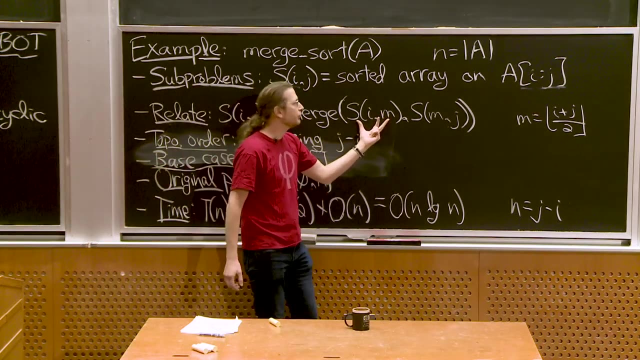 If we merge those, that gives us the sorted array from i up to j, And that's exactly what merge sort does. So this is in general. this relation is just some algorithm, for if you're given the solutions to some smaller subproblems. 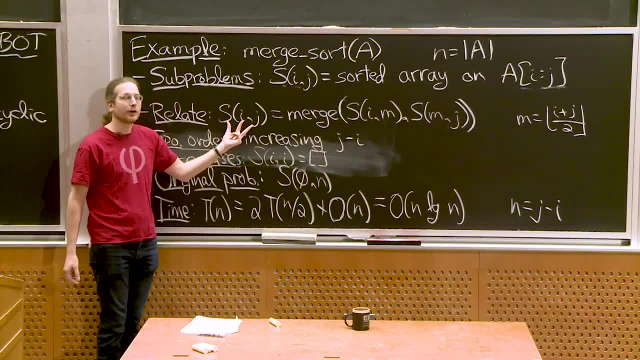 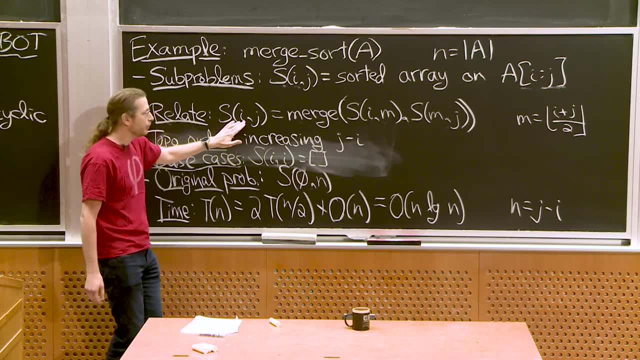 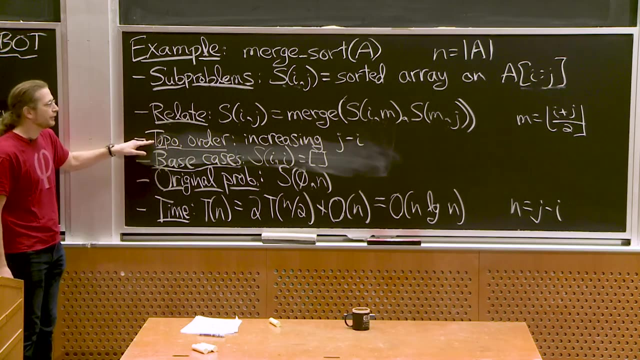 how do I solve the subproblem that I want to solve? And so we need to make sure that this problem is bigger than the ones that we recursively call on and that we don't get an infinite cyclic loop of recurrence And here a valid topological order. 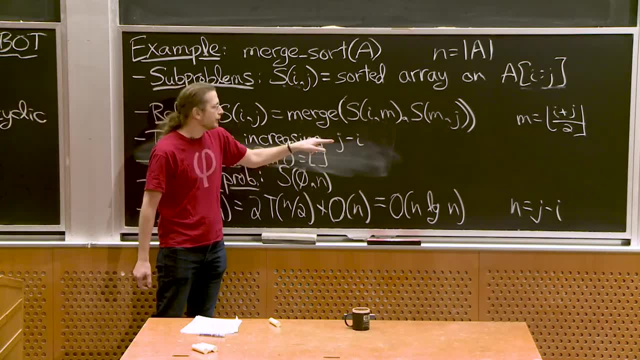 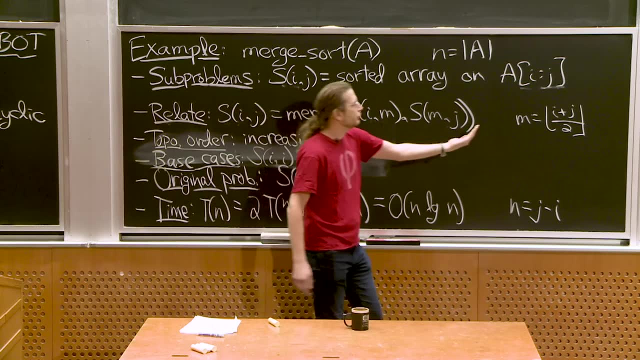 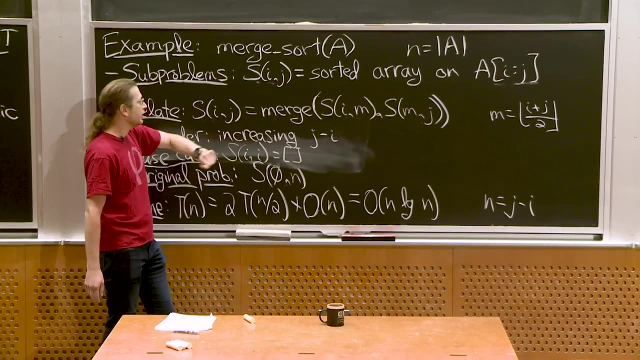 is to say solve these problems in order where j minus i, the length of the subarray is increasing. And then you can check, because m is strictly between i and j. As long as we're not in a base case, then we know we can. 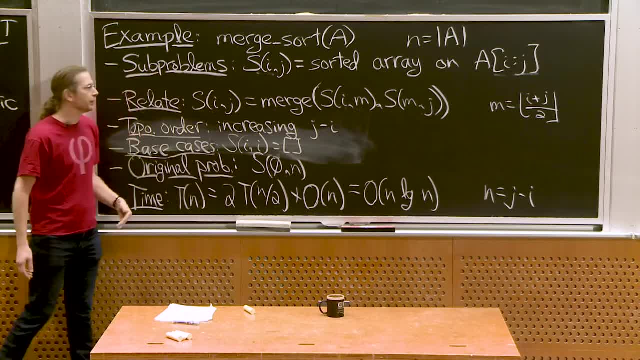 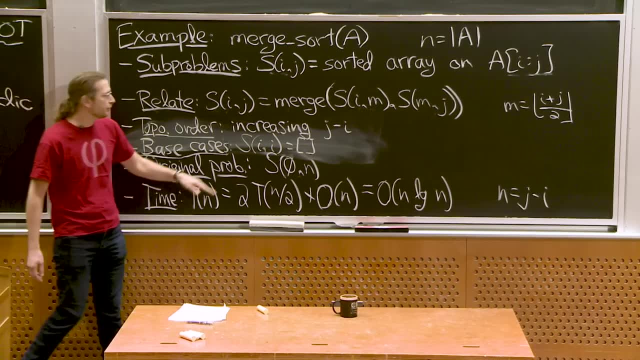 These subarrays will be smaller than this one, And so this increasing order gives us a valid topological order. on all of the problems, all the subproblems, We have a base case which is, if we don't want to sort anything, that's the empty array. 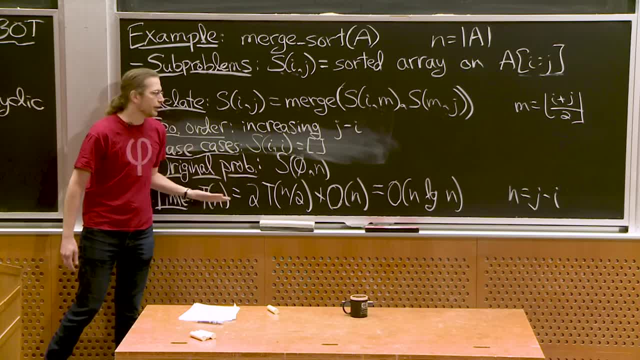 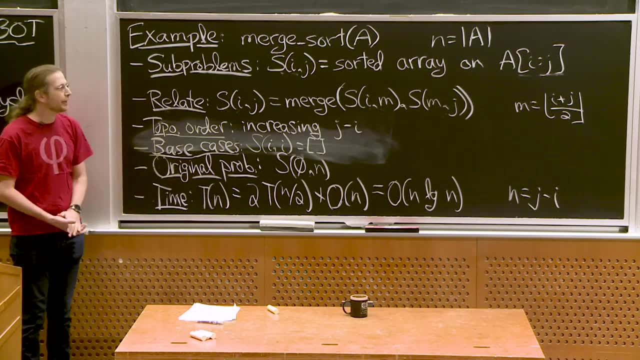 I already said, the original problem And then running time is, I mean, there's no better way to solve it than the recurrence that we already saw how to solve. So this is just another way to think of n log, n merge, sort in this labeled framework of sort bot. 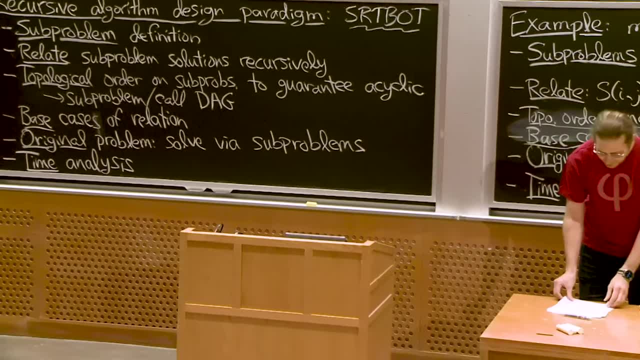 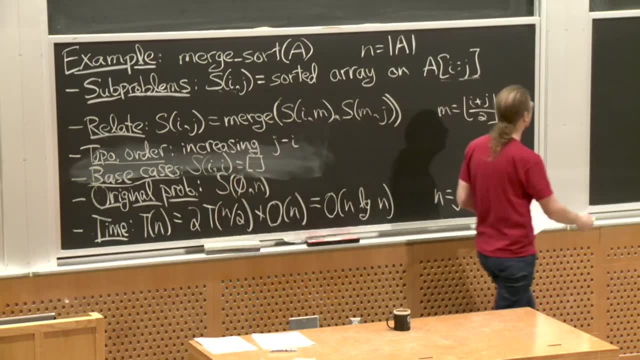 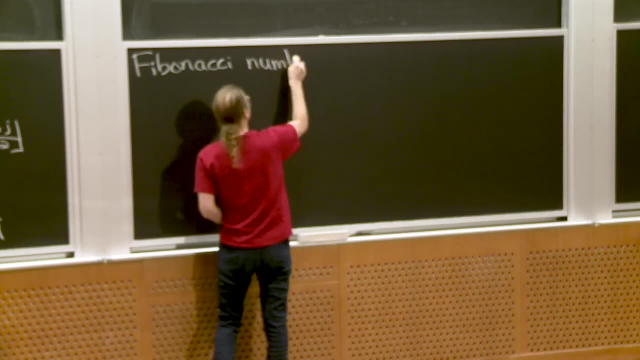 Let's get to another problem that does not fit recursion so well, but we can make it better. So we're going to start with a very simple problem, which is computing Fibonacci numbers. It's really just a toy problem to illustrate a very powerful idea, which is memorization. 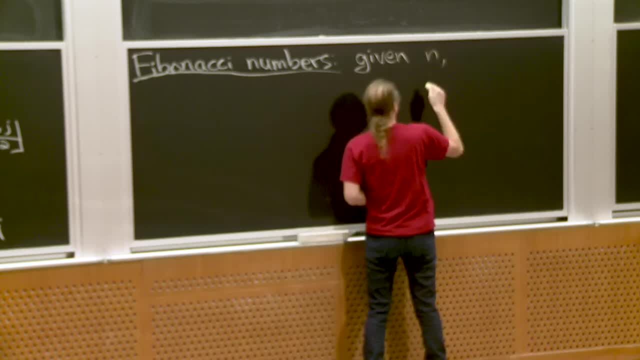 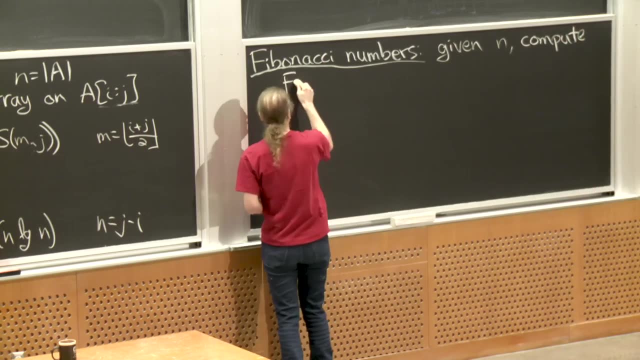 So the problem I'm interested in is: I'm given a particular number, n, And I want to compute the n-th Fibonacci number. And, in case you forgot, the n-th Fibonacci number is given by this recurrence Fn is Fn minus 1 plus Fn. 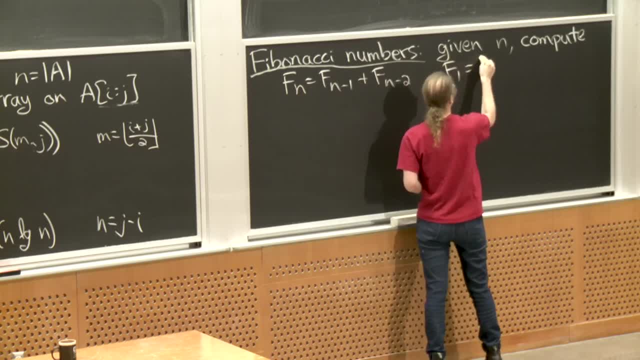 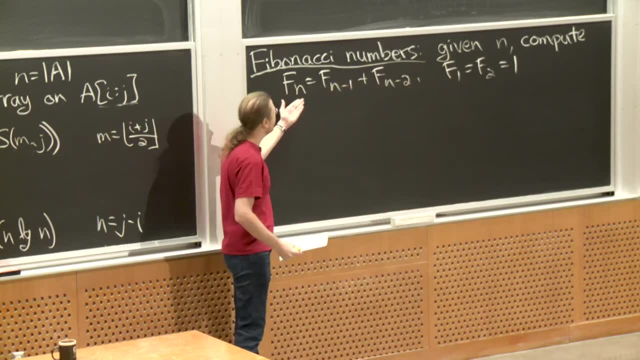 Fn minus 2. with base case, let's say F1 equals F2 equals 1.. And so we'd like to compute this: This seems this is a recurrence, So it seems very natural to write it as a recursive algorithm. 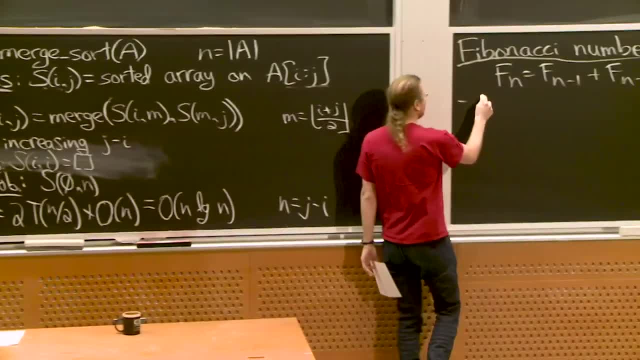 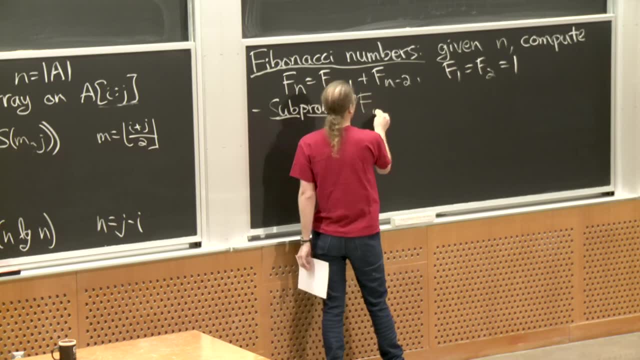 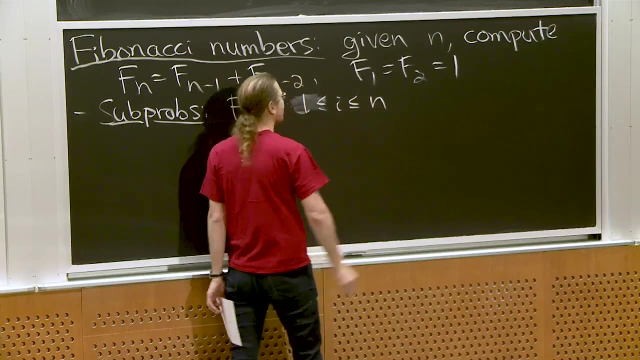 So let's try to do it. We start with. what are the subproblems? The obvious subproblems are just the various Fibonacci numbers: Fi for i, between Between 1 and n. So there are n of these subproblems. Cool. 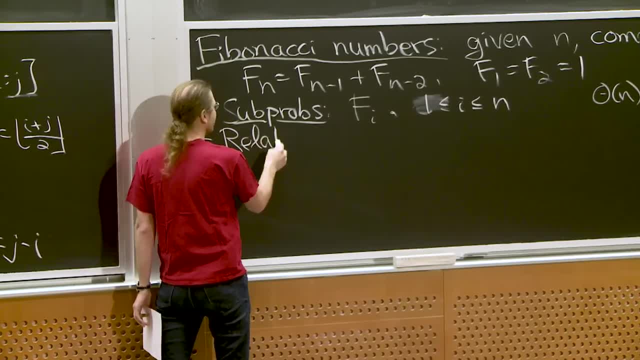 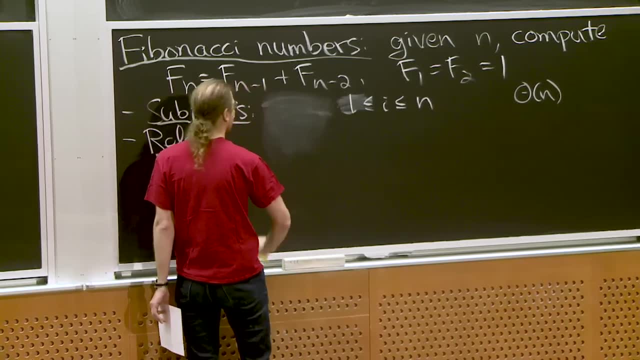 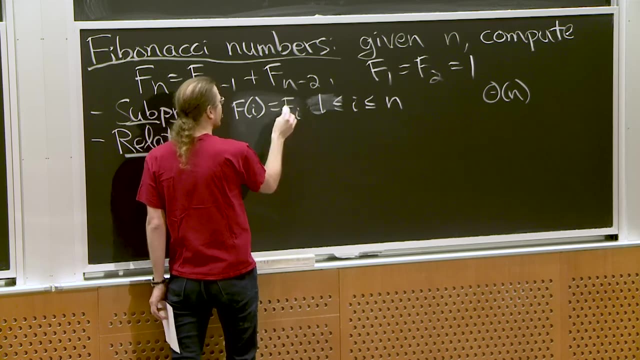 Let's see. we want a relation between them. Well, maybe I'll just to distinguish the problems from the Fibonacci numbers, let me write f of i. This is a function, an algorithm we're going to define, And it's defined to be the goal we're trying to get. 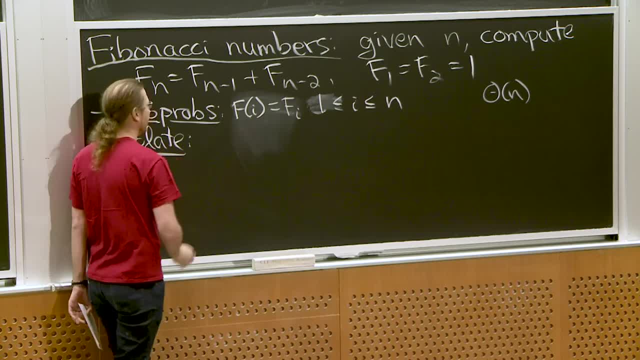 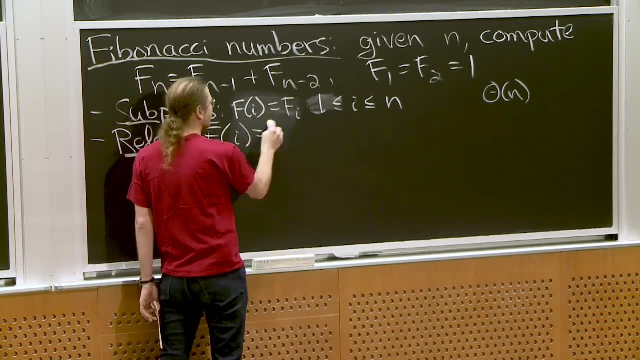 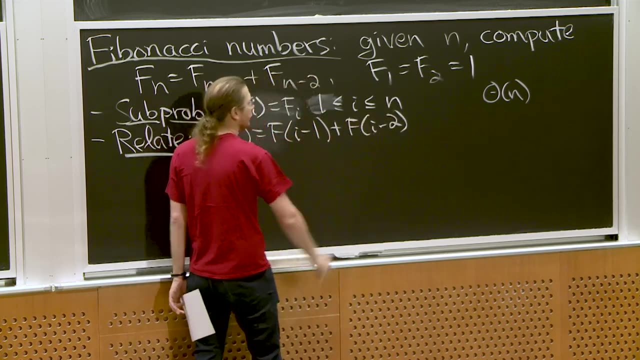 is the n-th Fibonacci number, OK, Is the i-th Fibonacci number given i? And then we can write the recurrence relation on these guys: just F of i equals F of i minus 1 plus F of i minus 2.. So in other words, recursively compute those Fibonacci numbers. 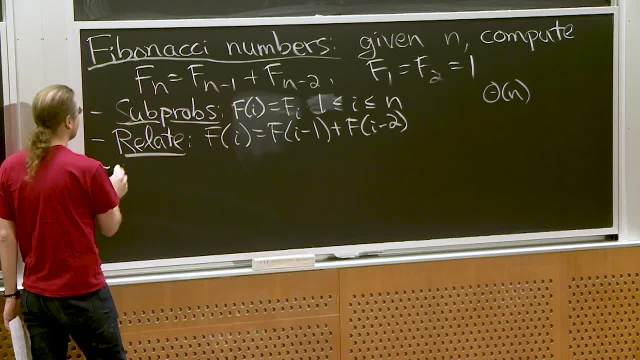 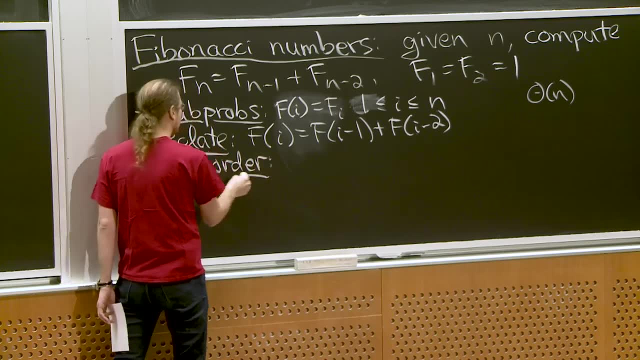 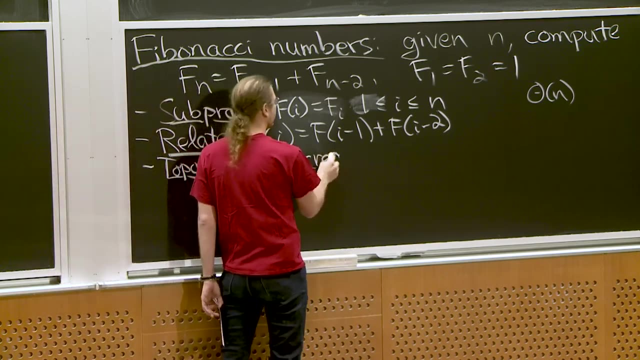 then add them together. That's an algorithm. Next is T for topological order. Here, of course, we just want to. We want to compute these in order of increasing i from the base cases up. Another way I like to write this is as a for loop. 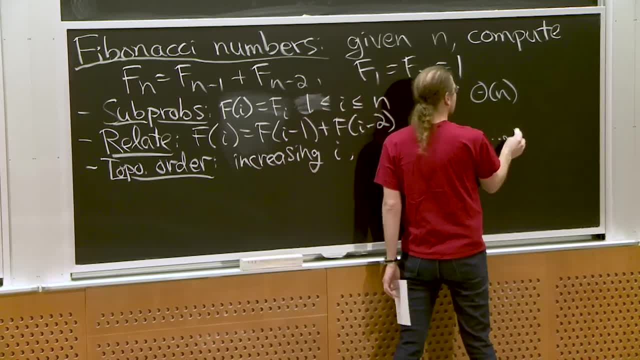 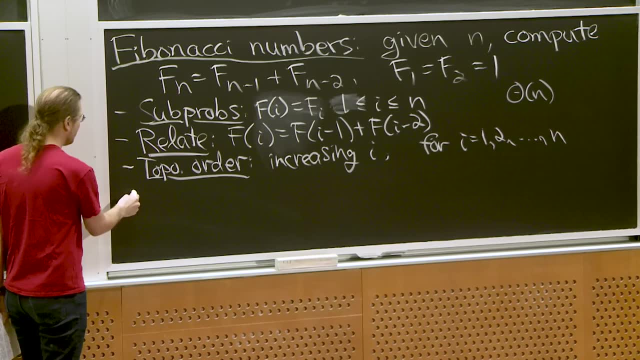 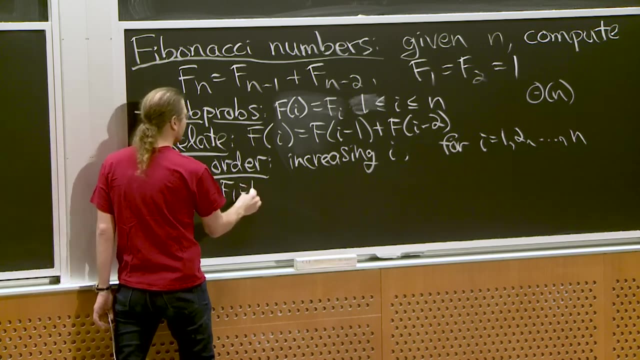 For i equals 1 to n. Maybe we'll see why, But this gives an explicit order to compute these subproblems And all right. base case is just the same As the Fibonacci numbers, But I guess I should write parentheses. 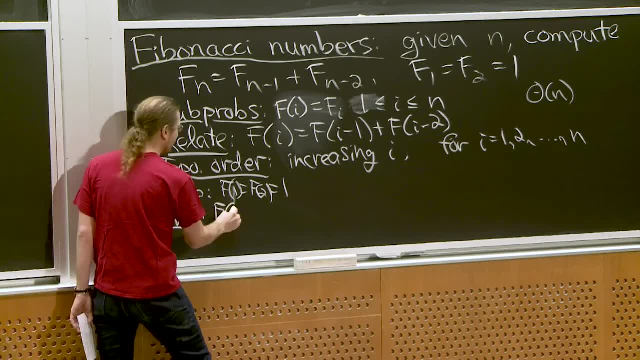 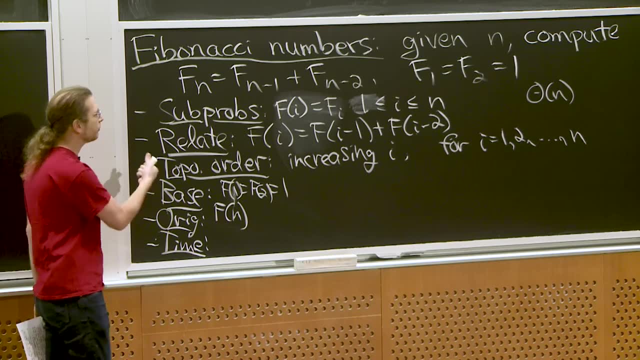 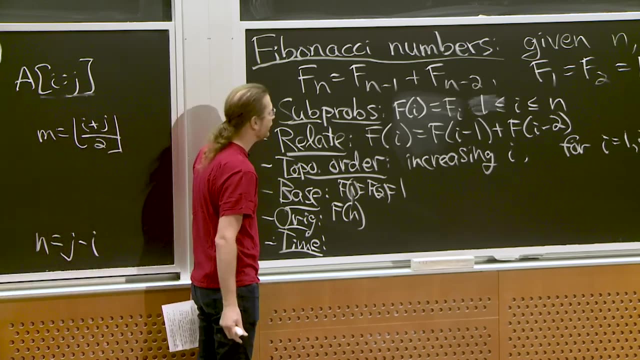 The original problem we want to solve is F of n And the time all right. here's where things get interesting or bad. So what is the running time of this recursive algorithm? As I've stated it so far, the running time is given by a recurrence. 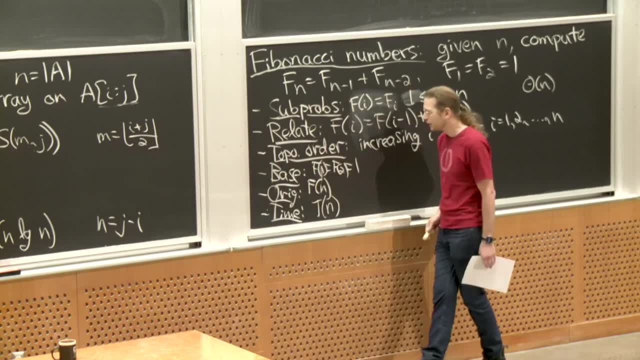 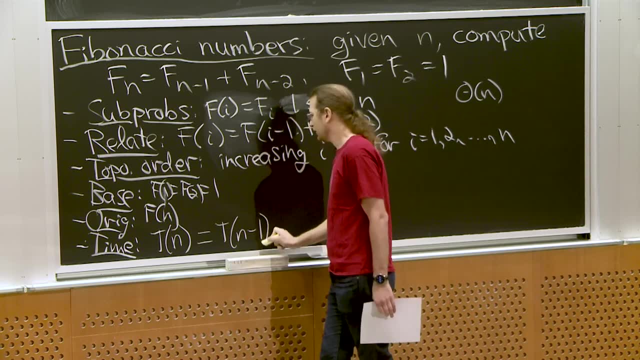 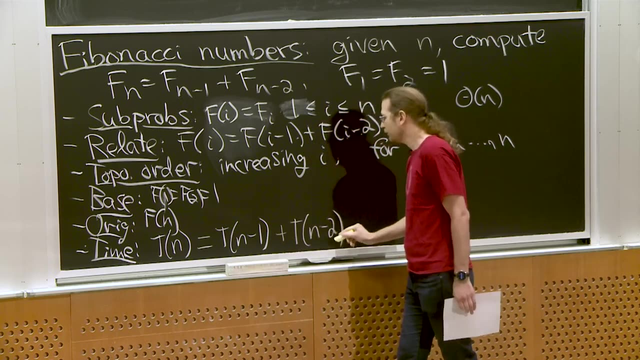 Let's write the recurrence So in order to compute F of n. OK, So I recursively compute F of i minus 1 or F of n minus 1 here, And I recursively compute F of n minus 2.. So that will take T of n minus 2.. 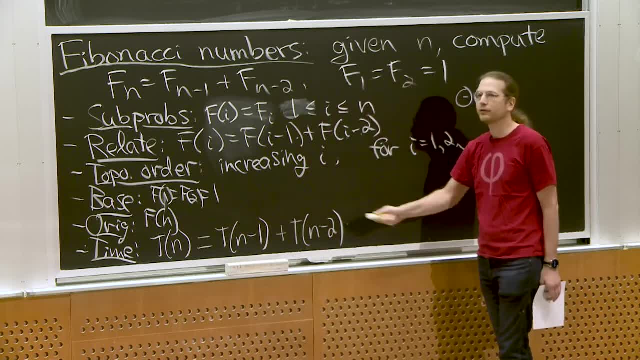 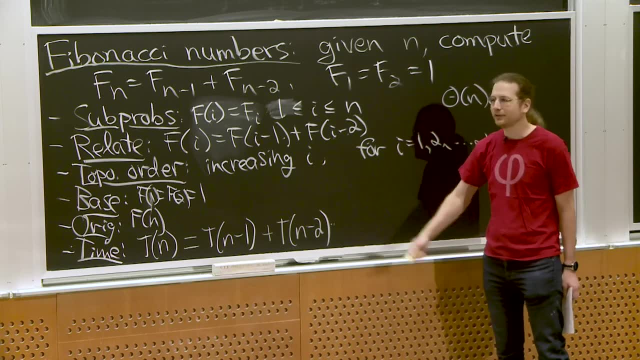 This first step will take T of n minus 1.. And now I need to solve this recurrence. This is not a recurrence that falls to the master method. It doesn't have a divided by, So we have to think about it a little bit. 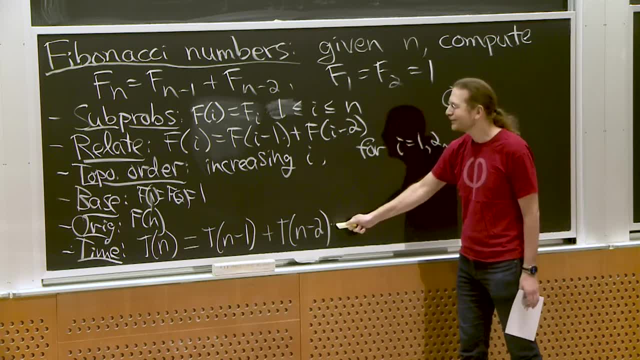 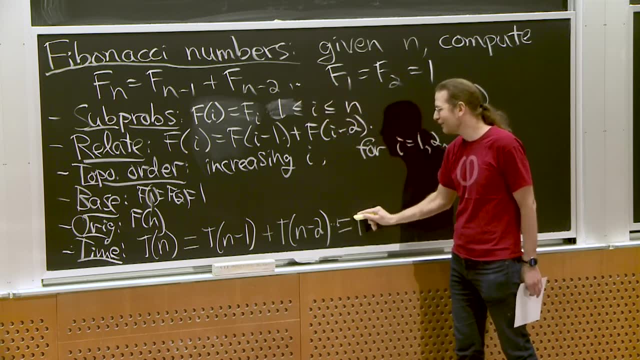 But we don't have to think about it too hard, because this recurrence is the same as this recurrence, which is the same as this recurrence. I've written it three times now, And so the solution to this is the nth Fibonacci number. Oh sorry. 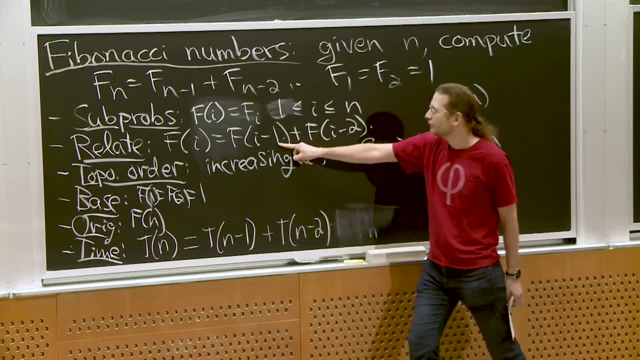 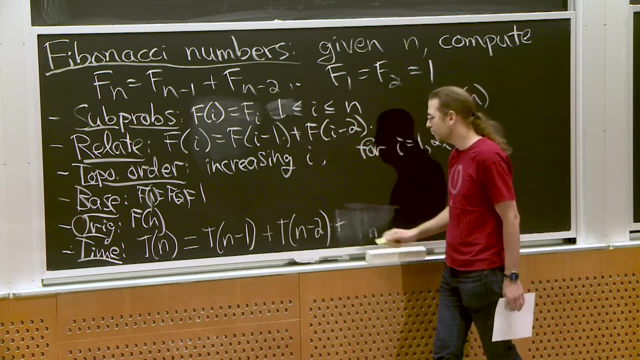 It's a little bit worse because, in addition to those recursions, I also spend constant time to do the addition. Maybe more than constant time, But if we just count the number of additions we do, it will be plus 1. Plus 1.. 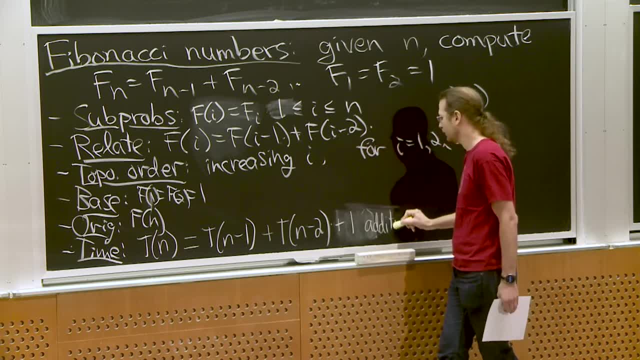 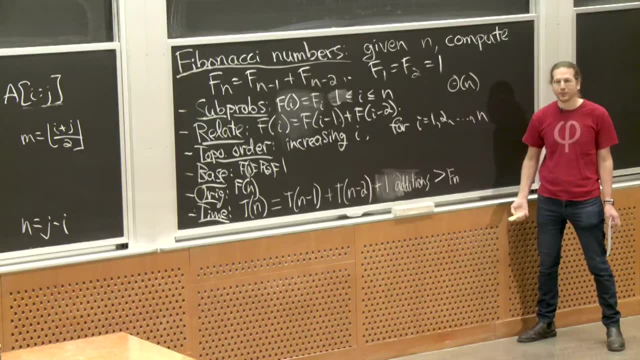 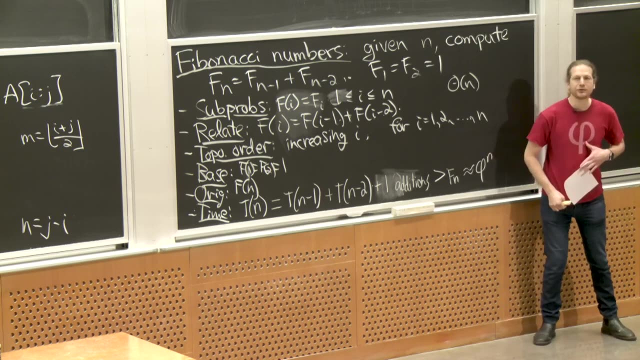 Plus 1. Additions. But this is bigger than the nth Fibonacci number And if you know anything about Fibonacci numbers, they grow exponentially. They're about golden ratio to the n. I'm wearing golden ratio in case you forgot the number. 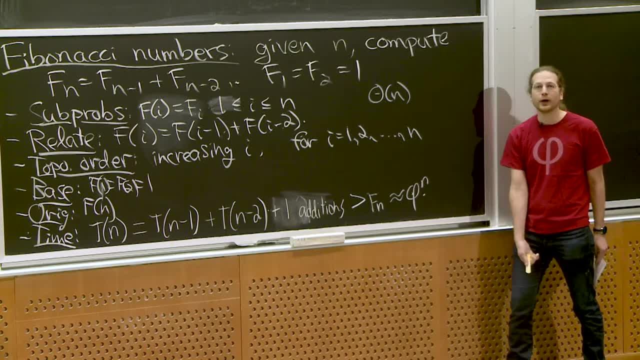 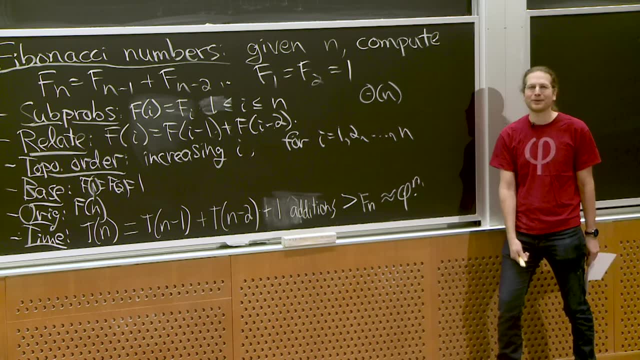 So that's bad because golden ratio is bigger than 1.. So this is exponential growth. As we know, especially in this time, exponential growth is bad And algorithms' exponential growth is bad because we can only solve very small problems with exponential growth. 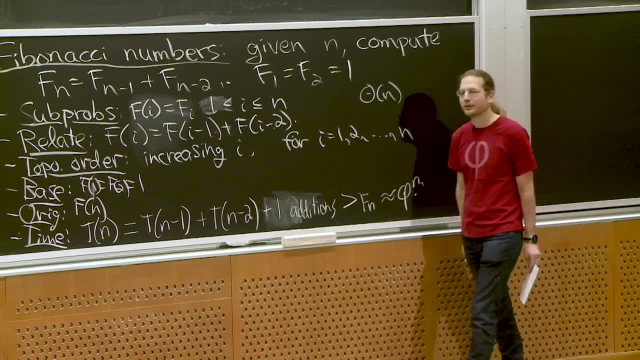 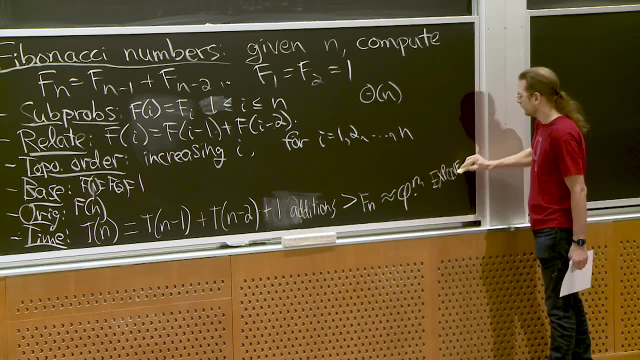 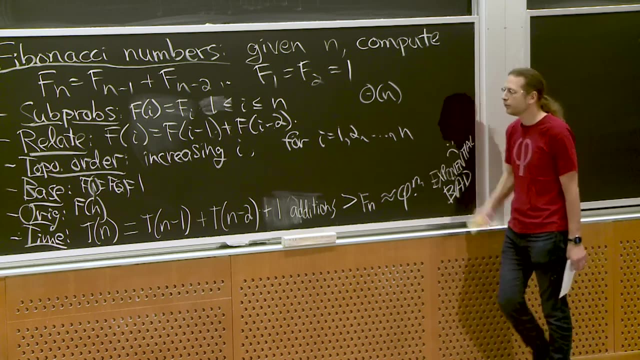 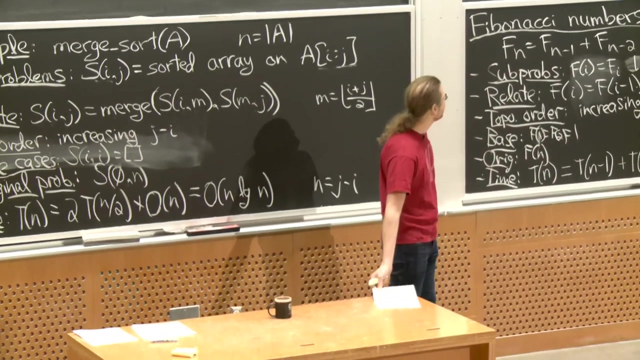 Very small n, So this is a terrible way to compute the nth Fibonacci number: Exponential, Bad OK, So don't do this. But there's a very tiny tweak to this algorithm that makes it really good, Which is memoization. 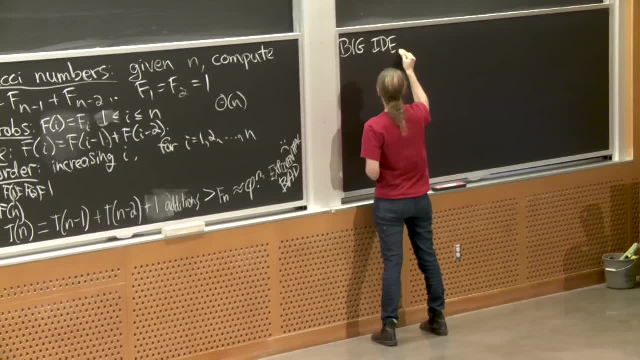 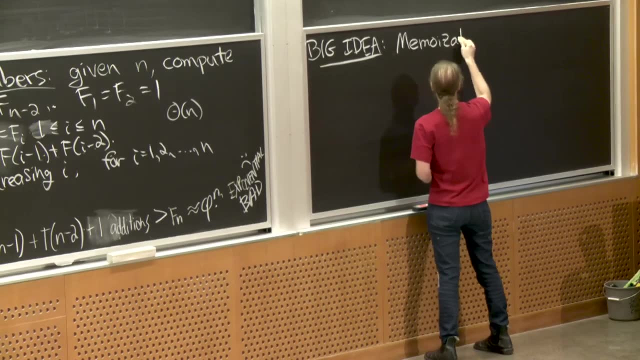 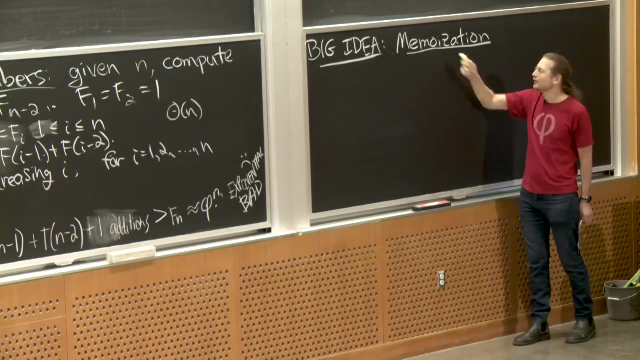 And this is a big idea. It is the big idea of dynamic programming. It's a funny word, probably made up by computer scientists. Instead of memorization, it's memoization, because we're going to write things down in a memo pad. 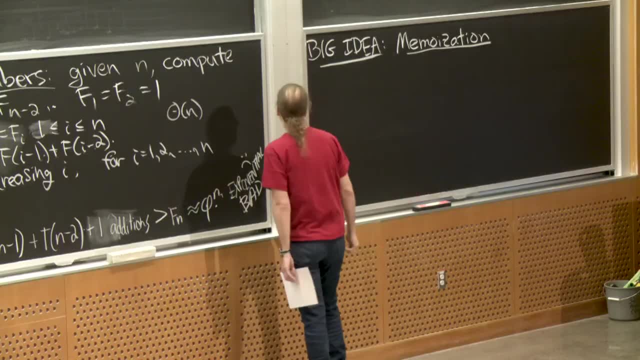 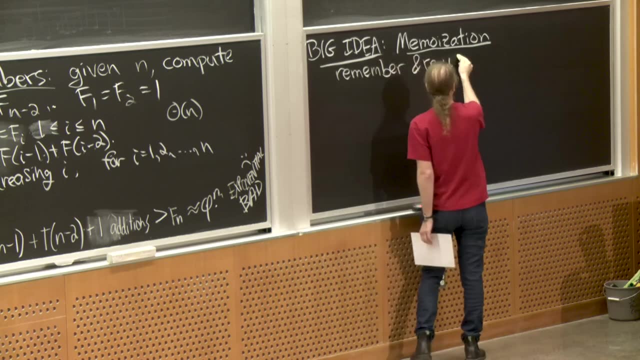 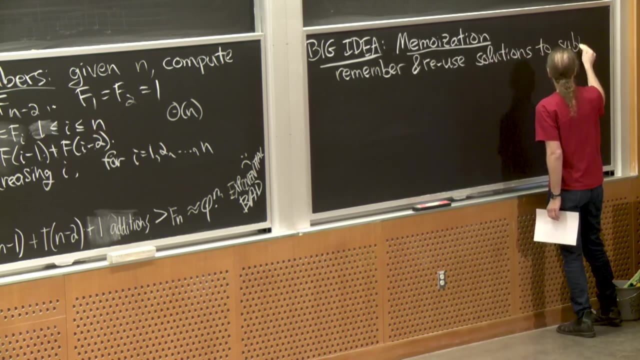 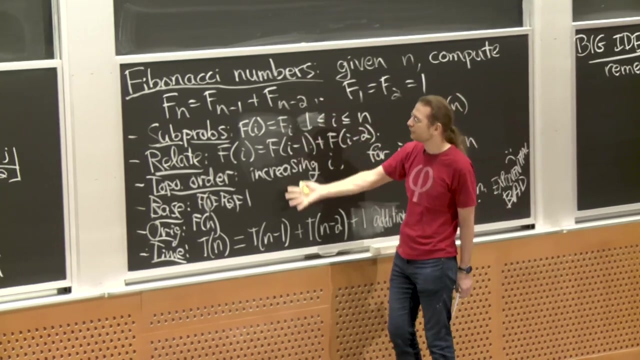 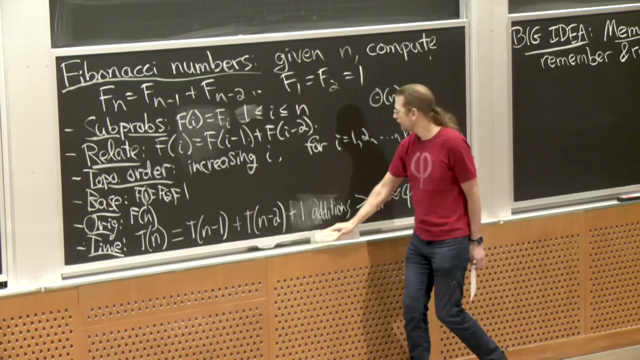 That's the idea, And it's a very simple idea, which is just remember, Remember And reuse solutions to subproblems. So let's draw the recursion tree for this recursive algorithm, as we've done it so far. So at the top, we make a little bit of space. 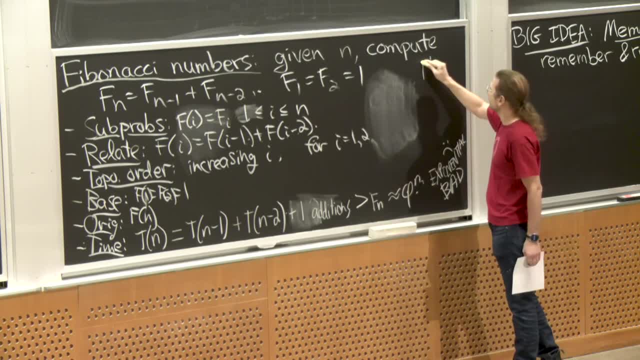 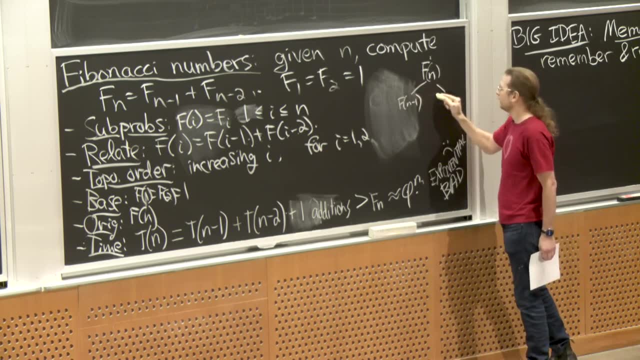 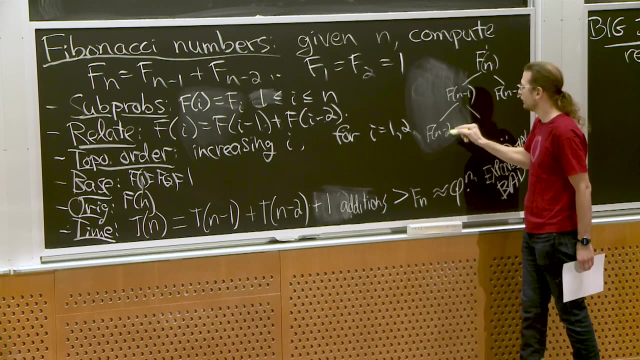 Let me make a little bit of space At the top. At the top we are calling f of n, And then that calls f of n minus 1 and f of n minus 2.. And it does an addition up here And then this calls f of n minus 2.. 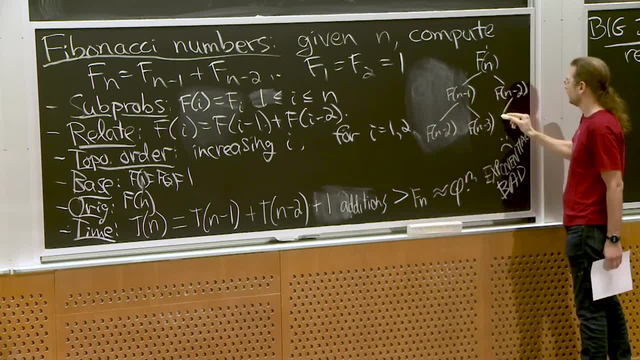 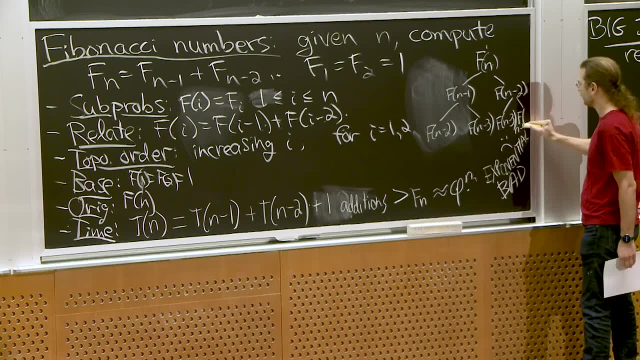 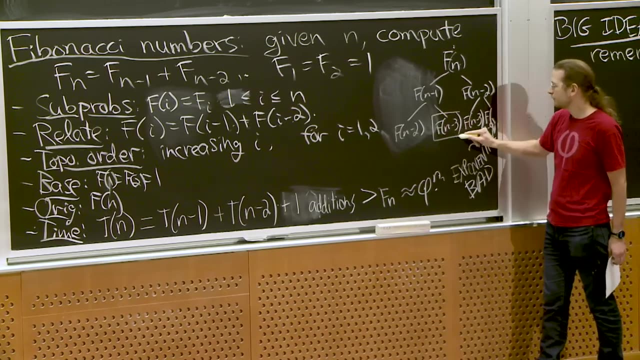 And this calls f of n minus 3.. This calls f of n minus 3.. And this calls f of n minus 4.. OK, And we notice that. We notice that this subproblem is the same as this subproblem. So to compute f of n minus 1, I need f of n minus 3.. 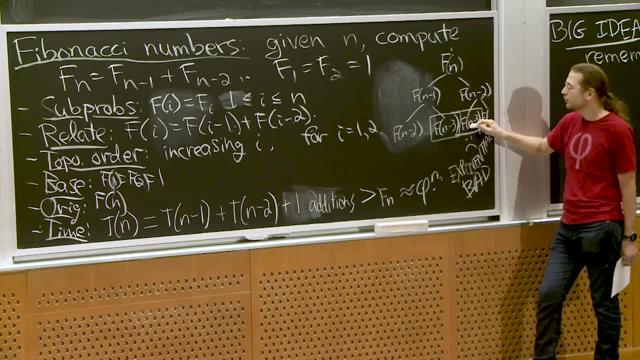 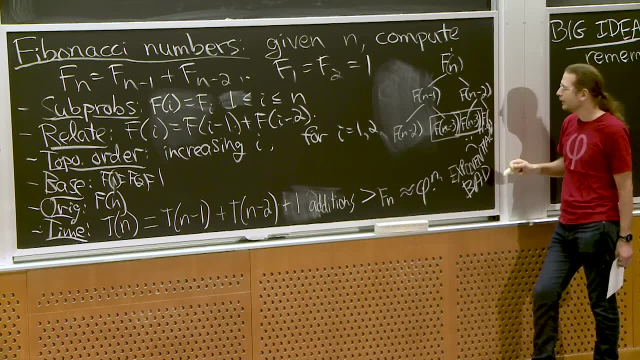 And also to compute f of n minus 2, I need f of n minus 3.. So why are we computing it twice? Let's just do it once. When we solve it, let's write it in a table somewhere, And then, when we need it again, we'll just reuse that value. 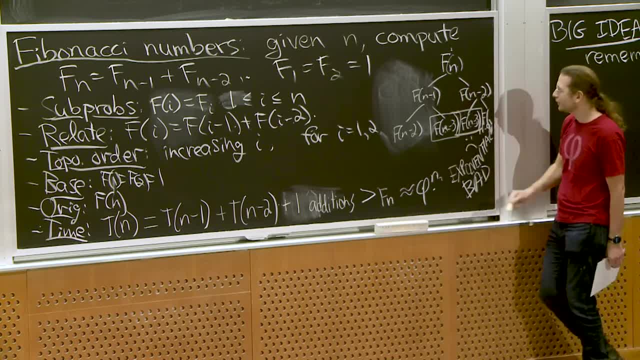 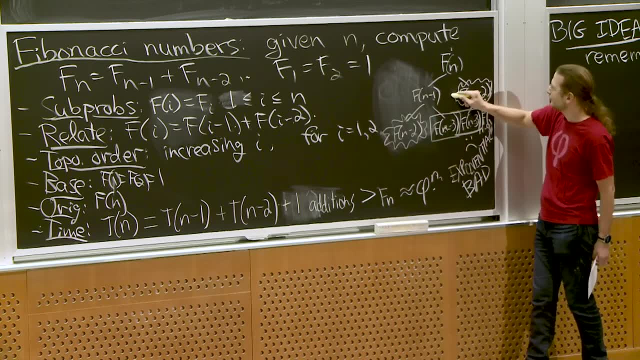 Question: What about f of n minus 2?? f of n minus 2 is also shared, So let me use a different Symbol. f of n minus 2 is already here, So this was at the same level, but we also get shared reuse between different levels. 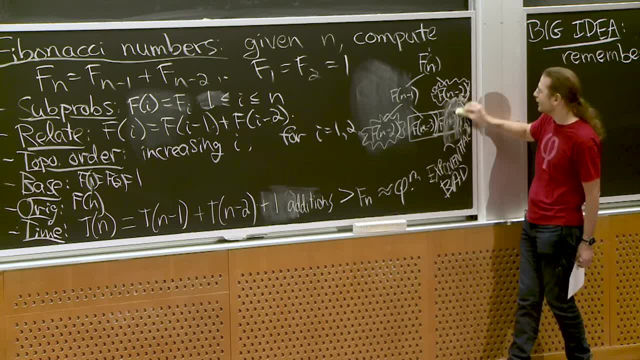 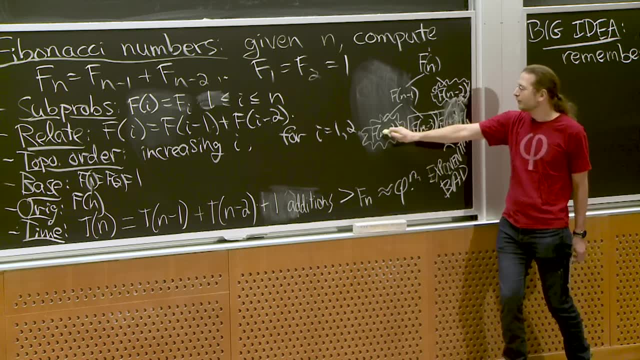 In fact I wouldn't even call f of n minus 3, because this whole part doesn't need to be computed a second time If I already computed it here. it doesn't matter which one comes first. Let's say this one comes first. 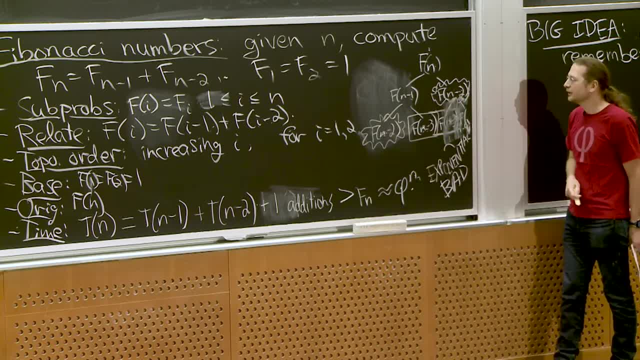 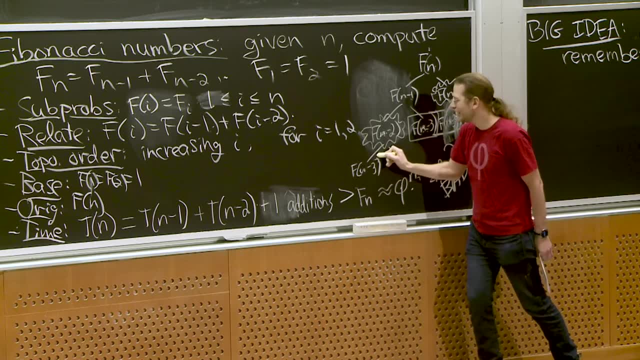 Once this is done, I can write it down and reuse it over here. OK, But actually, and then in here we're going to call f of n minus 3.. OK, So there's still another computation of f of n minus 3.. 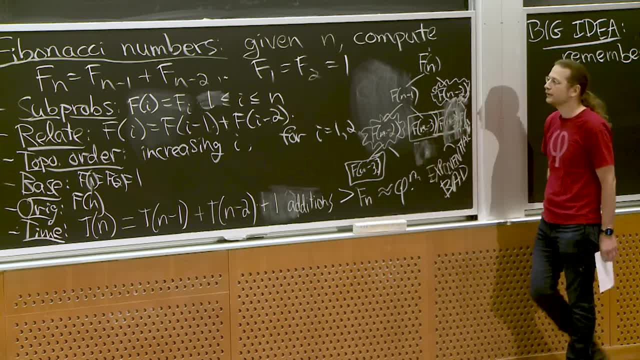 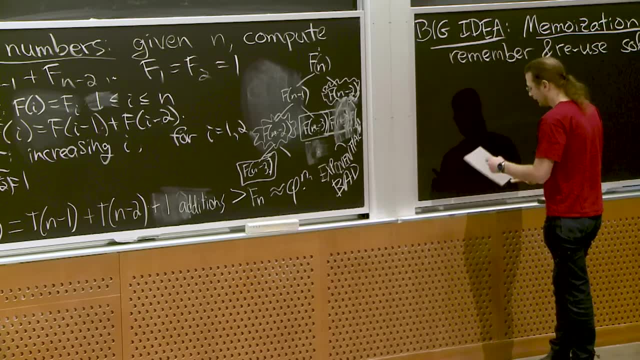 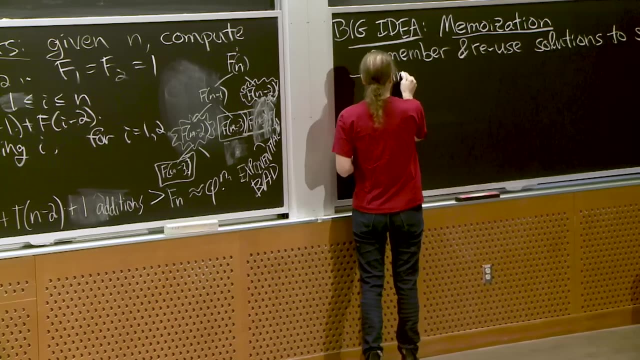 When that one's done, I won't need to do this recursively. OK, So magically, this is going to make this algorithm efficient with this very simple tweak. Let me write down the tweak more explicitly. I won't write code here, but just describe it. 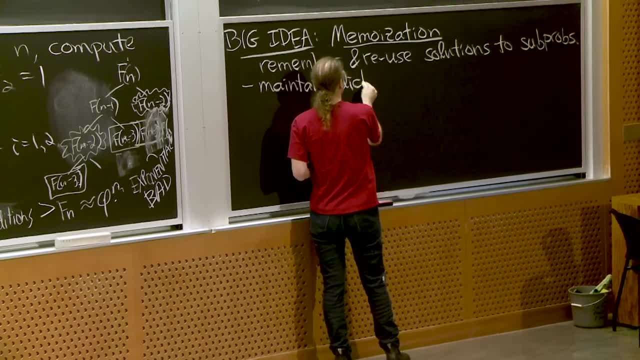 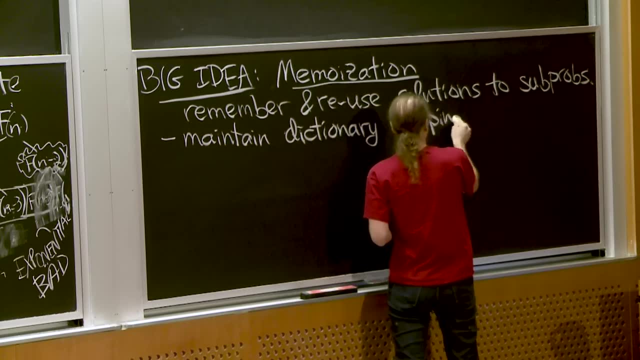 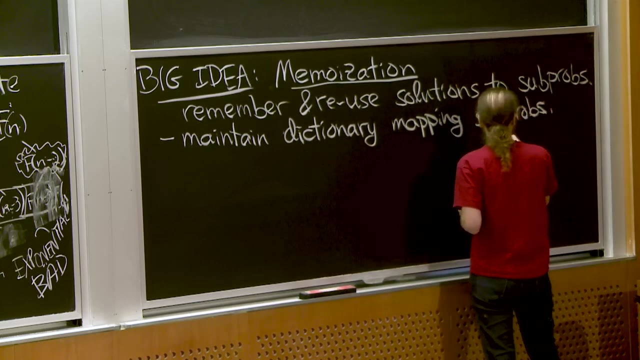 as a data structure. So we're going to maintain our good friend, the dictionary, Which is abstract data type or interface. We could use different data structures to do it, But we're going to map subproblems to their solutions, at least the ones that we've solved already. 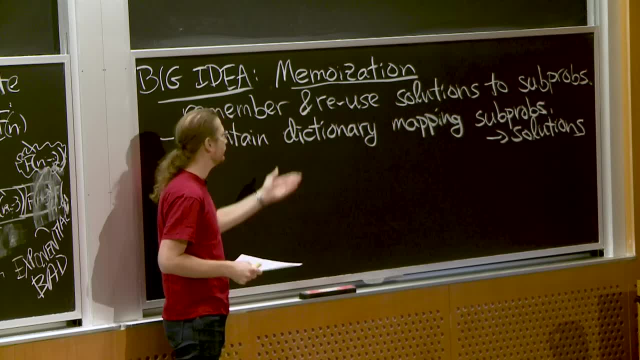 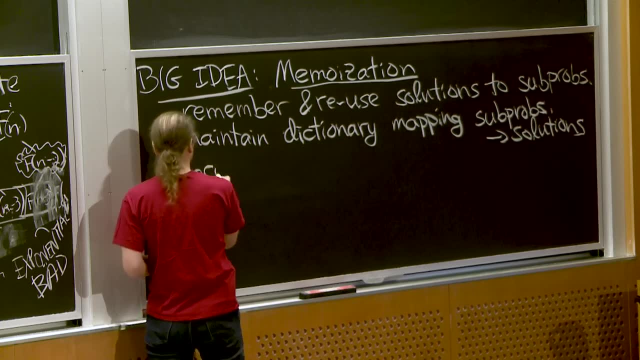 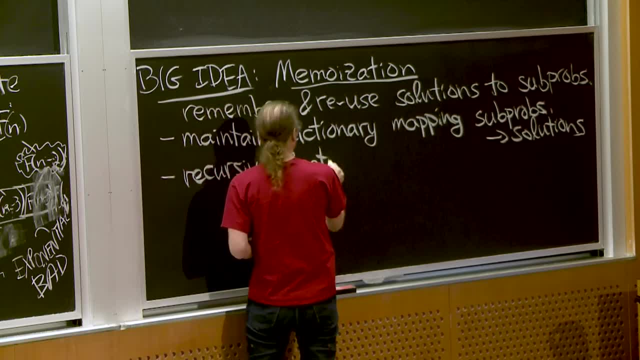 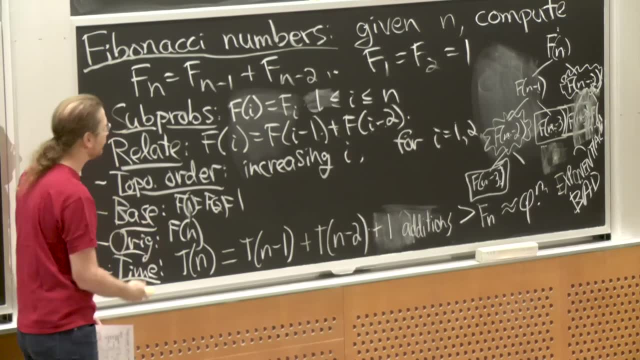 OK, OK, OK, OK, When we write the code for our recursive function. So in general, once we have a sort bot description, we can turn this into code. We define f of i And it says: am I in a base case? 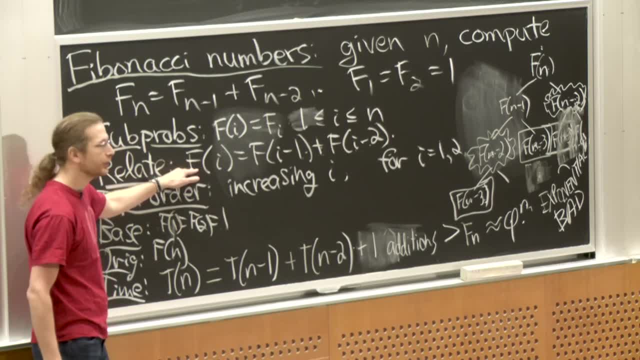 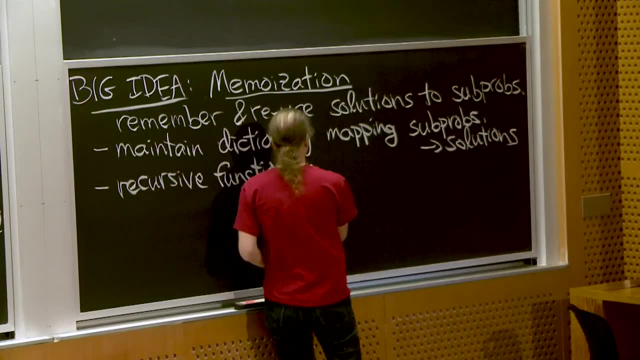 If so, return this. Otherwise, do this recursive call. That's our recursive algorithm, But we're going to do a little more now, And first we're going to check whether this subproblem that we're trying to solve has already been solved. 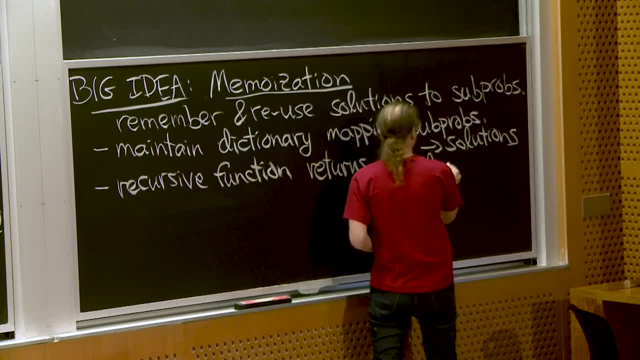 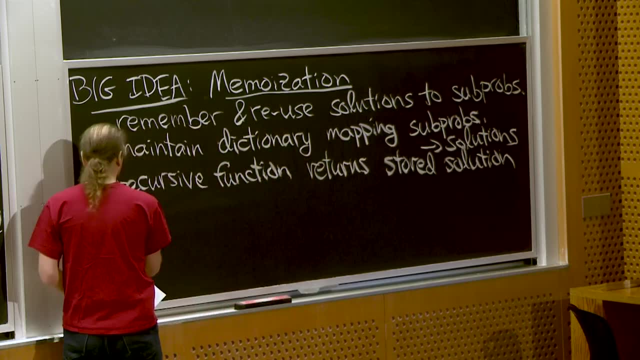 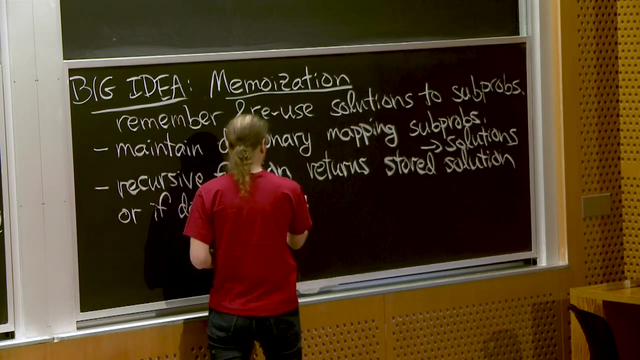 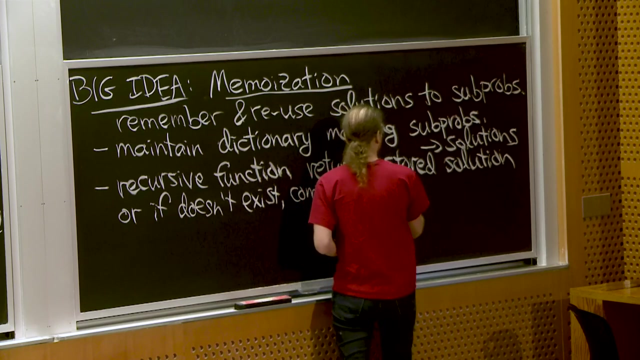 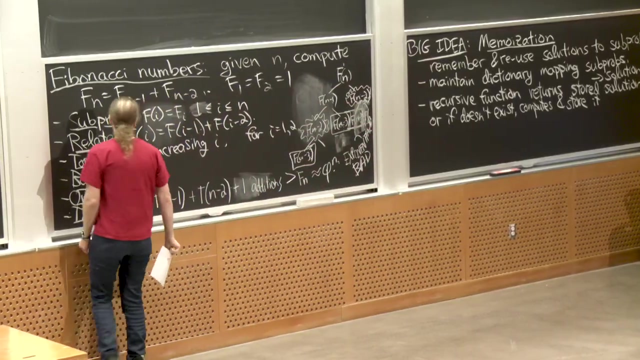 And if so we return that stored solution. That's the easy case, But it might not exist, And then we'll compute it in the usual way. So what the code then would look like to define. to define f of i is: first we check. 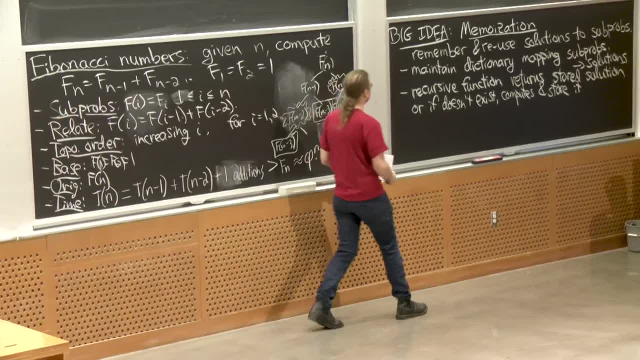 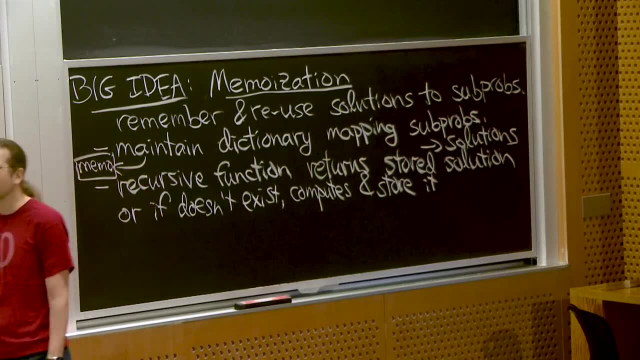 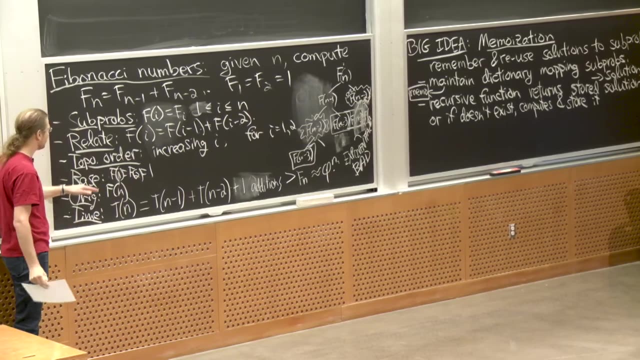 is i in our data structure. This is usually called the memo. So we say: is this subproblem? is i in my memo data structure? If so, just return memo of i Done. No recursion necessary, Otherwise check if I'm a base case. 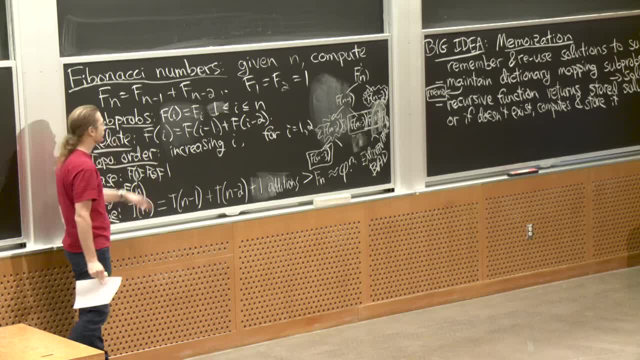 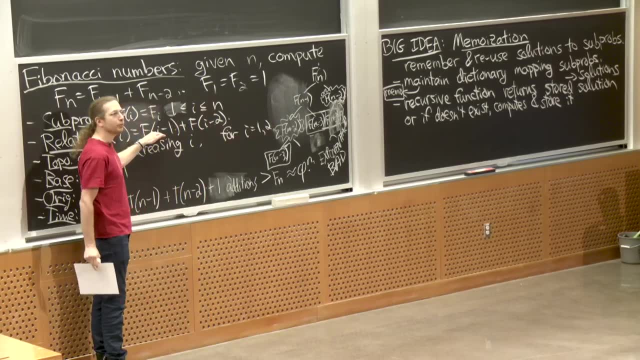 If so done, Otherwise recurse. So recursively call f of i minus 1 and f of i minus 2.. And in this recursion we can see, OK, We can see- that after we call f of i minus 1, in fact, 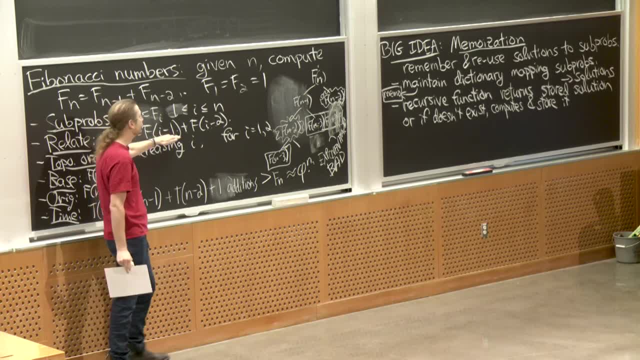 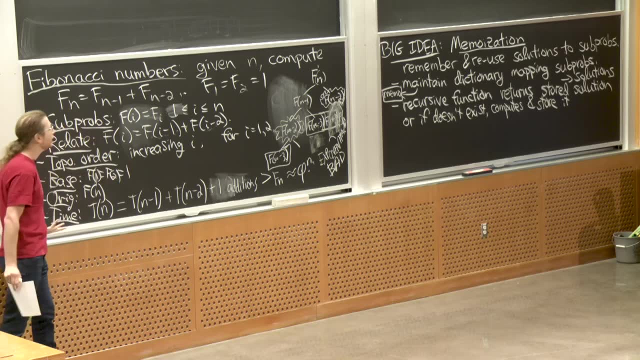 it will have already computed f of i minus 2.. So while this call is recursive, this one will immediately terminate, because i minus 2 will already be in the memo table, And so, if you think about what happens, in fact, we'll just have recursion down the left branch of this thing. 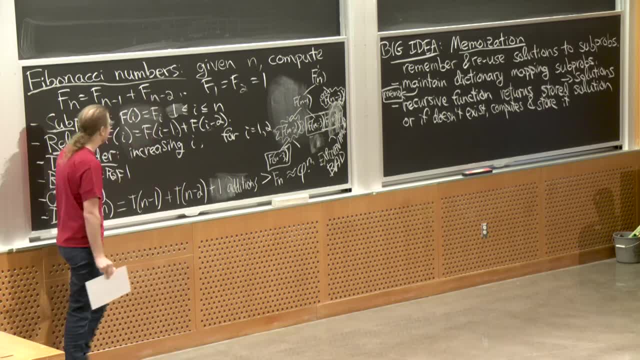 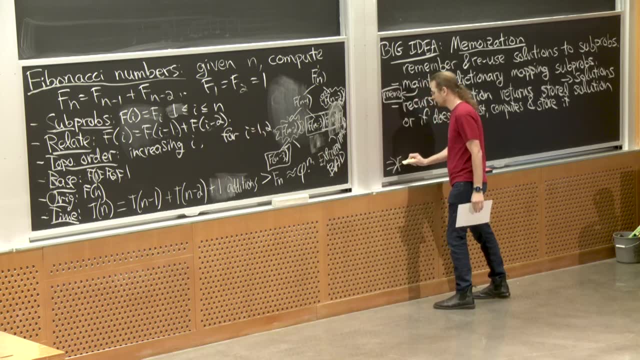 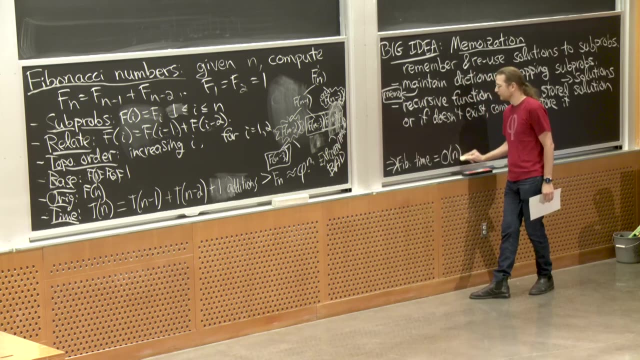 And all the right branches will be free. We can just look things up in the memo table. So what is the overall running time For Fibonacci? This should be order n. Why is it order n? This is number of additions. Come back to that in a second. 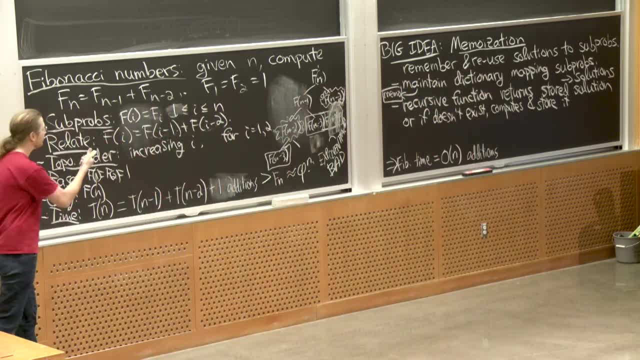 In general, the way to analyze an algorithm like this that uses memorization is we just count how many different subproblems are there, Because once we solve the subproblem, we will never solve it again. That's the whole idea of a memo table. 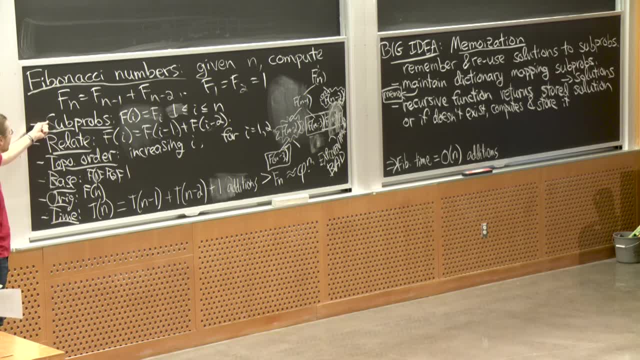 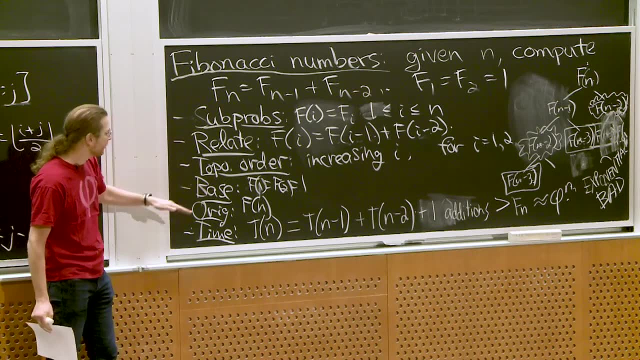 So we will solve each subproblem at most once, And so we just need to count how much time does it take to solve every subproblem? And here you can see it's constant. Either it's a base case and it takes constant time. 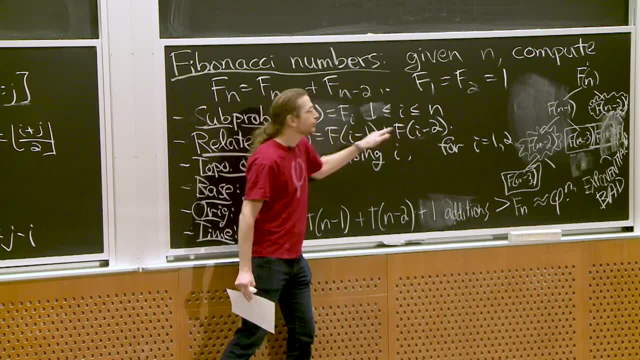 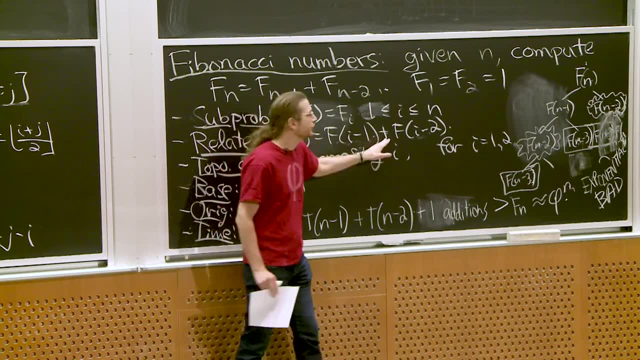 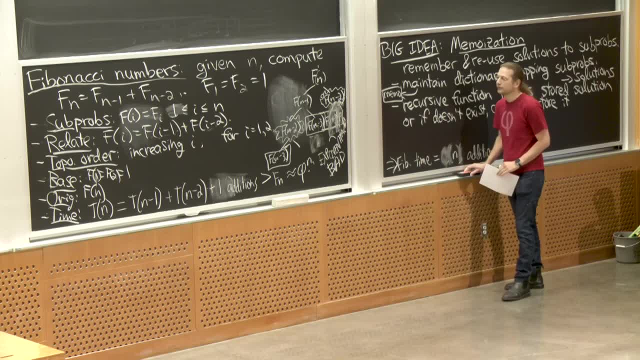 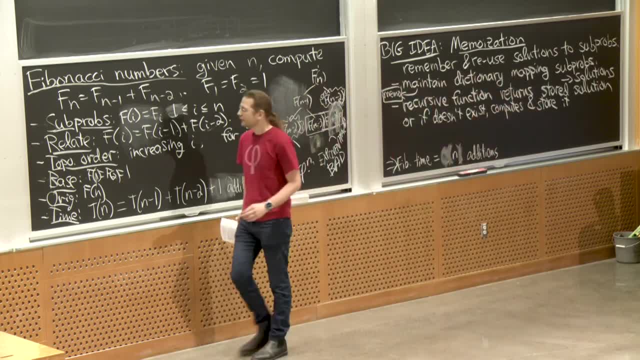 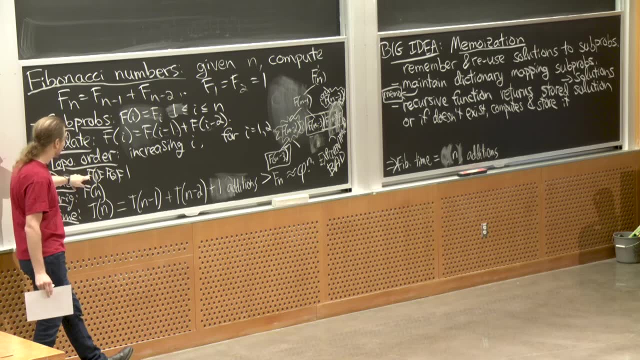 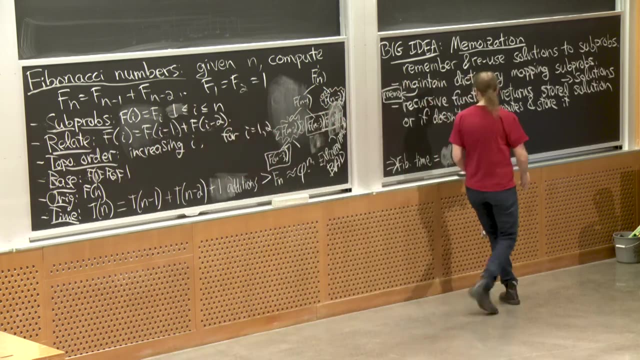 So it turns out to be a very nice closed form. in this case It should be exactly n subproblems to compute F of n, because we start at 1. And each one has one addition involved. I guess not the base case, so maybe n minus 2.. 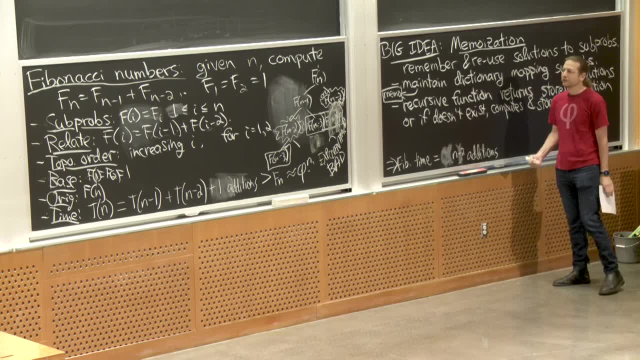 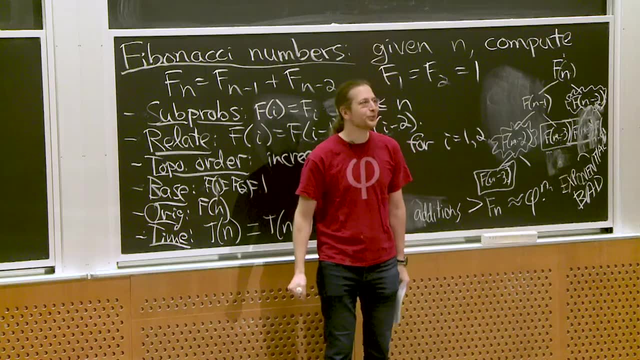 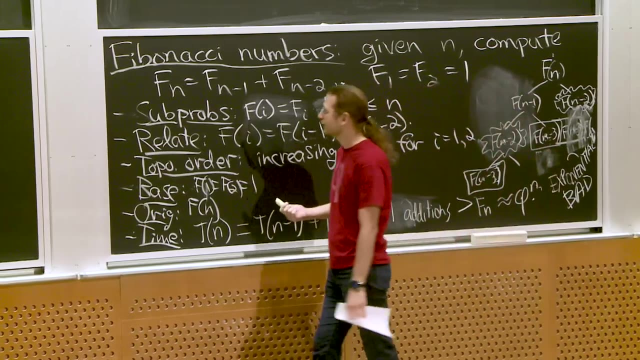 Definitely order n. Now there's this one subtlety, which. let's forget about dynamic programming for a moment and go back to good old lecture 1 and 2, talking about the word RAM, model of computation, A question here that usually doesn't matter in this class. 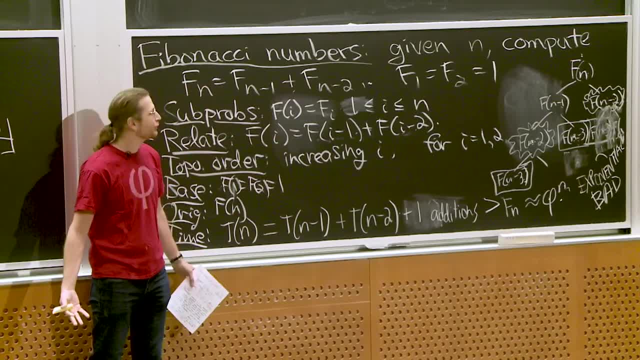 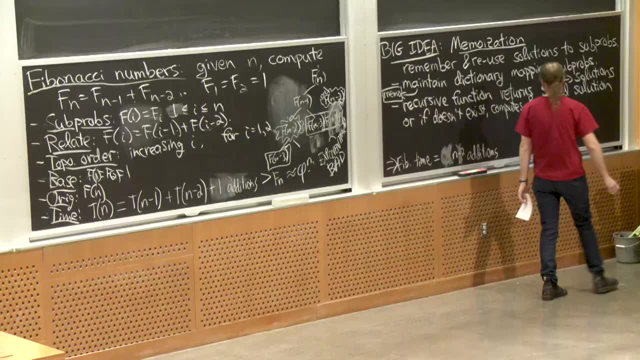 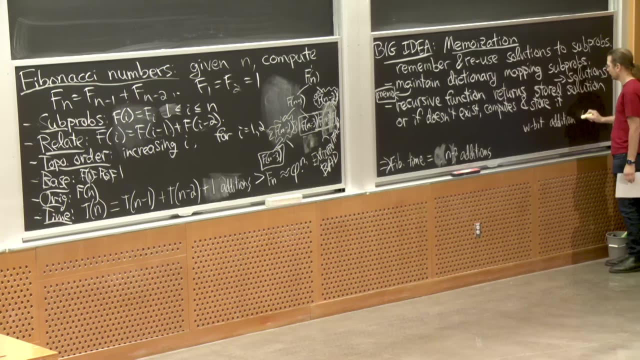 Usually we assume additions take constant time, And we usually do that because it's usually true And in general our model is that w bit additions, where w is our machine word size, takes constant time. But for this problem, and this problem only pretty much. 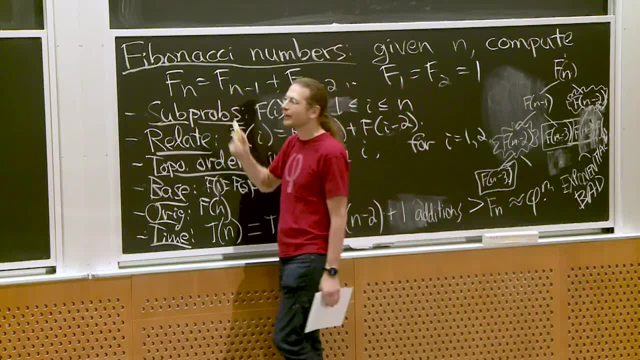 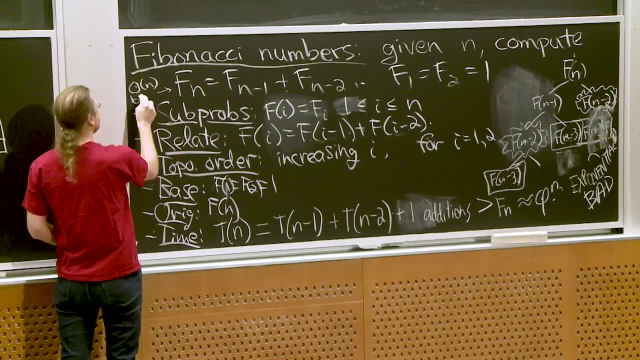 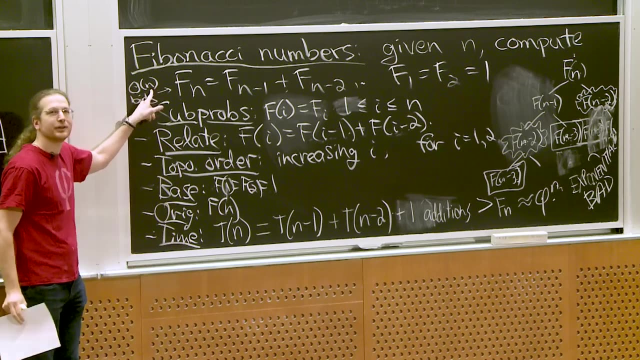 for Fibonacci numbers. I happen to know that the Fibonacci numbers grow exponentially, So to write them down actually requires theta n bits, because they are some constant to the n power And so they're actually really big. n is probably bigger than w. Usually you think of problems that. 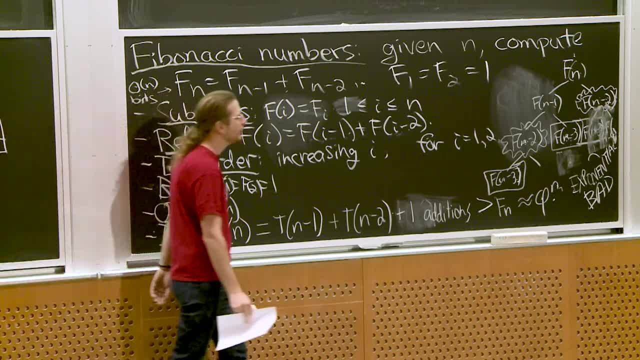 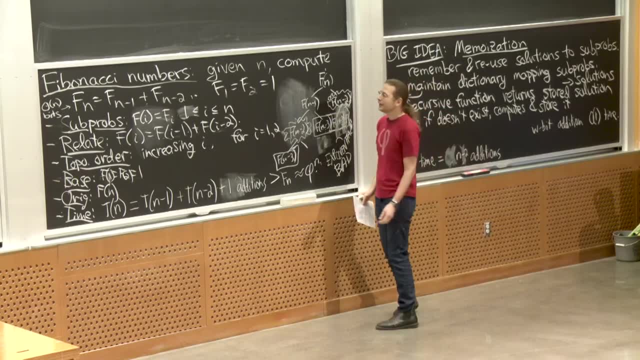 are much bigger than 64 or whatever your word size happens to be. We do assume that w is at least log n, But n is probably bigger than w. It might be bigger or smaller, We don't know. And in general, to do an n bit addition, 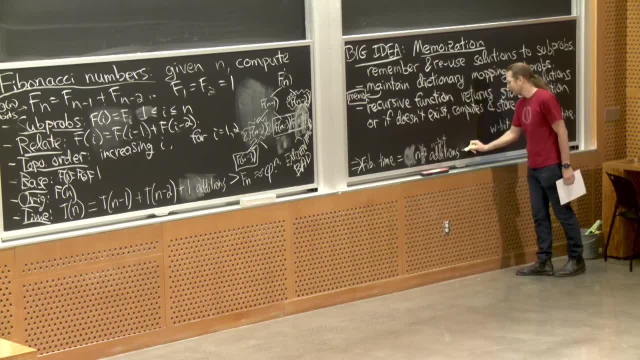 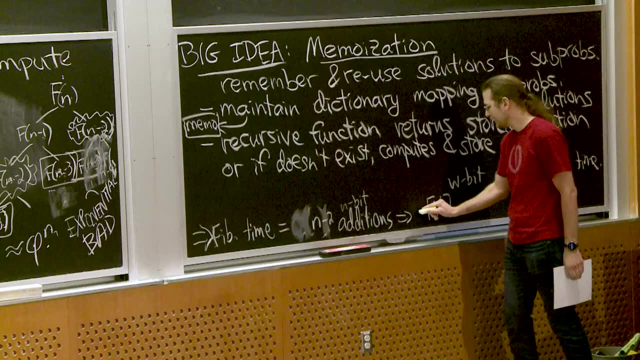 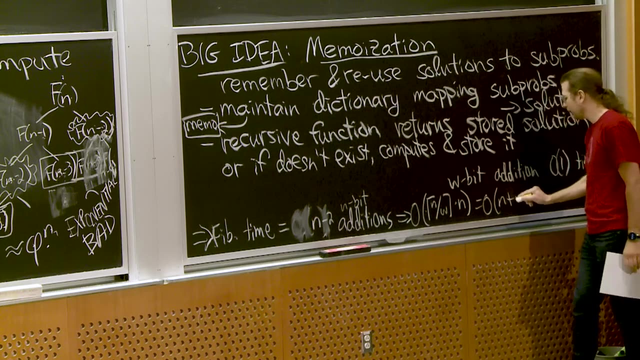 these are n bit additions is going to take a ceiling of n over w time, So in the end we will spend this times n because we have to do that many of them, which is n plus n squared over w Time. 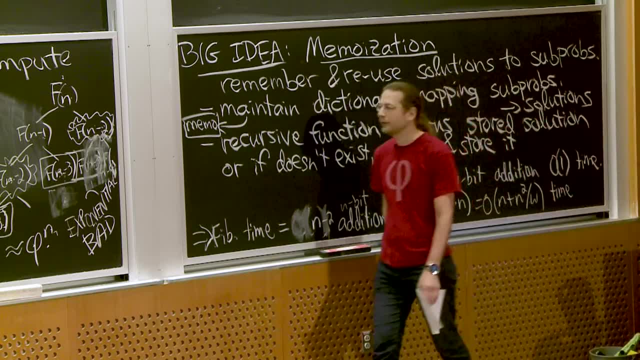 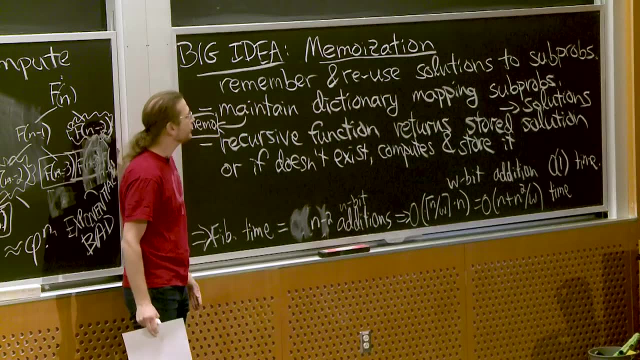 So a bit of a weird running time, but it's polynomial. Whereas this original recursive algorithm was exponential- here, using this one simple idea of just remembering the work we've done- suddenly this exponential time algorithm becomes polynomial. Why? Because we have few subproblems. 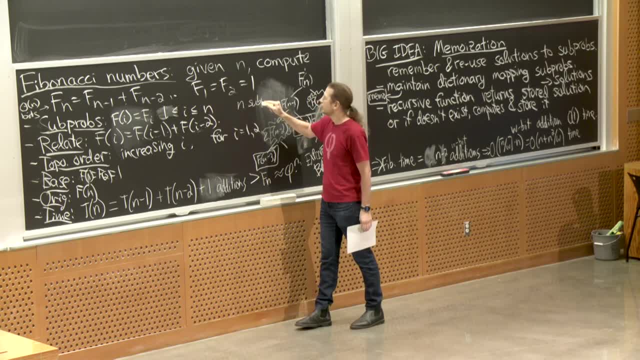 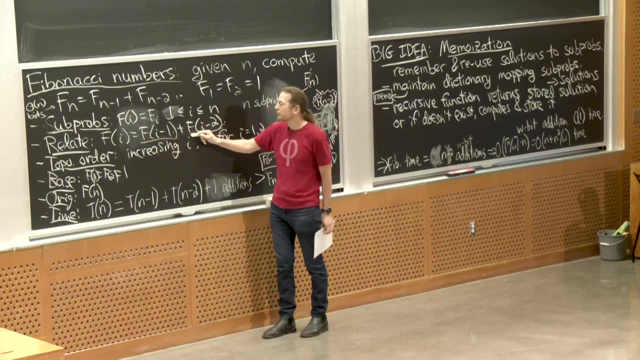 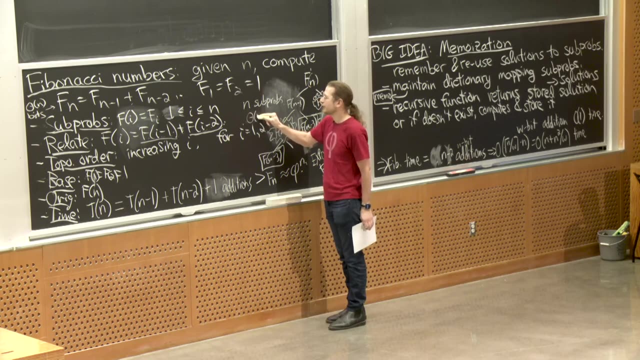 We had n subproblems And for each subproblem we could write a recurrence relation that if we already knew the solutions to smaller subproblems we could compute this bigger problem very efficiently. This happened to be constant time or constant additions, n over w time. 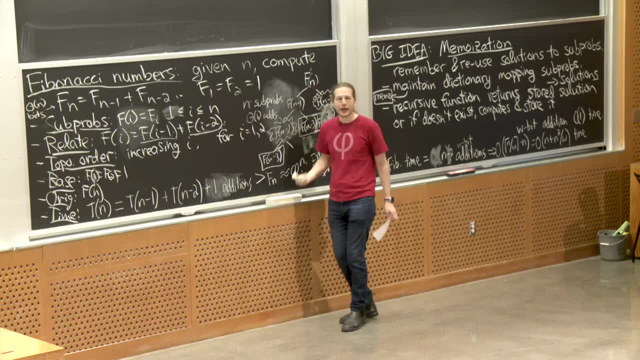 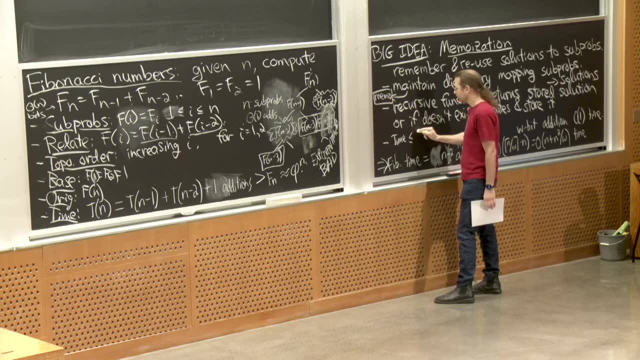 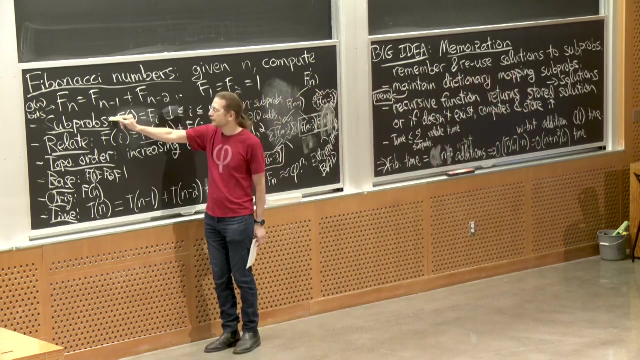 But as long as this is polynomial, and this is polynomial, we're happy Because we have this nice formula that the time it takes is at most the sum over all subproblems of the relation time. OK, So I'm referring to subproblems, the number of them. 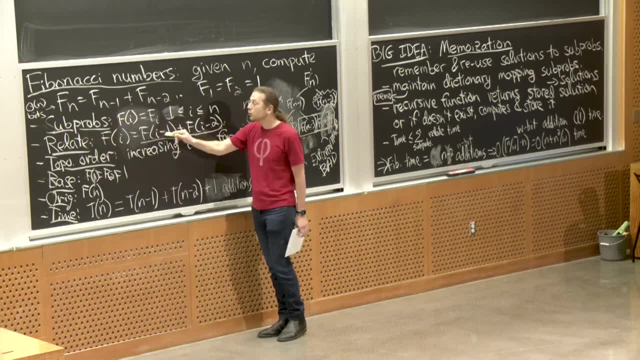 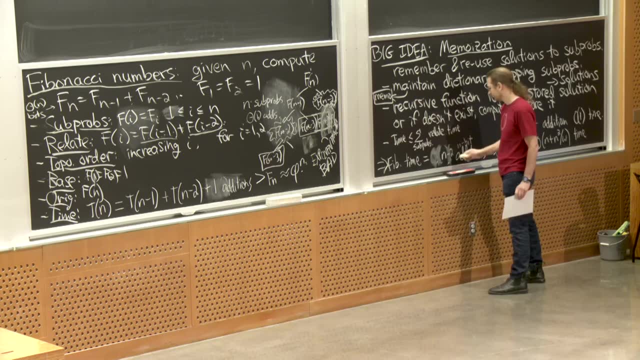 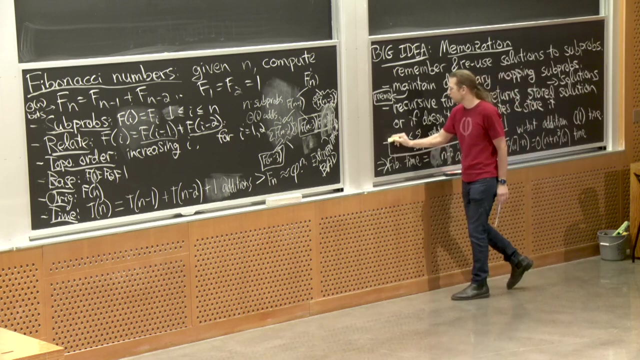 and the time it takes to evaluate this, ignoring the recursive calls. That's important. This is the non-recursive part In the notes. I call this non-recursive work, So this formula gives us a way to bound the running time of one of these algorithms. 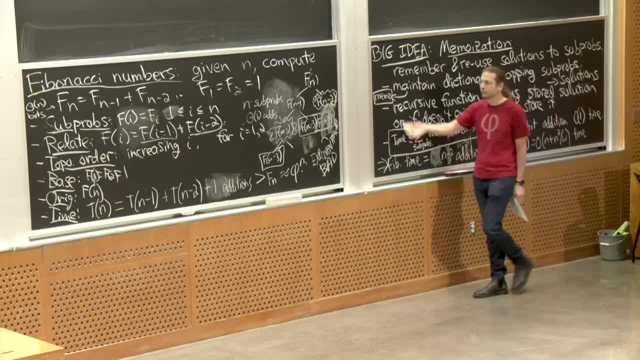 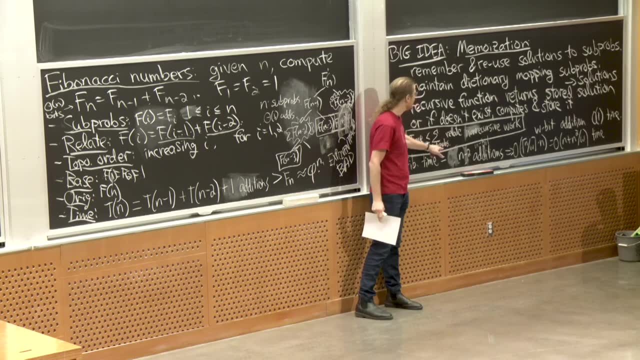 if we use memoization. Without memoization, this is not true. Fibonacci took exponential time. But if we add memoization, we know that we only solve each subproblem once, And so we just need to see for each one: how much did it cost me to compute it? 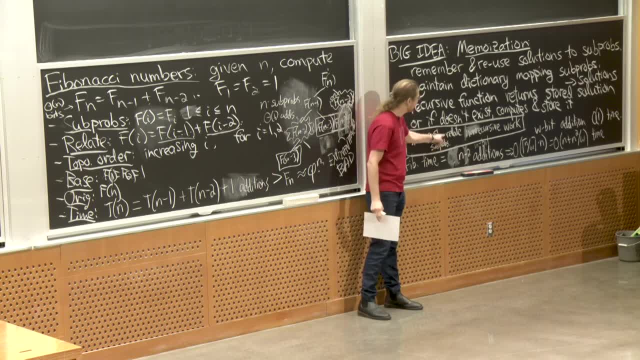 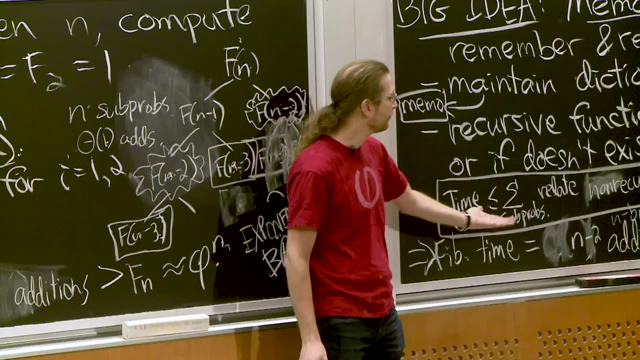 assuming all the recursion work is free, because that's already taken into account by the summation. OK, So in particular, this summation is at most the number of subproblems times the time per subproblem, which in this case is order n. 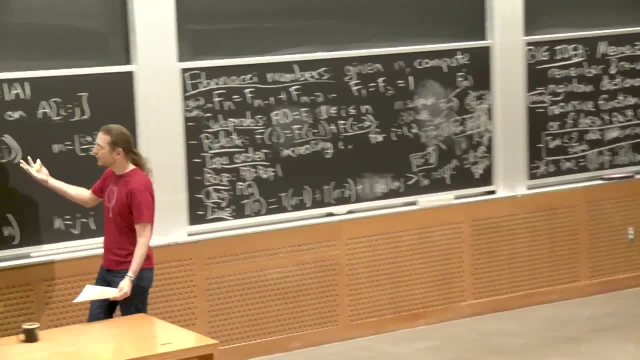 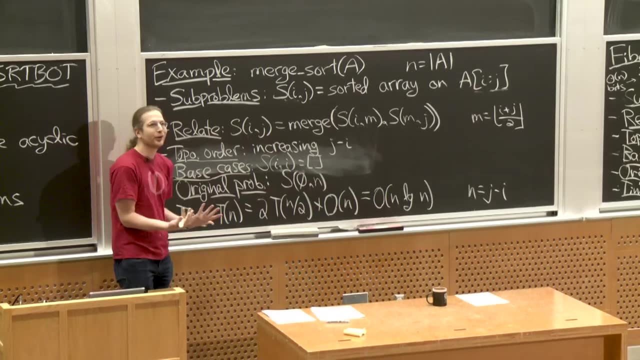 We could try to apply that analysis to merge sort, because after all this is also a recursive algorithm. It happens to not benefit from memoization, But we could throw in memoization, It wouldn't hurt us. But if you think about the call graph here, 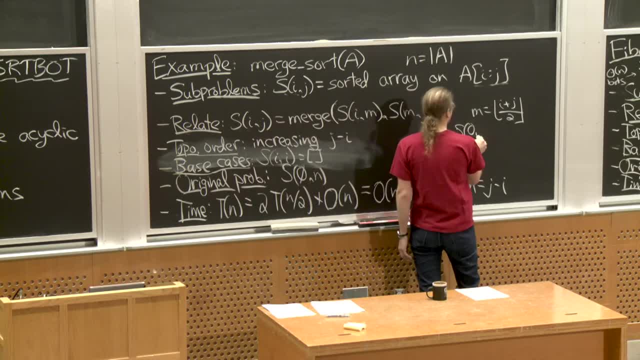 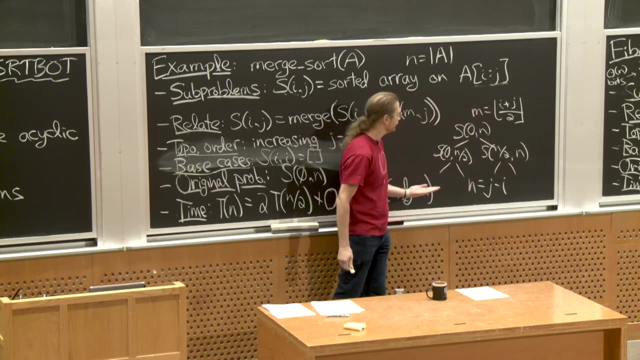 which is like s of 0- n, which calls s of 0 n over 2, and s of n over 2 n, and so on. it has the same picture, But there's actually no common substructure here. You'll never see a repeated subproblem. 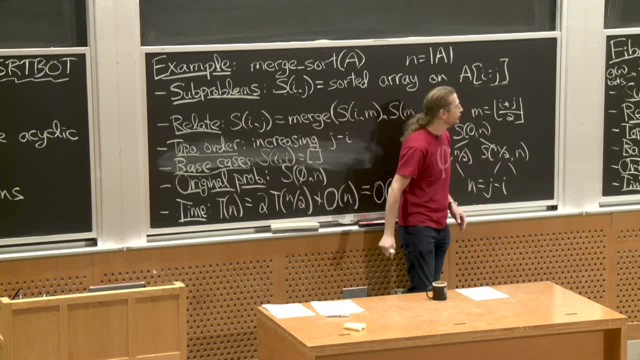 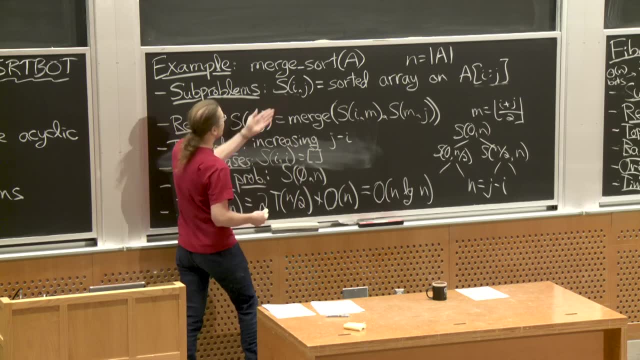 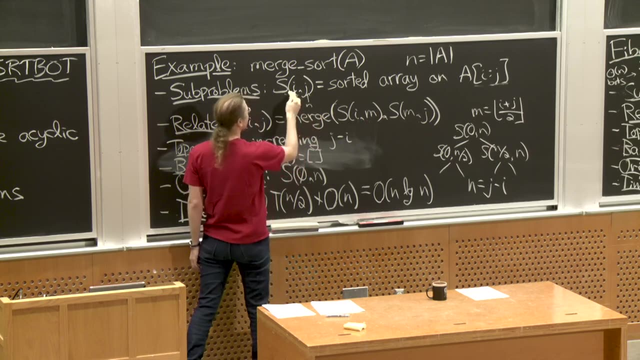 because this range is completely disjoint from this range. But you could throw in memoization and try to analyze in the same way and say: well, how many subproblems are there? Well, it looks like there's n choices for i and not quite n choices, but in general it's at most. 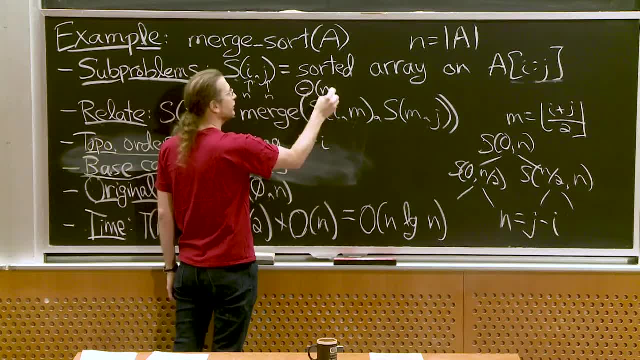 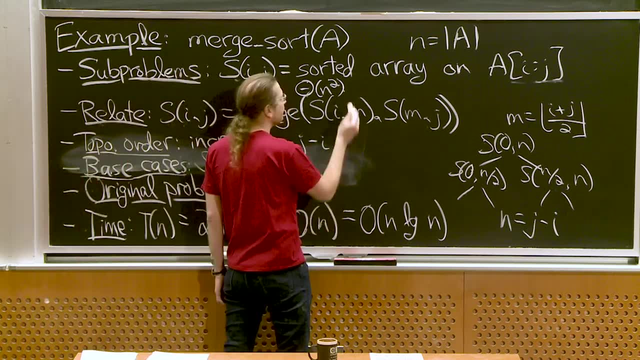 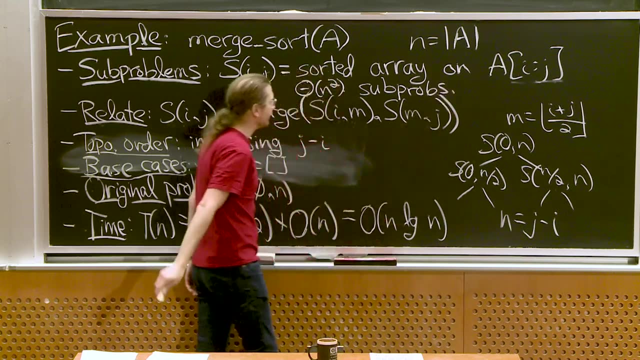 n squared, different choices. In fact it's the triangular number: sum of i equals 1 to n of i, different possible choices for i and j. But this is theta n squared subproblems, which seems not so good. And then, how much time are we spending per subproblem? 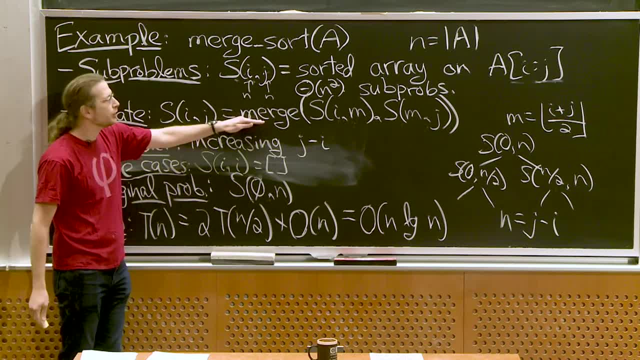 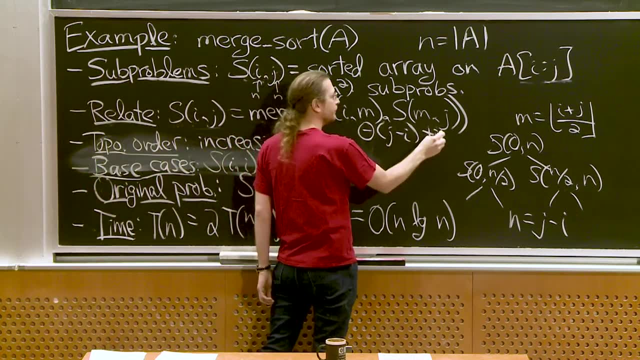 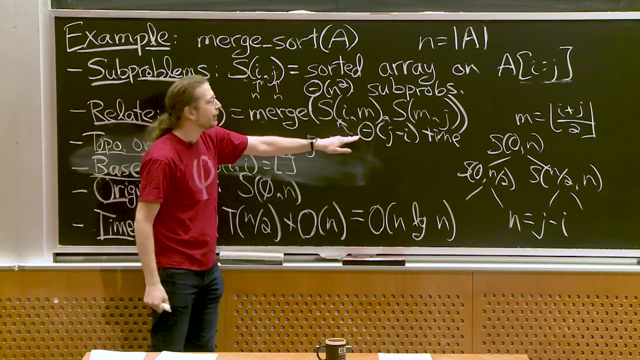 Well, to solve s of ij we have to merge about that many elements. We know merge takes linear time, And so this takes theta j minus i- time to evaluate, And so what we'd like to do is sum over all the subproblems of j minus i. 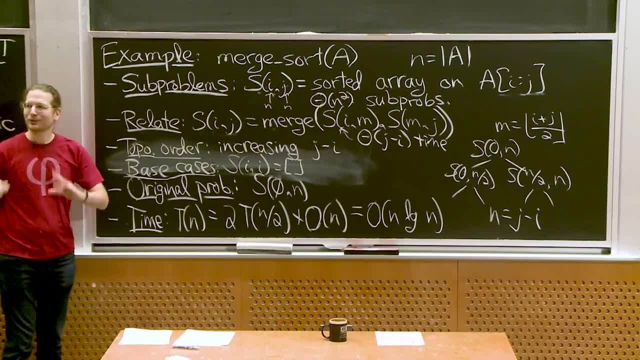 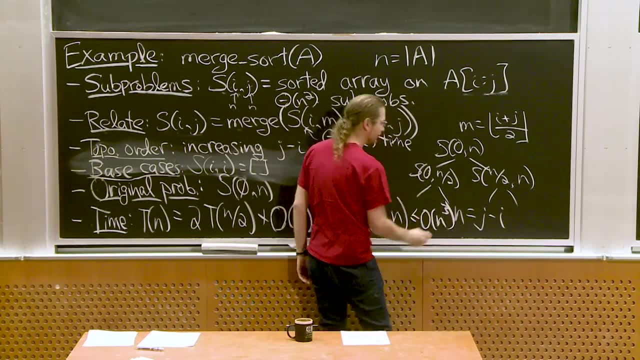 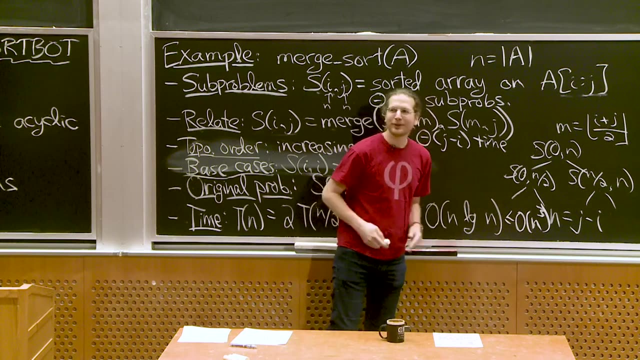 This is the not triangular number, but the tetrahedral number, I guess, And so we end up that the running time is at most n cubed. Great, So it's true that n log n is less than or equal to n cubed. 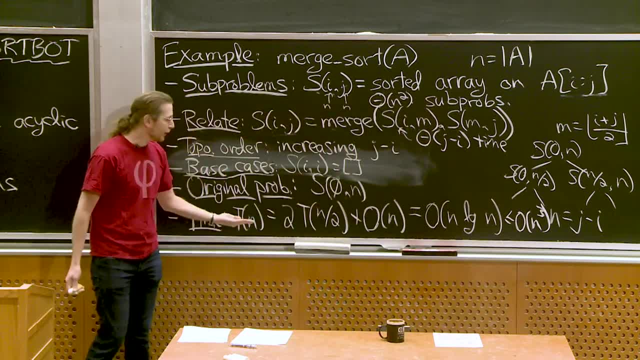 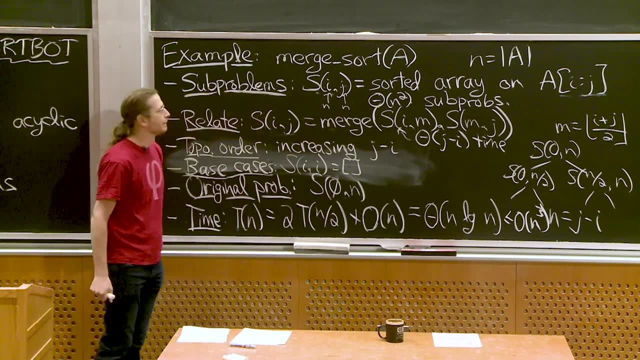 but obviously not terribly useful. This algorithm, by the way, we are already know how to analyze. it is indeed n log n, And the running time turns out to be theta n log n. So sometimes this equation is not what you want to use. 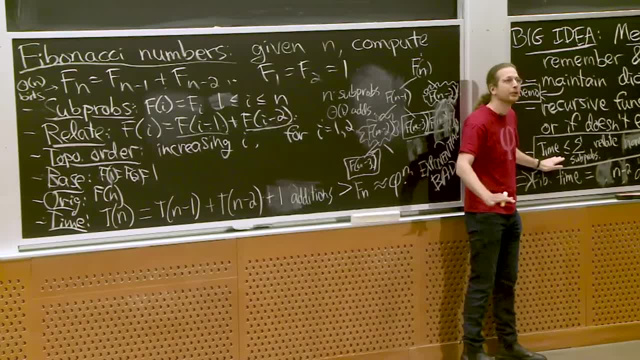 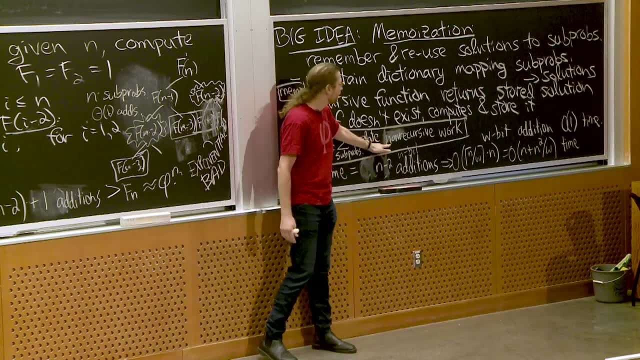 But often it's good enough And especially if you just want to get a polynomial upper bound, then you can try to optimize it later. This will give you a polynomial upper bound as long as the number of subproblems is polynomial and the time per subproblem is polynomial. 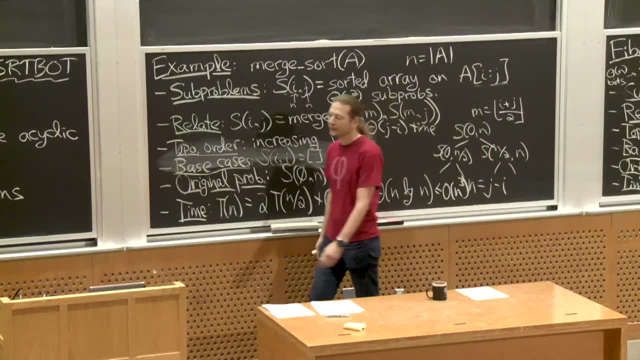 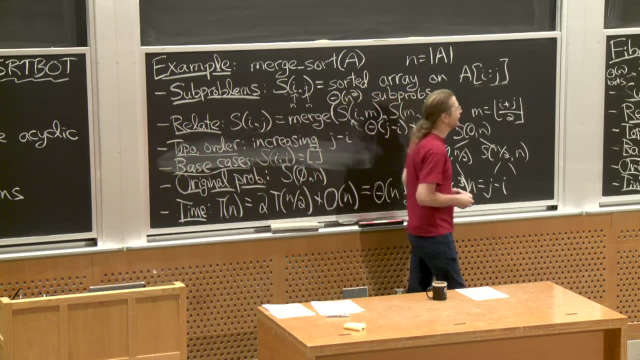 And indeed n cubed is polynomial. It's not a great polynomial, but this is an alternate way to analyze merge sort. Obviously don't do this for merge sort, but it illustrates the technique. Good so far. Any questions? All right. 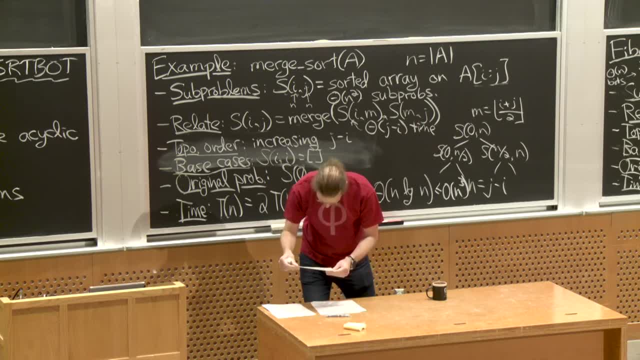 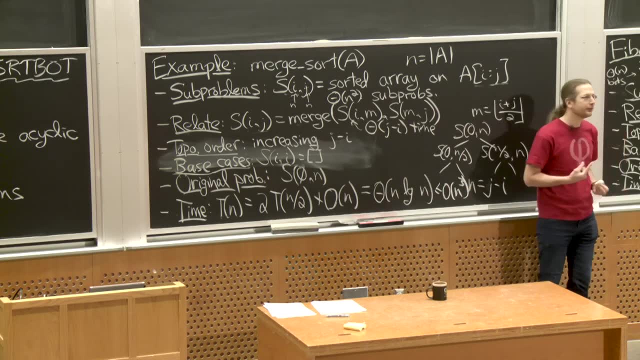 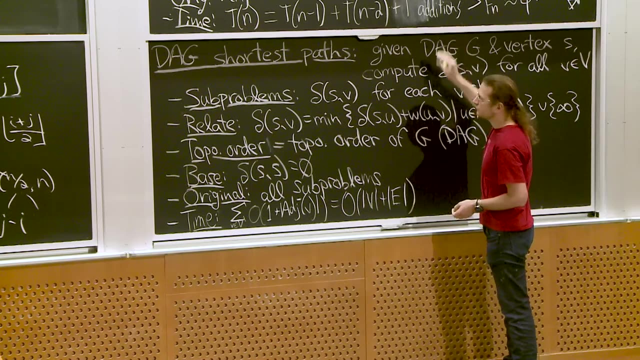 Let me remember where we are Cool. So the next thing I'd like to do is show you one more algorithm that we've already seen in this class that fits very nicely into this structure, arguably, is a dynamic program, And that is DAG: shortest paths. 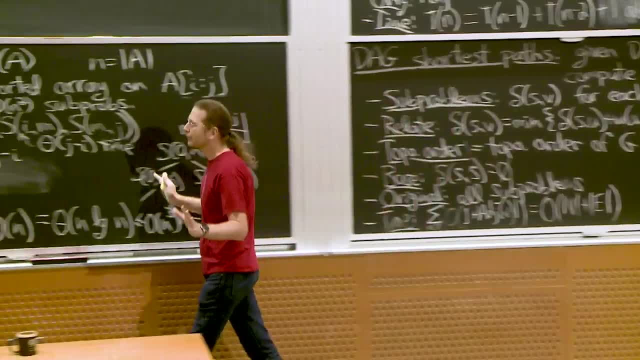 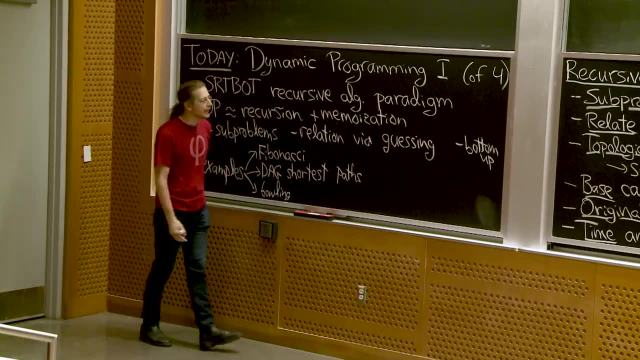 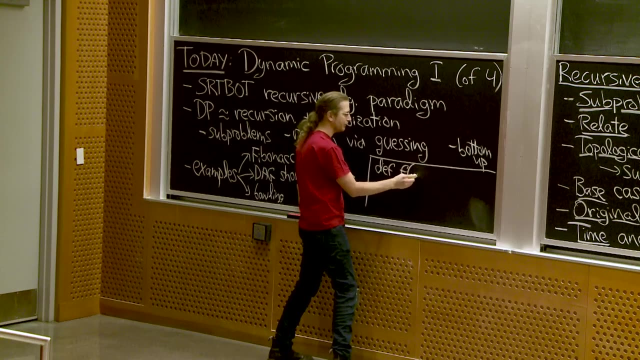 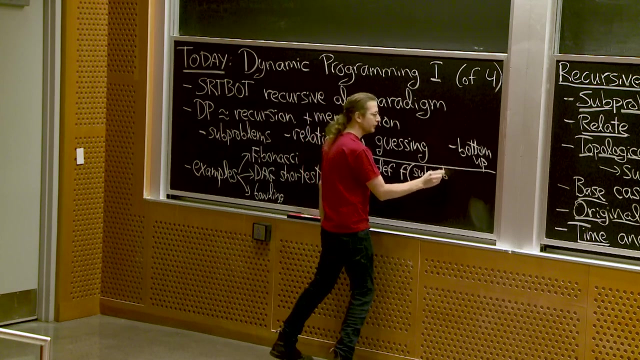 Oh, so just to close the loop here: when I say dynamic programming I mean recursion. with memoization I mean we write a recursive piece of code which is like def f of some args, some subproblem specification We check Is. 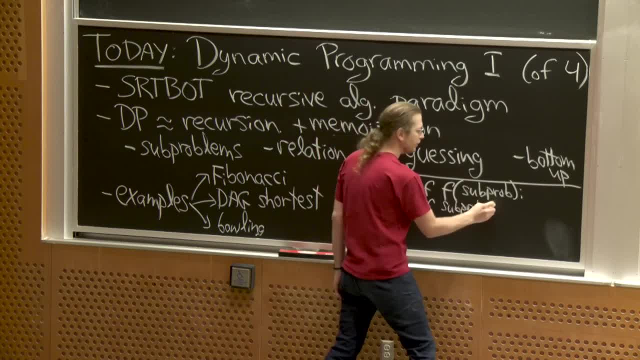 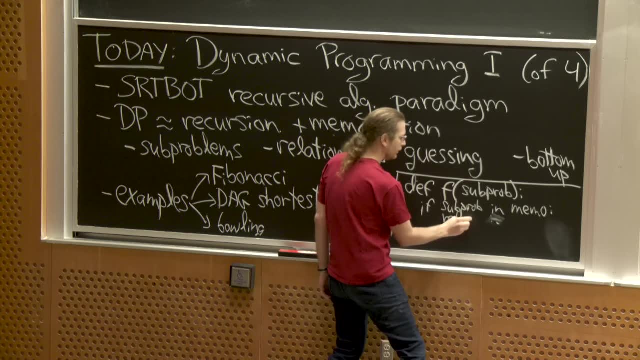 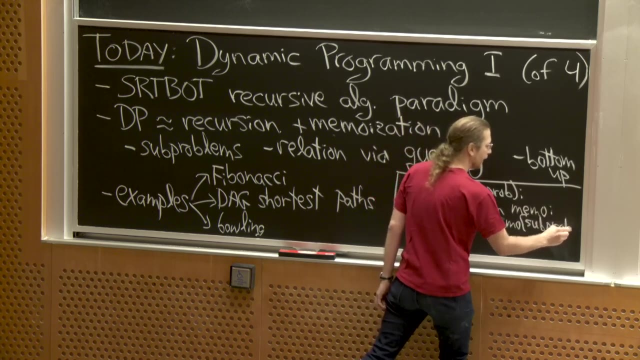 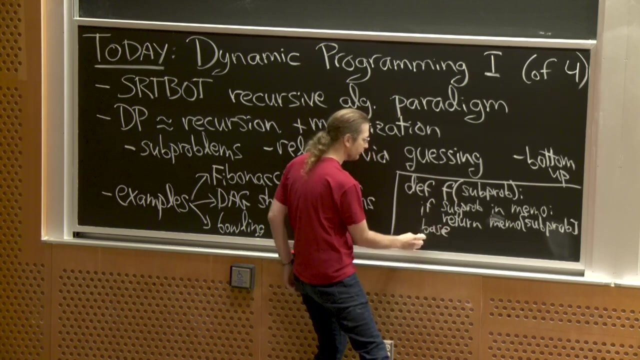 Is the subproblem in the memo table. If so, return memo of subproblem And otherwise check if it's a base case and solve it. if it's a base case And otherwise write the recurrence, Recurrence, Recurrence. 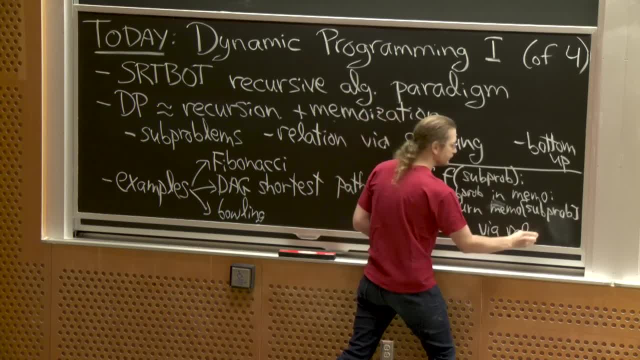 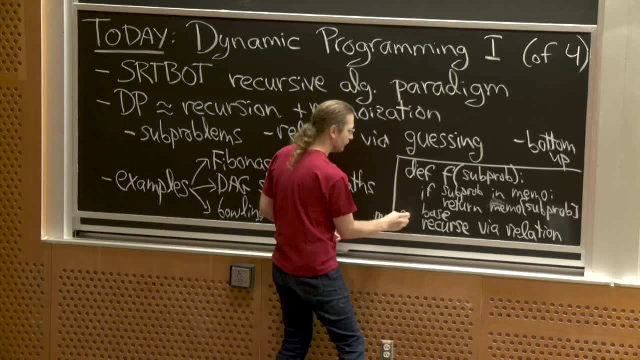 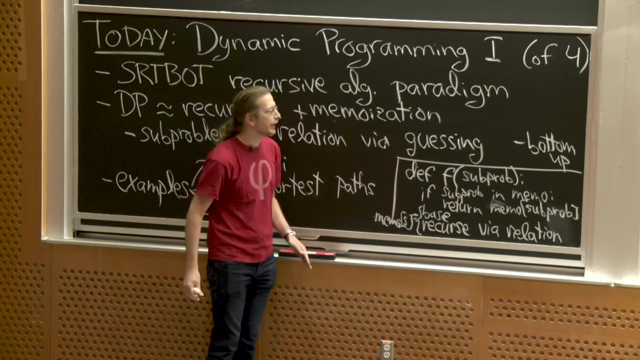 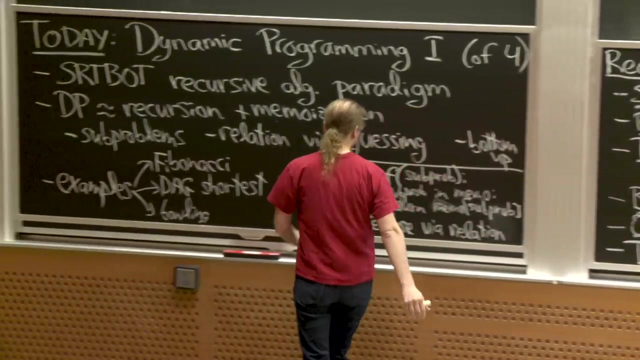 Recurrence via relation and set the memo table of the subproblem to be one of those things. So this is the generic dynamic program And implicitly I'm writing Fibonacci in that way And all of the dynamic programs have this implicit structure where I start with a memo table which is empty. 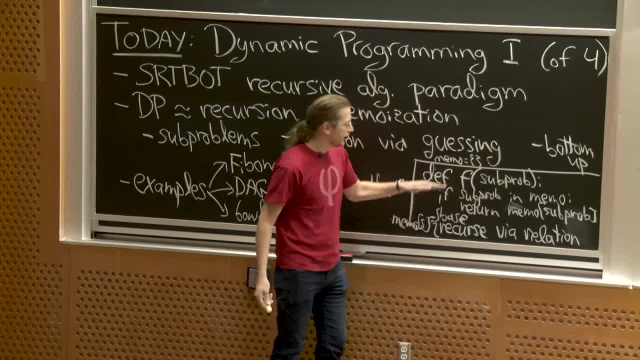 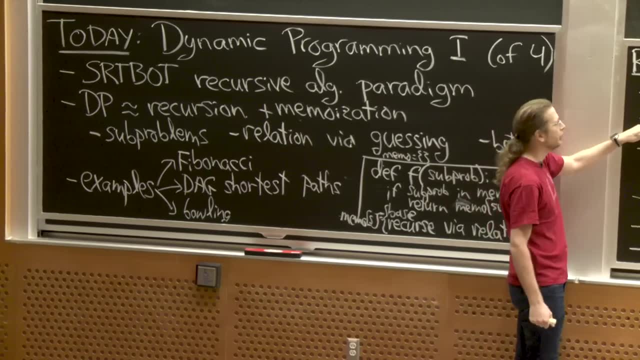 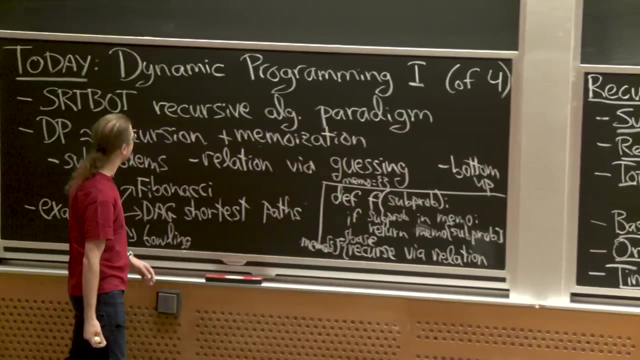 And I always just check if I'm in the memo table. If I am, I return it. Otherwise I compute according to this recursive relation by recursively calling F And that's it. So this is. every DP algorithm is going to have that structure. 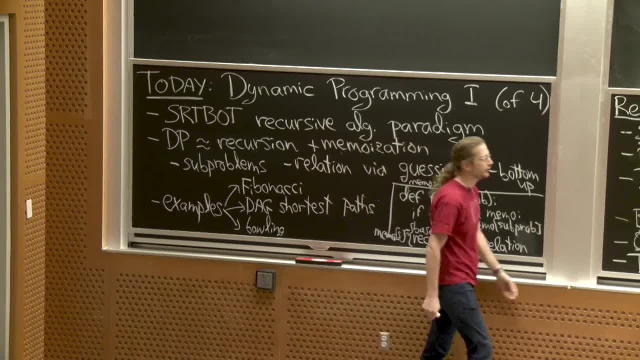 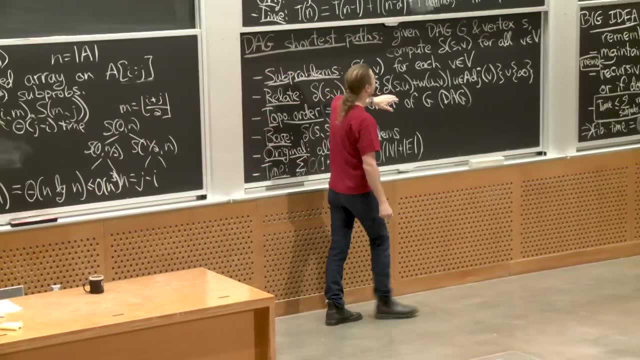 And it's just using recursion and memoization together. OK, So now let's apply that technique to think about, Let's talk about the DAG- shortest paths problem. The problem was: I give you a DAG, I give you a source, vertex S, single source- shortest paths. 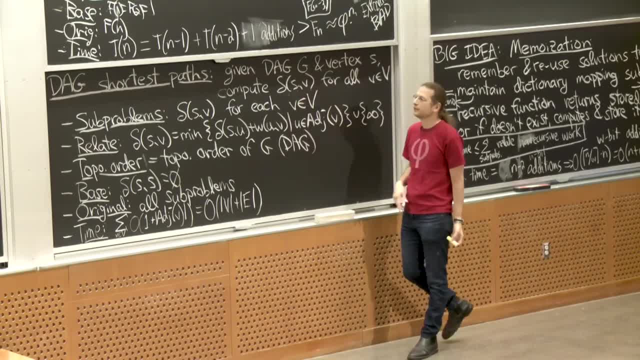 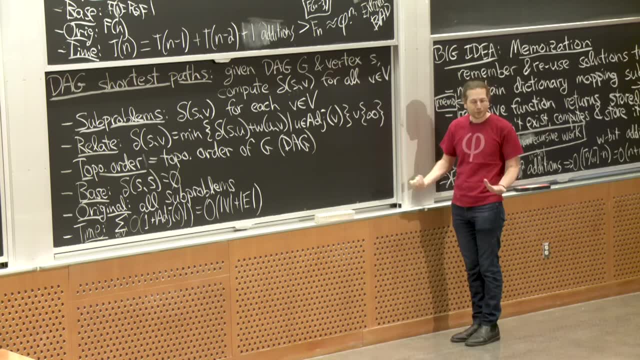 Compute the shortest path weight from S to every vertex. That's the goal of the problem, And we saw a way to solve that, which is DAG relaxation. I'm going to show you a different way, which turns out to be basically the same, but upside down. 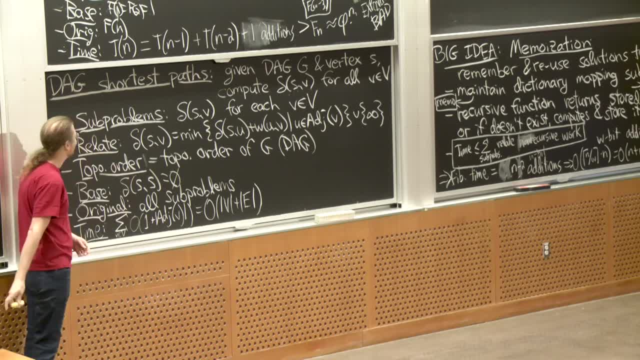 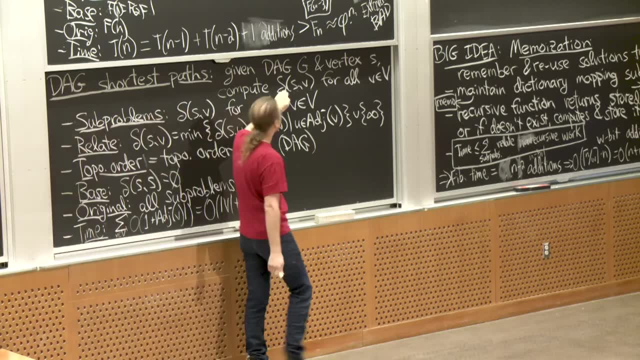 or flipped left to right, depending which way you direct your edges. So what are our subproblems? Well, here, actually, they're kind of spelled out for us. We want to compute delta of SV for all V, So that is size of V. subproblems: 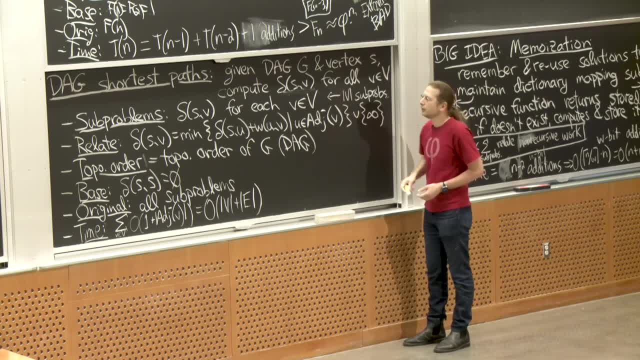 That turns out to be enough for this overall problem, And the original problem we want to solve is all of the subproblems. We solve all the subproblems, we're done. And then we have- I think we wrote this at some point during the DAG- shortest paths lecture. 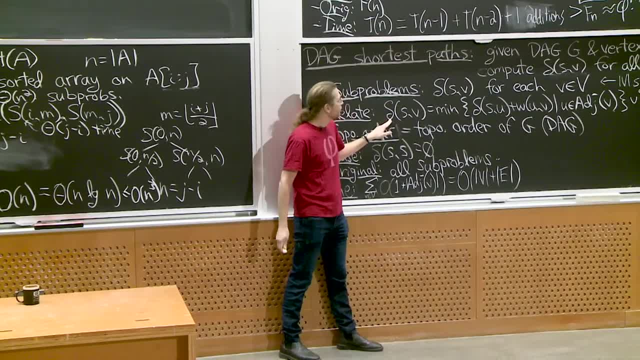 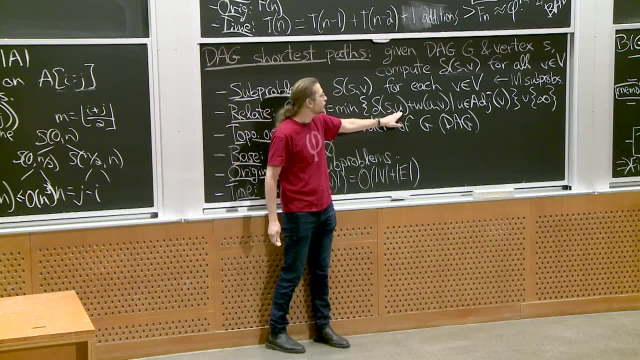 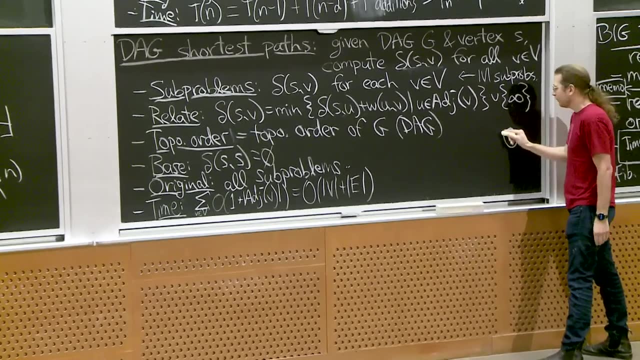 We have a recursive relation saying that the shortest way to get from S to V is the minimum of the shortest path to get to some vertex U plus the weight of the edge from U to V. Why? Because if we look at a vertex V unless we started there, 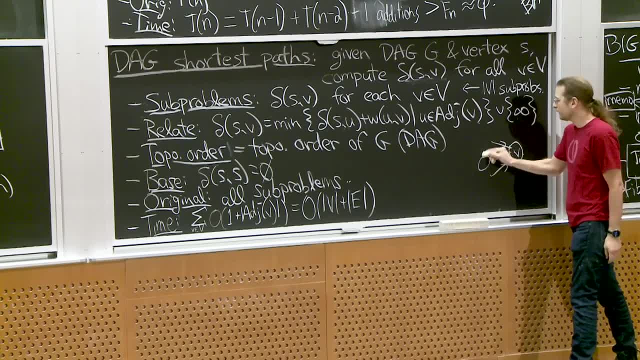 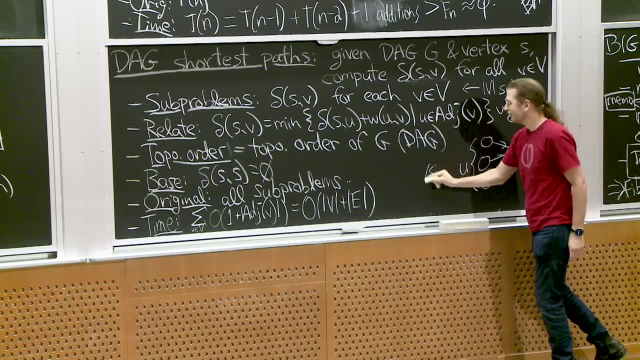 we came from somewhere, And so we can consider all of the possible choices for the previous vertex U, And if you start at S and get to V, you must go through one of them, And so this is finding the best way among all of them. 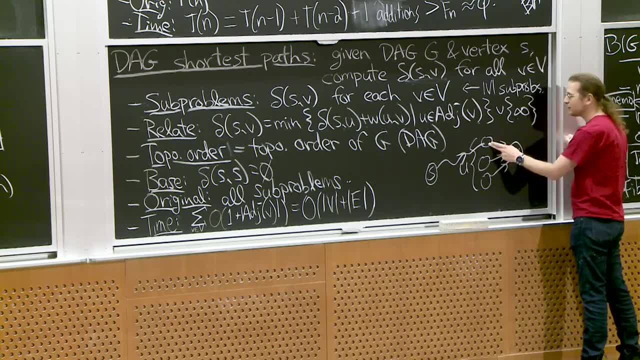 to get to some vertex U, And if you start at S and get to V, all the choices of U, what's the best way to get to U and then take the edge from U to V, For all edges, U, V, And this is adjacency minus. 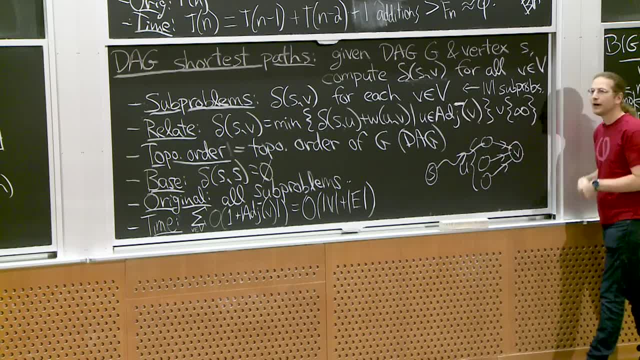 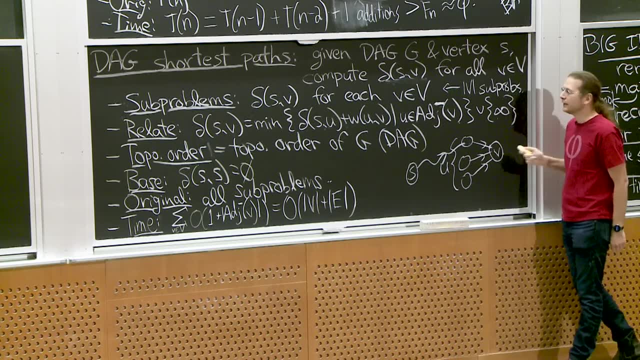 We don't usually think of that. Usually we look at adjacency plus the outgoing edges. This is the incoming edges, And so U is an incoming, UV is an incoming edge into V. If we take that minimum- and of course it's possible- 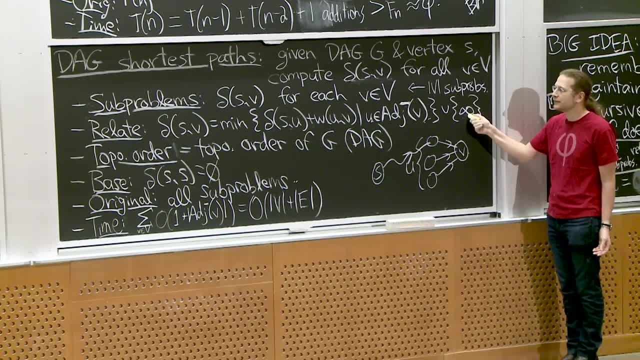 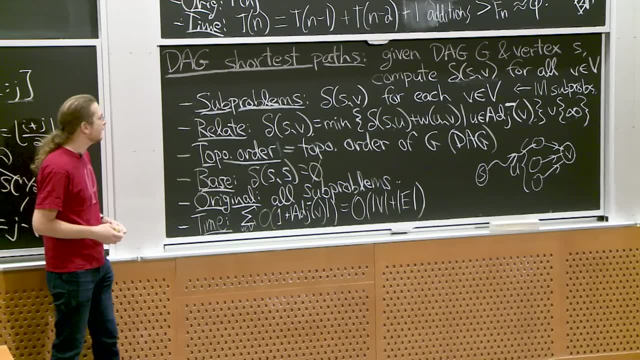 there is no way to get to V, And so I'll also throw infinity into this set. Take the min of that set. That will give me the shortest pathway in an acyclic graph from S to V. And great, this is recursive. 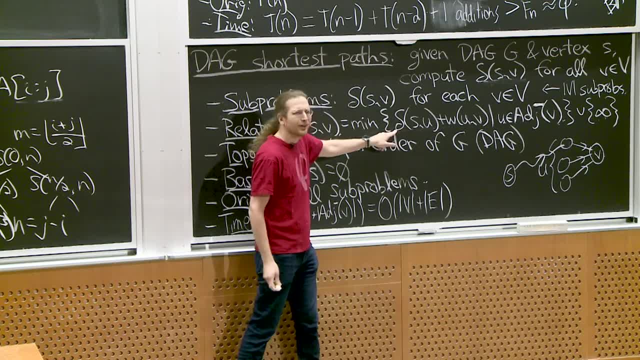 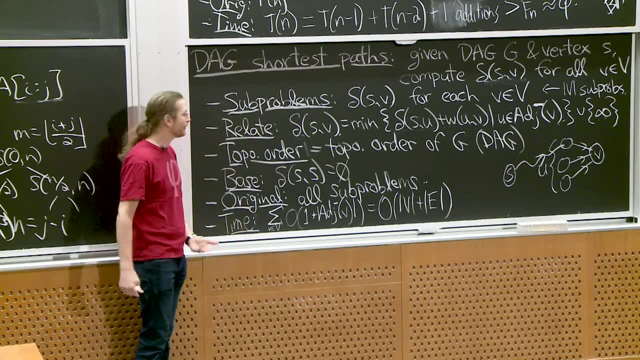 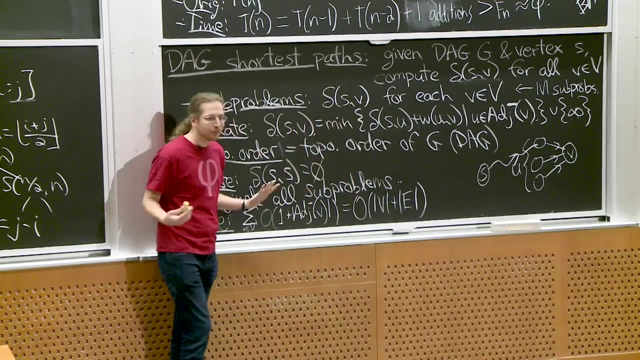 This was a subproblem. These are subproblems which are smaller. I guess There's no clear notion of smaller here, except we already know. the clear notion of smaller is the topological order of our DAG, Because our graph is acyclic, we know. 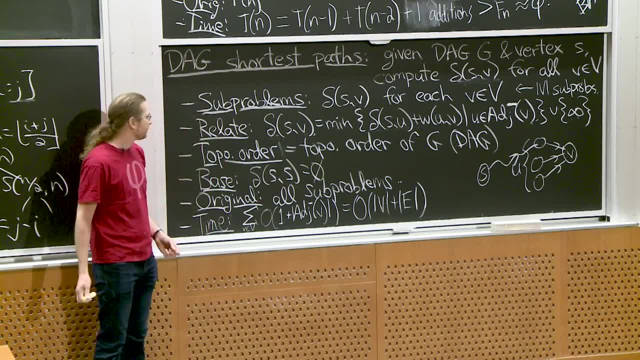 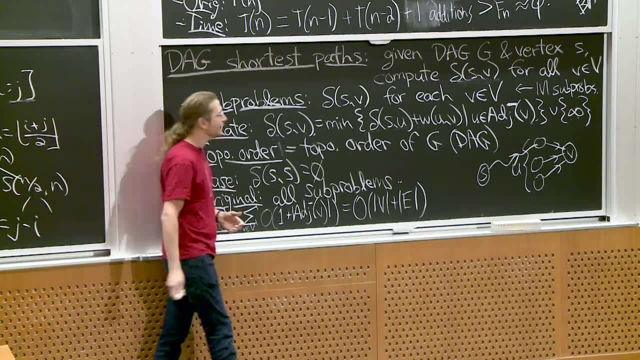 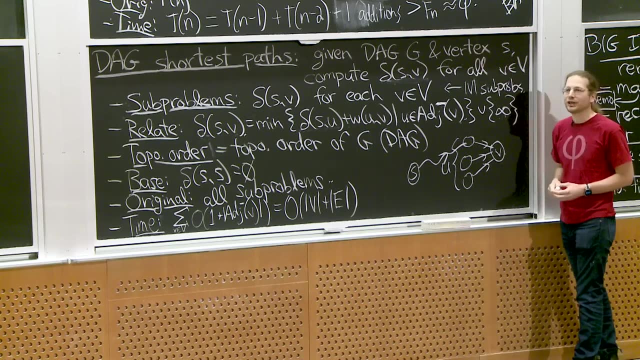 it has a topological order. We know how to compute it with DFS, And so that guarantees there is a topological order to compute these problems And in fact, the relationship between problems is exactly the given. graph G In order to compute the shortest path: weight from S to V. 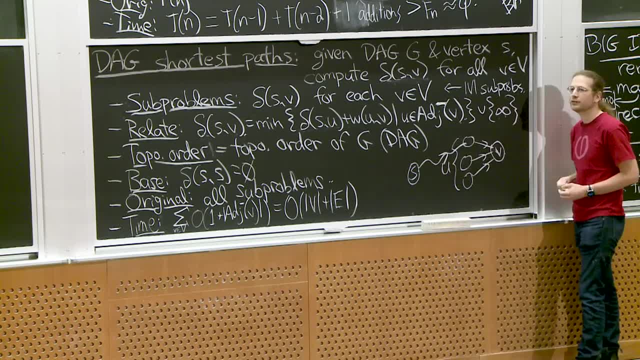 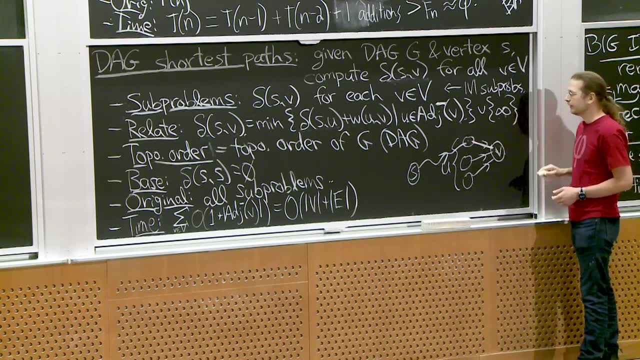 I need to know the shortest path weight from S to all of the incoming vertices to V, And so this is, I guess, in the call graph, this vertex calls this vertex. But I'll go ahead, I'll direct the edge this way to say. 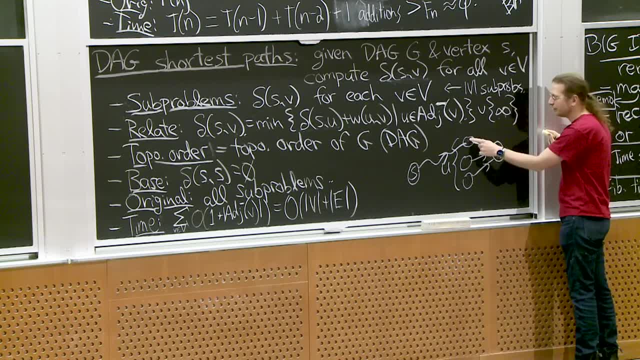 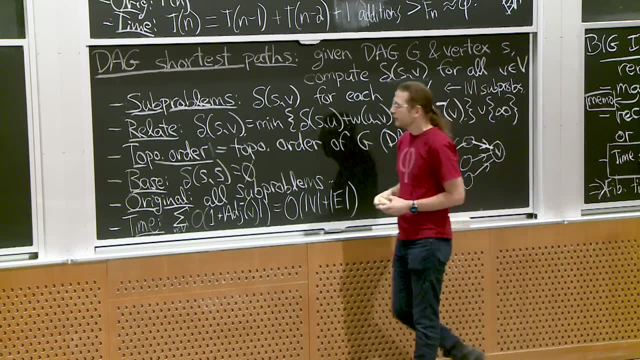 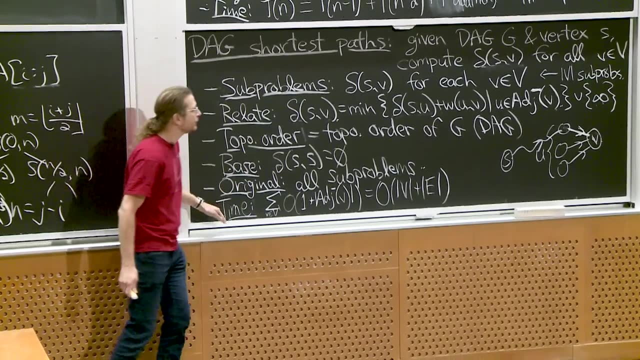 that this vertex requires. this vertex needs to be computed before this one, And so then I can compute them in a topological order. We have a base case which is delta of SS equals 0. And the running time is. again, we can use this formula. 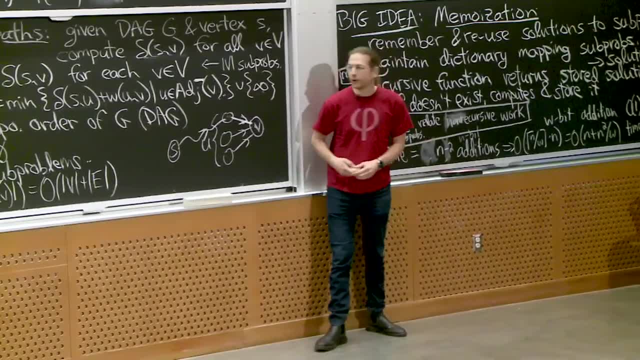 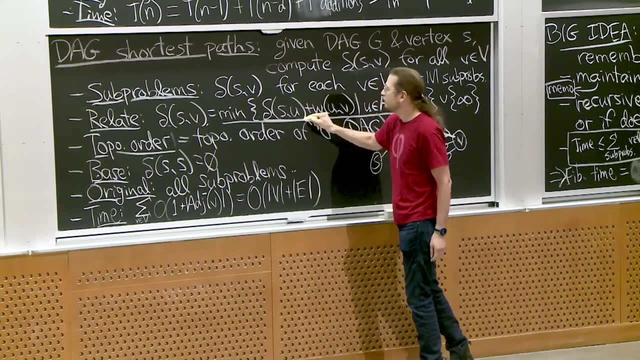 and say: let's just sum over all the subproblems of the non-recursive work in our recurrence relation. And so it's computing this min. If I gave you, OK, OK, OK, These deltas for free, and I gave you. 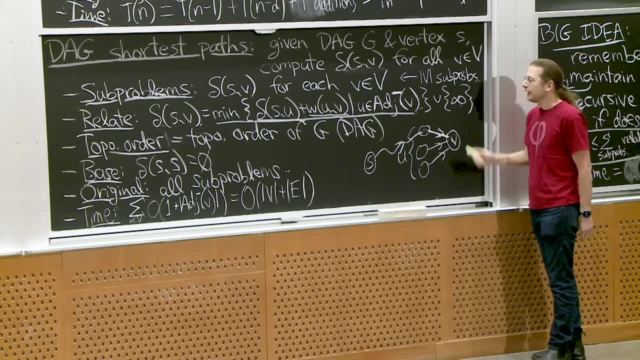 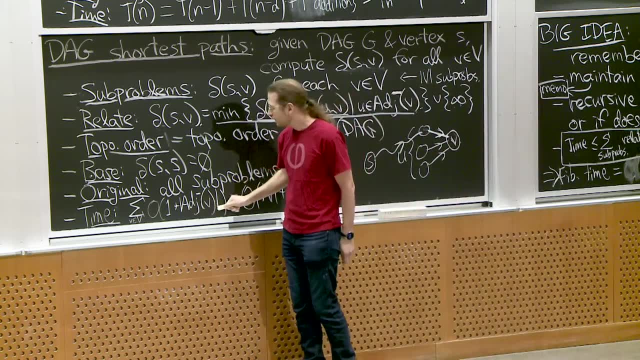 these weights which we know from our weight data structure. how long does it take to compute this min? Well, however many things there are, how many numbers we're minning, which is the size of the incoming adjacency list plus 1 for that infinity. 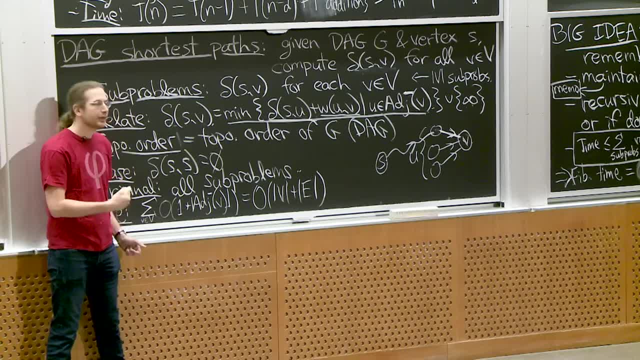 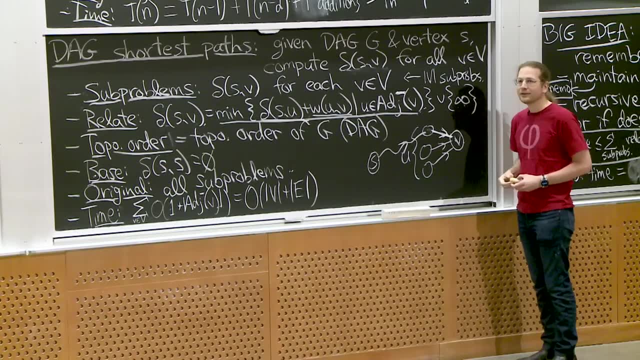 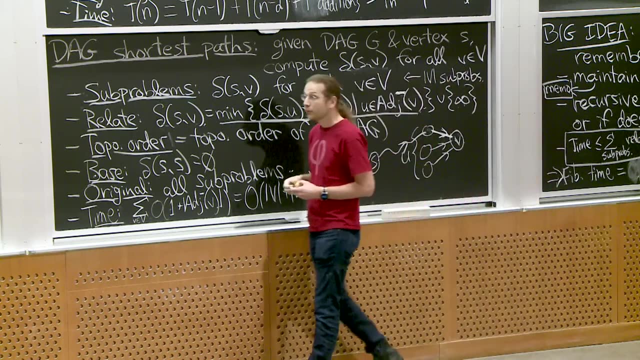 And so if you compute this sum, sum of incoming edges, to every vertex, that's all the edges. So this is V plus E. OK, So in fact this algorithm Is morally the same algorithm as the one that we saw in the DAG shortest path lecture, which 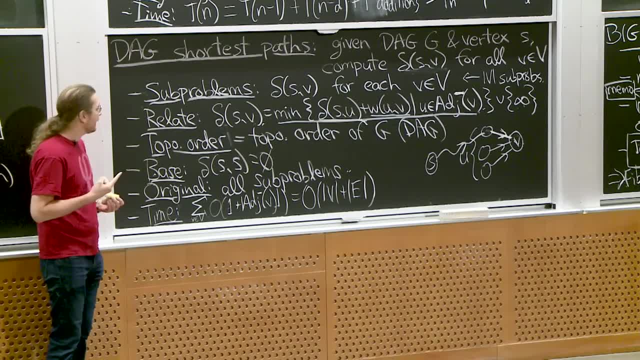 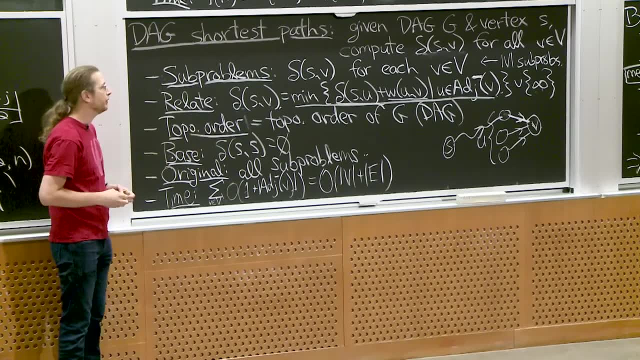 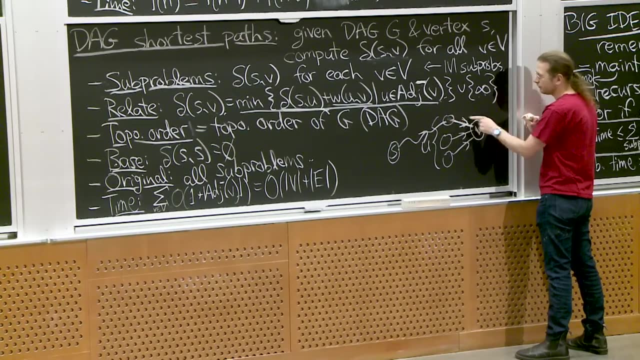 was computer topological order and process vertices in that order and relax edges going out from vertices. So here, so in that algorithm, we would have tried to relax this edge if there was a better path to V, And the first one certainly is better than infinity. 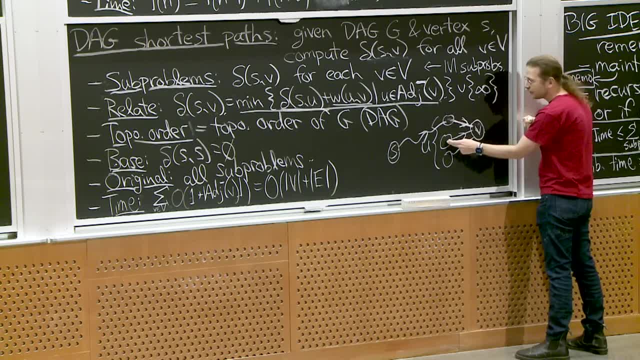 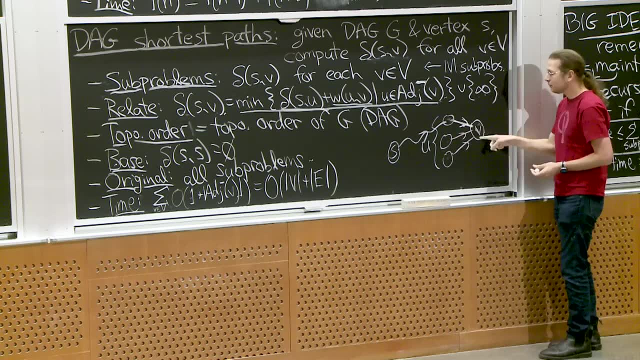 So the first one: we relax, Indeed, Indeed. The next edge. if this gave a better path from S to V, then we would relax that edge and update the weight here and do the same here. In the end we're just computing this min in the relaxation. 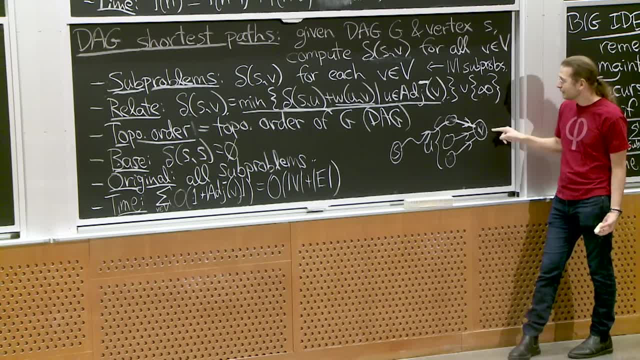 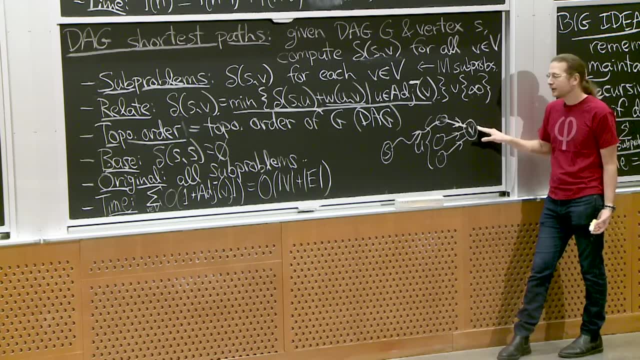 algorithm, but doing it step by step. In the relaxation algorithm, DAG relaxation- for each incoming edge to V, we update D of V if it's better, And so if you repeatedly update if you're better, that ends up computing a min. 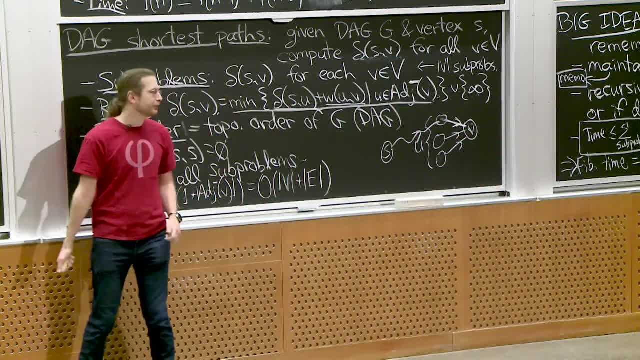 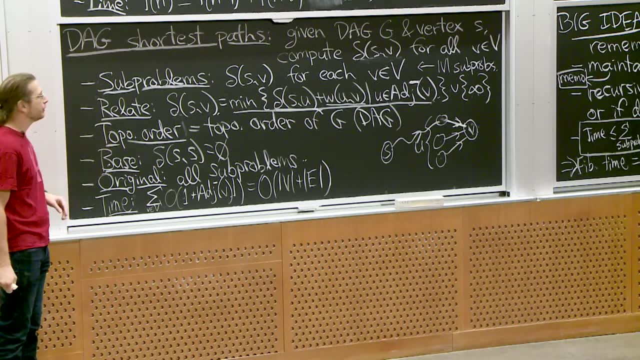 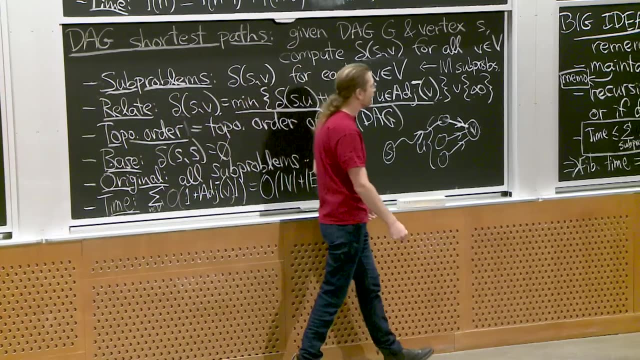 OK, So this is the same algorithm, just kind of flipped backwards. A funny thing: although we wrote down the topological order of the subproblem graph, here is the topological order of G. because the subproblem graph is G, the algorithm doesn't actually have to compute one. 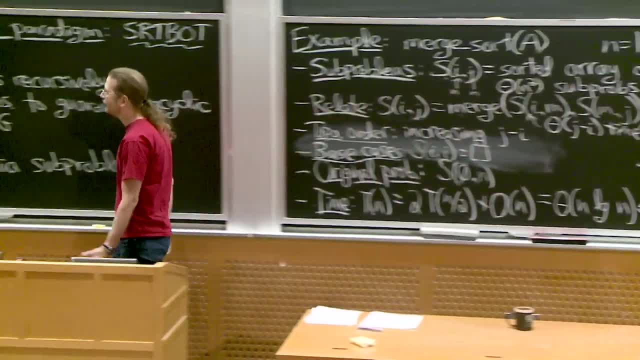 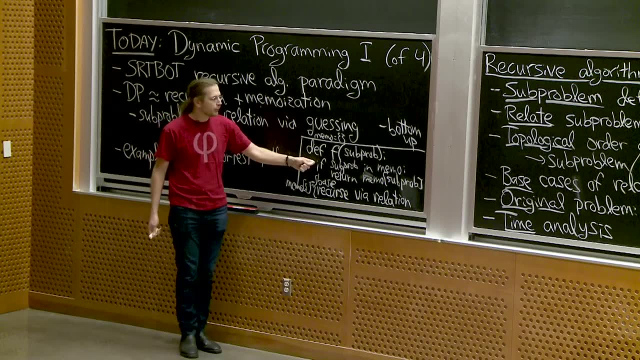 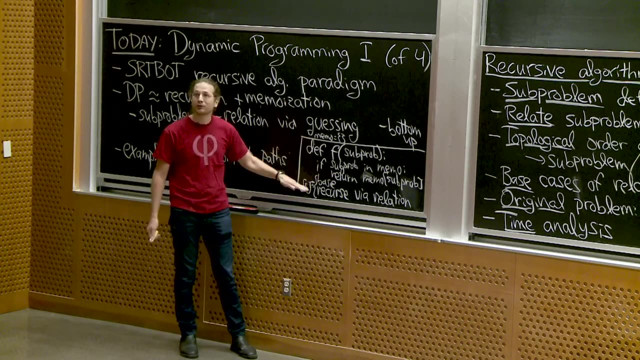 It's doing it automatically for free. If you think about this algorithm, generic D-P algorithm- which is Check whether we're in a memo table. If so, return, Otherwise recurse or base case, This actually is a depth-first search. 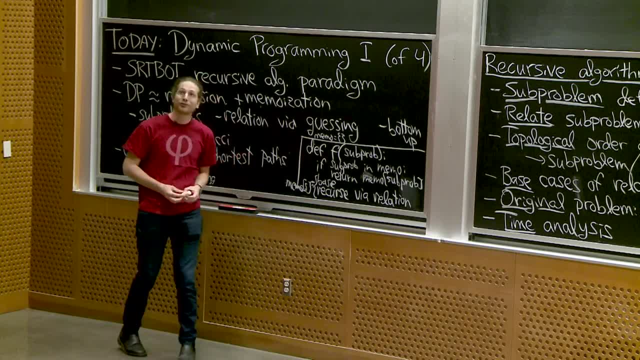 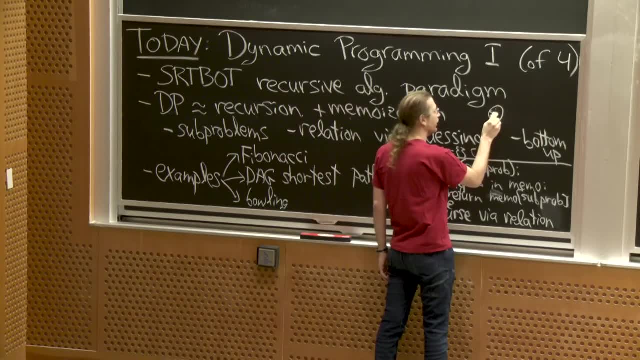 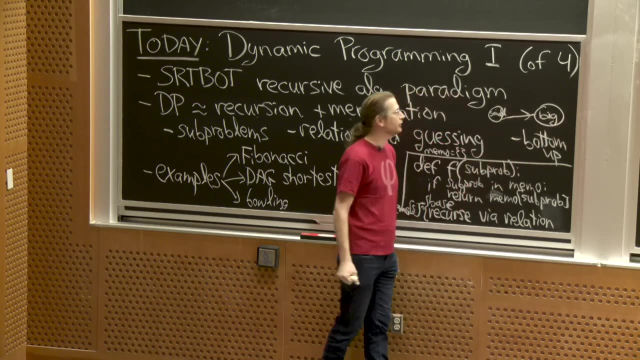 through the subproblem graph, technically through the reverse of the subproblem graph. If I draw an edge, so from small to big. So I'm just saying I orient the edges from my smaller subproblems to the ones that need it, Then I'm actually a depth-first searching backwards. 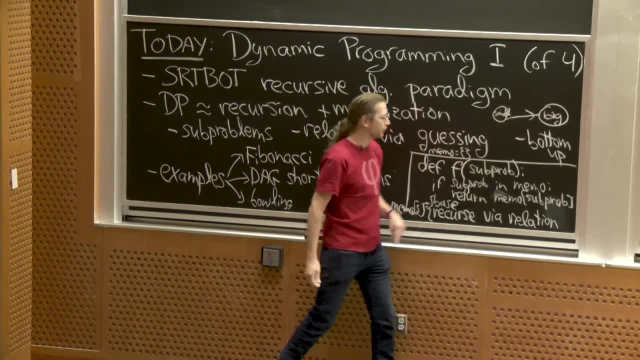 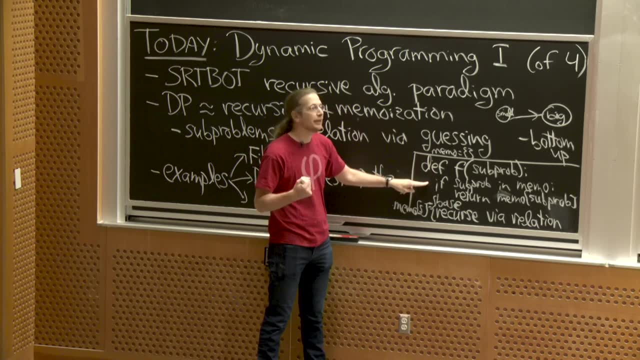 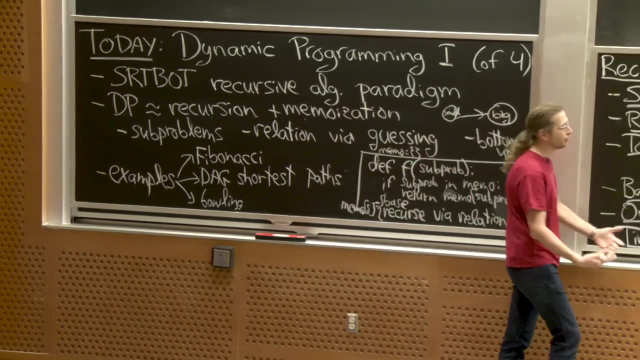 in this graph because the bigger problem calls the smaller problem And the memo table is serving as the. have I visited this vertex already? check in DFS. So this is actually a DFS algorithm plus. we're doing some computation to actually solve the subproblems we care about. 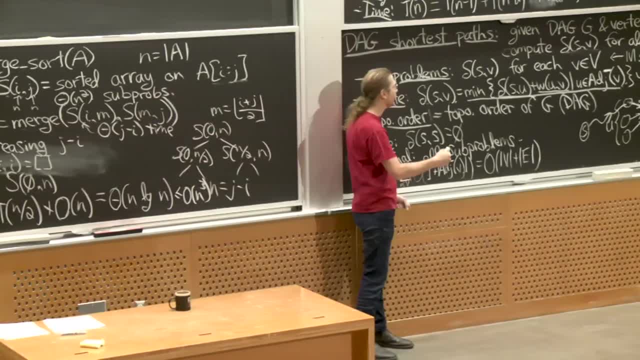 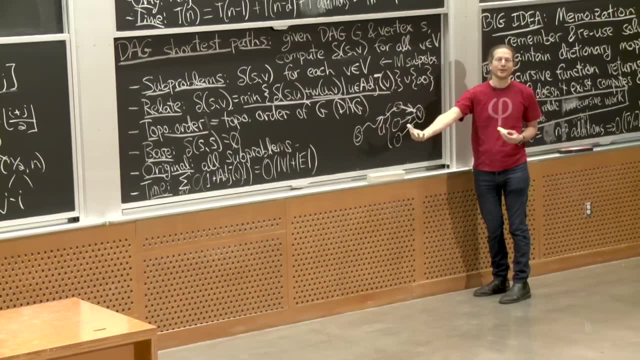 So, implicit in this algorithm, we are doing a DFS And at the same time we're doing this shortest path computation In the finishing order of that DFS traversal, because all the edges are backwards. this is the same as the reverse finishing order. 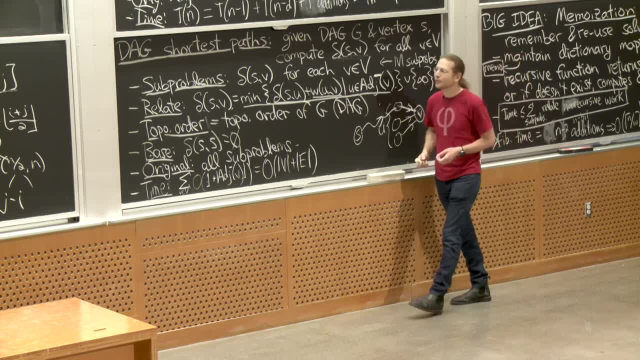 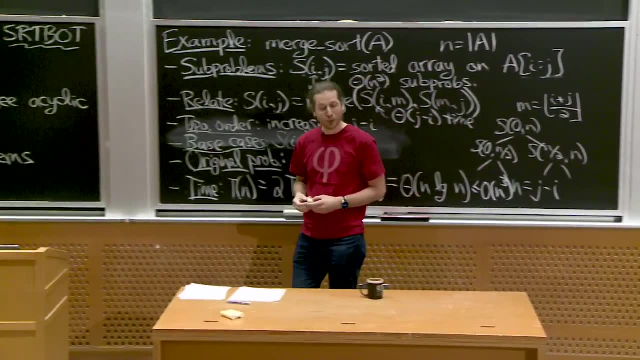 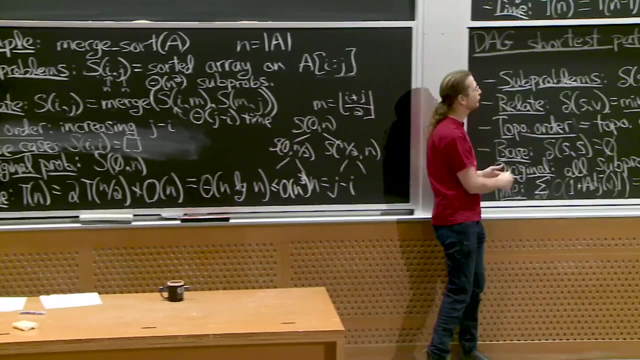 if the graph is forwards. So in the end we're computing a topological order, because dynamic programming includes in it depth first search, A lot of words. But it's kind of cool that this framework just solves DAG shortest paths without much work. 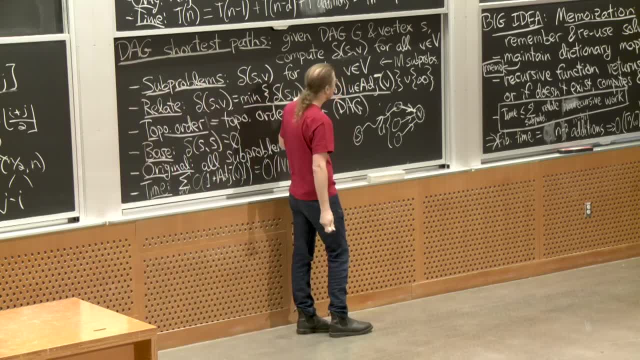 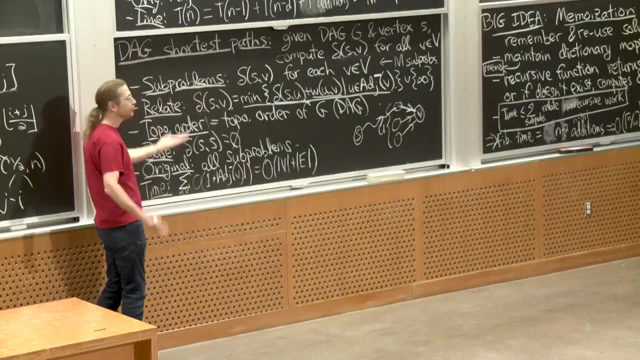 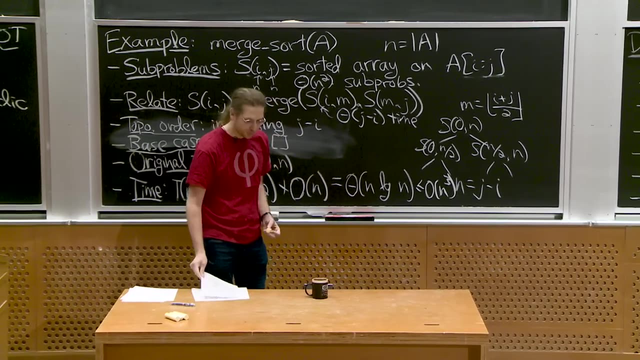 I mean, we did a lot of work in shortest paths to prove that this relation is true. Once you know it's true, the algorithm part is pretty much free. You just write down sort thought and you're done. OK, This brings us to in general at this point. 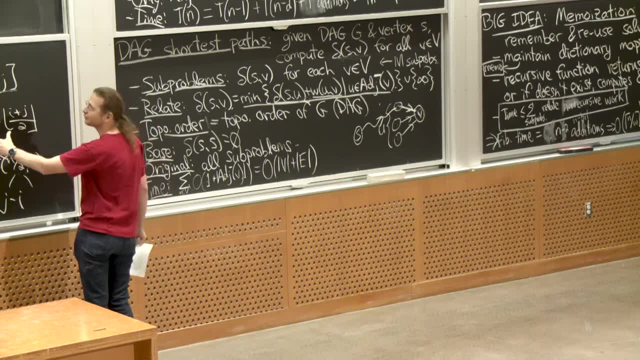 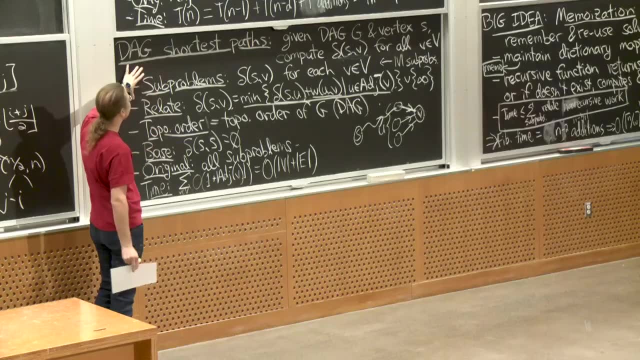 we have seen two examples of dynamic programming. I guess technically merge sort you could think of as a dynamic program but it doesn't actually reuse anything, So it's not interesting And indeed that gave us a really bad bound. But we've definitely seen DAG, shortest paths and Fibonacci. 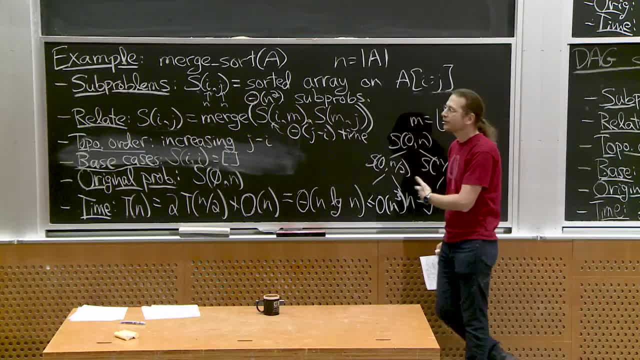 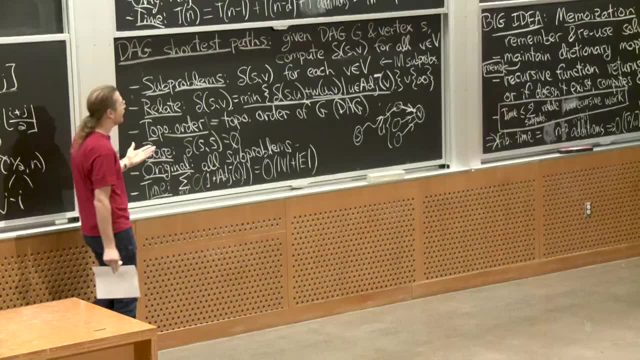 numbers as two interesting examples, And what the next remainder of this lecture and the next three lectures are going to be about is more and more examples of dynamic programming and how you can use it to solve increasingly general problems. So far, we've just solved an easy problem and a problem. 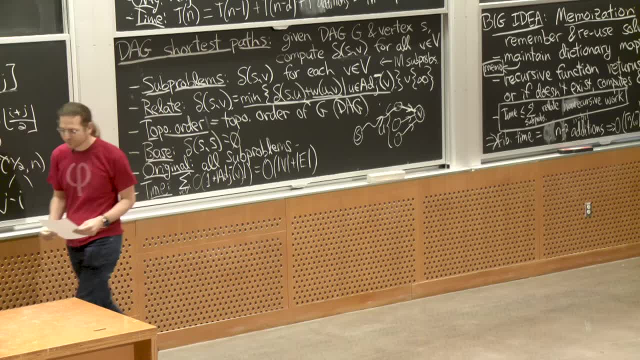 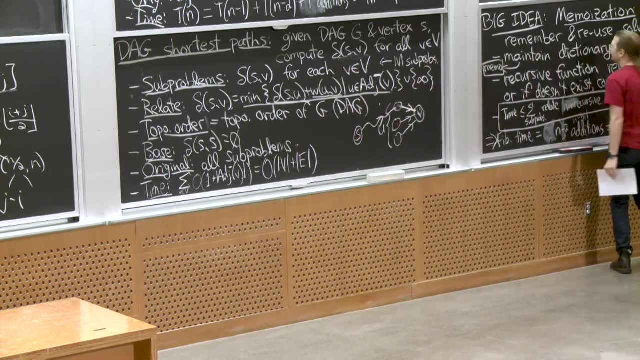 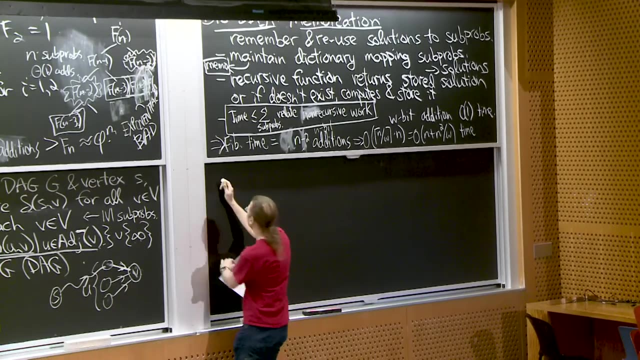 we already knew how to solve. Let's go to a new problem, which is bowling. Bowling is popular Boston. Boston likes to play candle pin bowling, which is a bit unusual. Today, we're going to play an even more unusual bowling game. 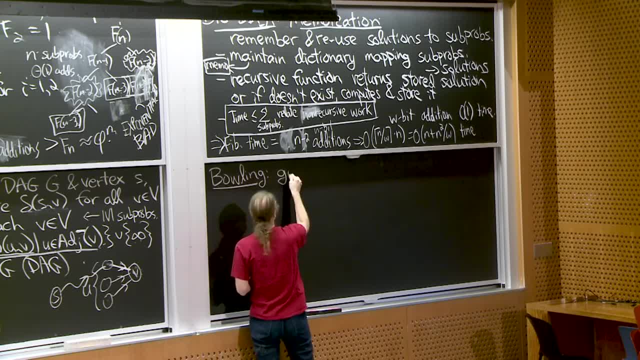 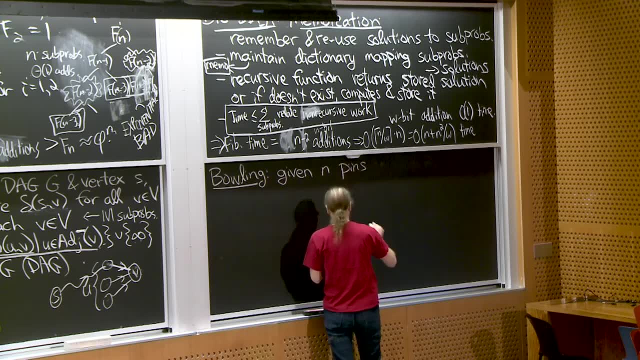 one that I made up, based on a bowling game that Henry Doudny made up in 1908.. So ancient bowling you might call it, Or I think linear bowling is what I might call it. I'll just call it bowling here. 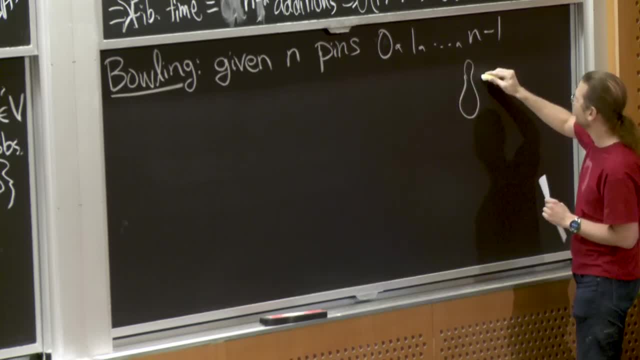 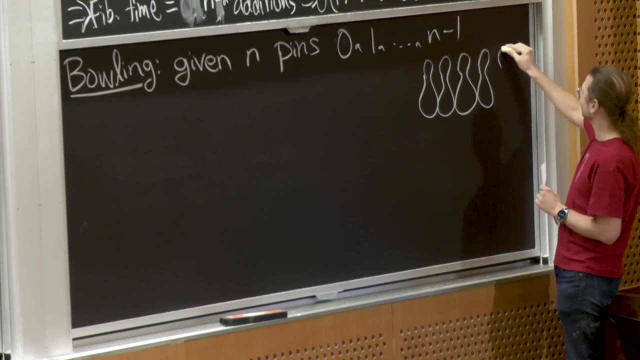 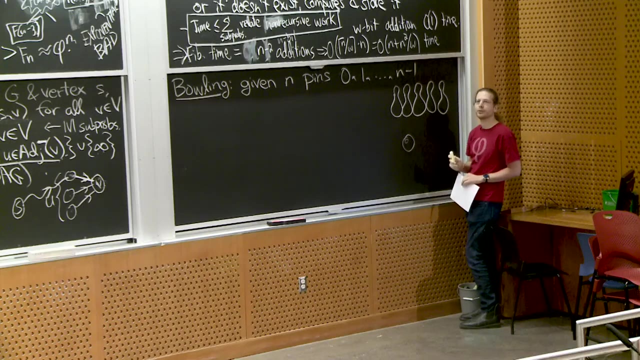 And now I'm going to attempt to draw. Draw a bowling pin, not bad. That might get progressively worse. So imagine n identical bowling pins. Please pretend these are identical And I have a ball which is approximately the same size as a bowling pin. 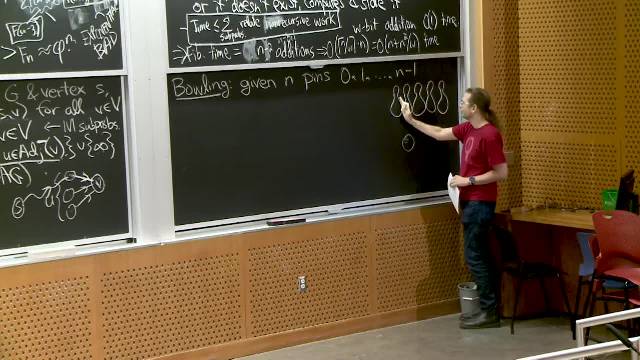 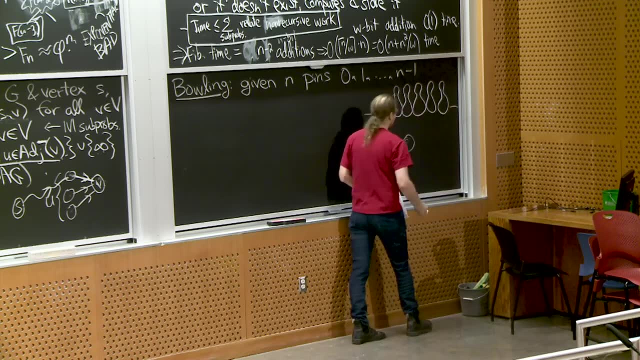 These bowling pins are pretty close together. I should have left a little gap here, And you are a really good bowler. Now, unfortunately, these bowling pins are on a line And you're bowling from way down at infinity. OK, So when you bowl, you can only hit one pin or two pins. 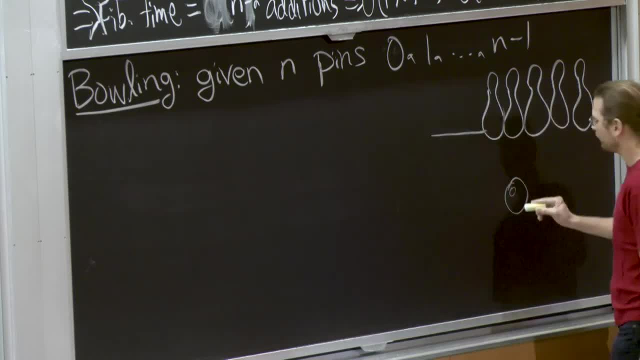 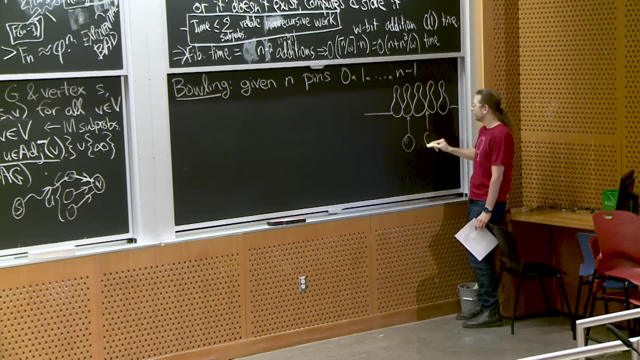 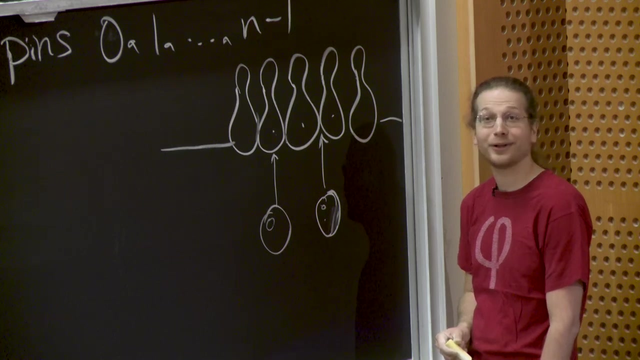 or zero pins, But probably you want to hit some pins. So if you bowl straight at a pin you will just hit that one pin, And if you bowl in the middle between two pins you will knock down two pins. This is your model of bowling, model of computation. 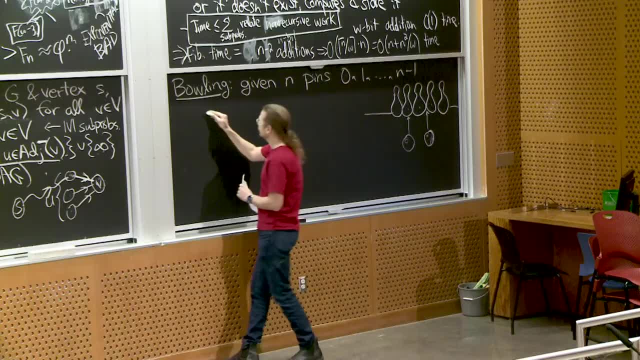 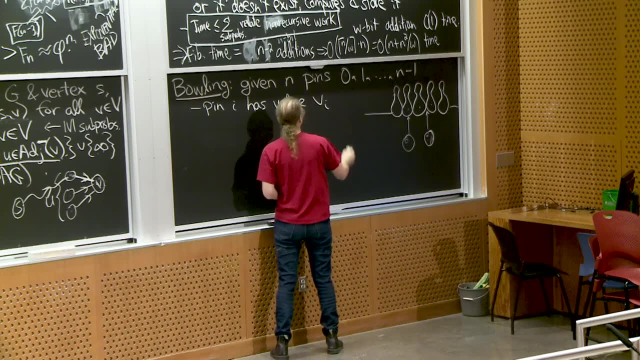 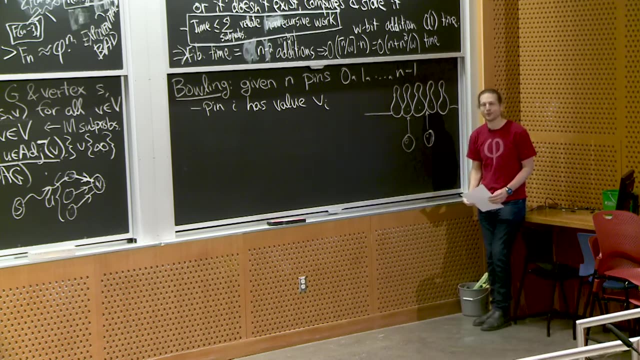 Now, what makes this interesting is that the pins have values. Pin i has value v i. This is obviously a toy problem, Though this problem, this type of bowling, does go back to 1908, it was also a toy problem in that setting. 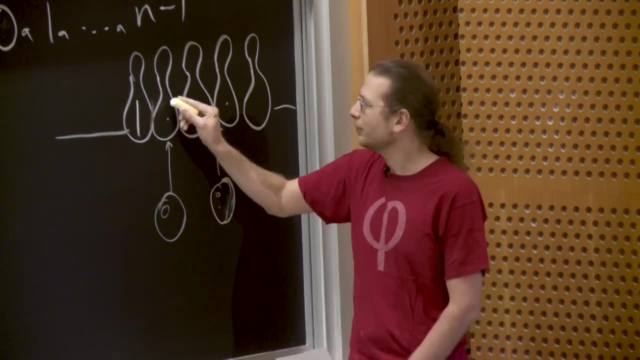 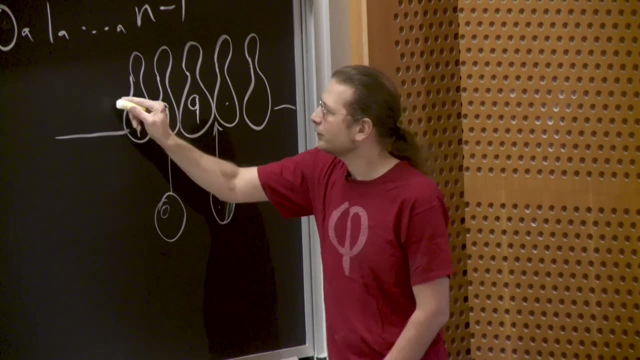 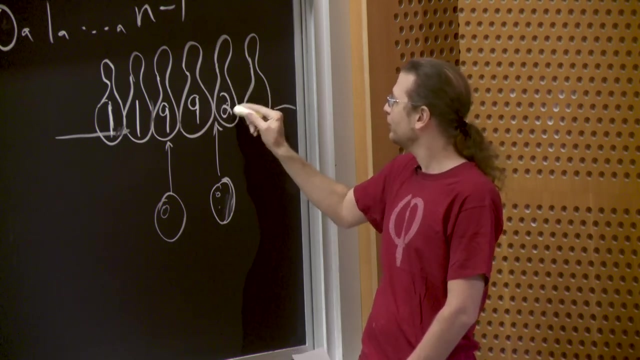 So each of these bowling pins has some number on it, Let's say 199.. Let me do a slightly more interesting example. Maybe another 1 here and a 2, and a 5, and a 5,, something like this. 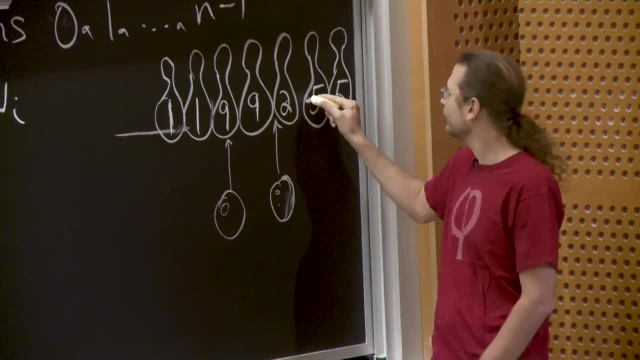 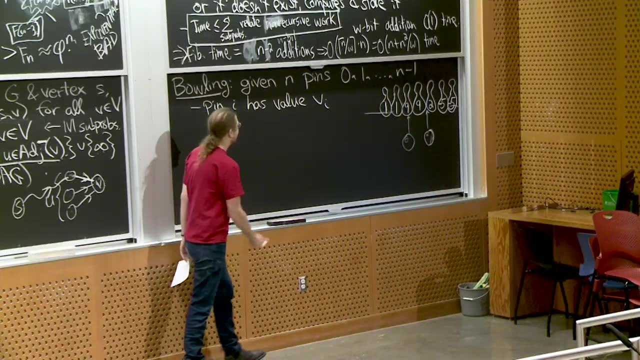 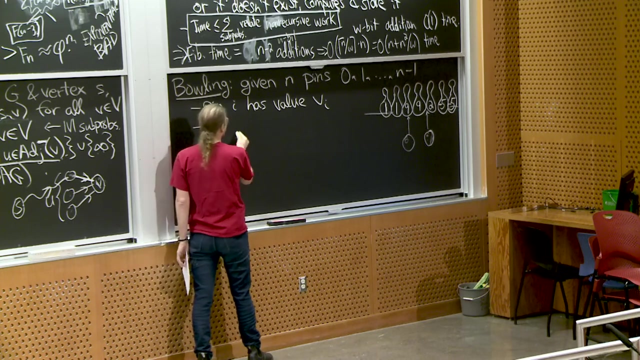 OK, Or maybe make it a little more interesting, Let's put some negative numbers on here. OK, And the model? so you're at the carnival bowling. Each pin has potentially different values, And the model is: if you hit one pin. 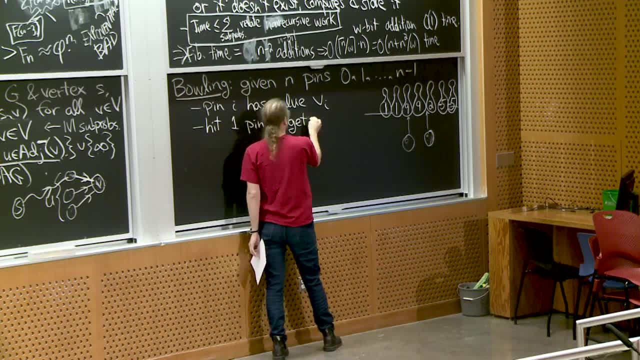 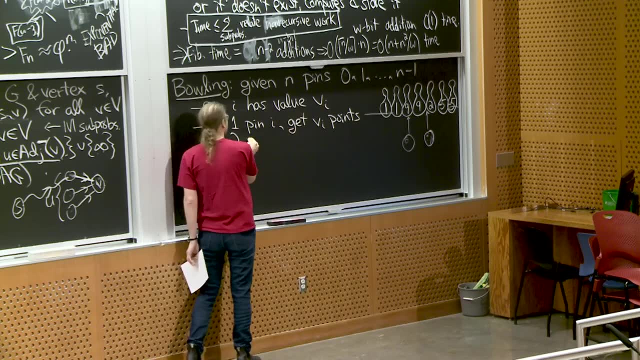 i, then you get v, i points. So that's straightforward. To make it interesting, when you hit two pins you get the product. So if I hit two pins, it's always i and i plus 1, for some i. 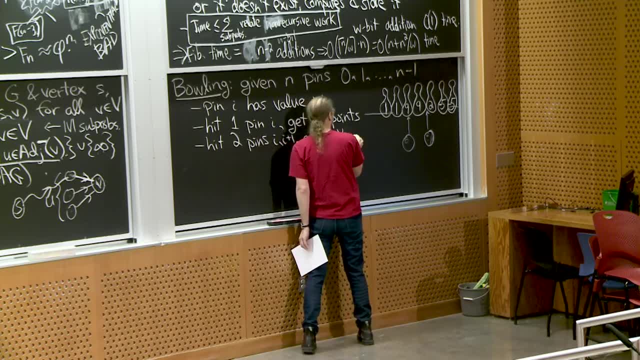 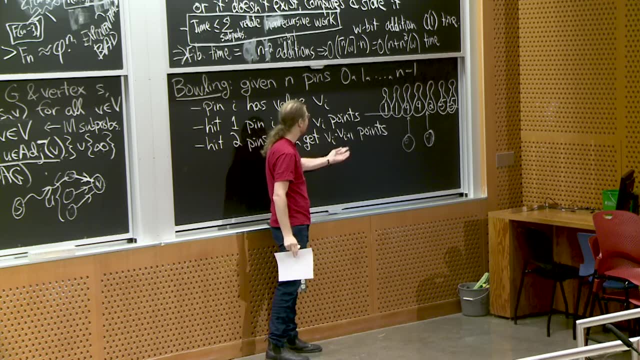 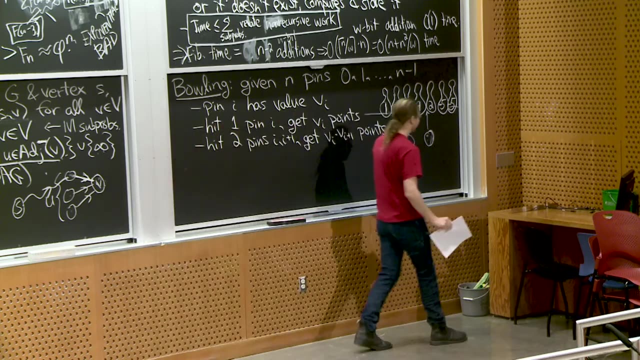 You get v i times v i plus 1 points. This is the game you're playing And it doesn't really matter that this is a product. The product is just some weird function That's hard to imagine If you stare at this long enough. 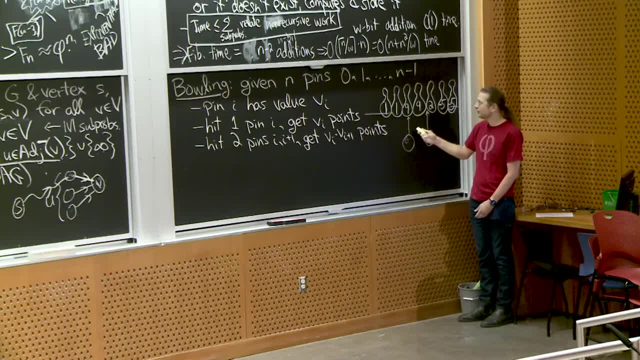 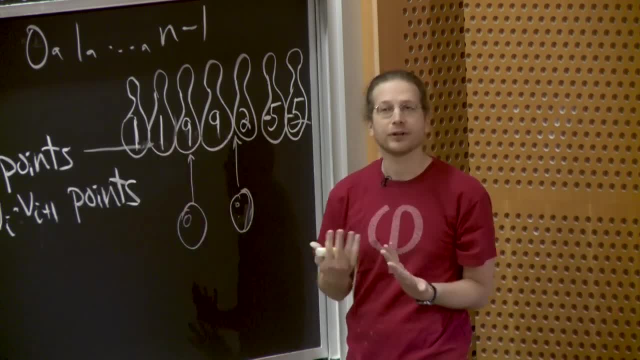 you should convince yourself that the optimal solution is probably to so for each of these numbers. I could leave it singleton, or pair it with its left neighbor, or pair it with its right neighbor, But the pairings can't overlap, Because once I hit a pin, it's gone. 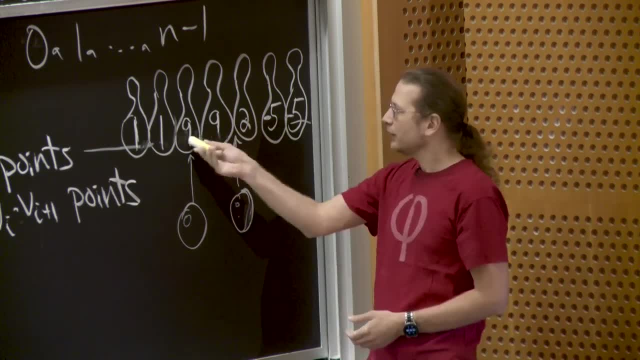 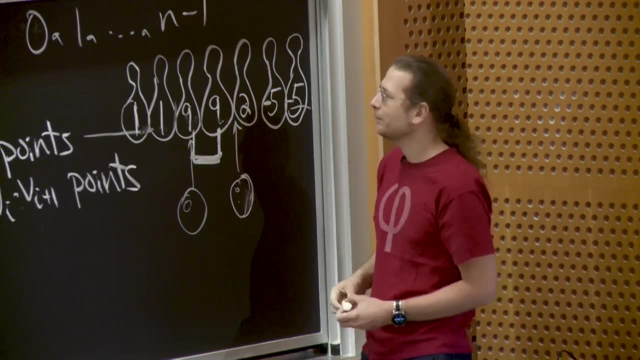 It's knocked over, It disappears. So, because of these 9s, which are very high value, what I'd probably like to do is hit both of them together. So pair them up, Because 9 times 9 is 81.. 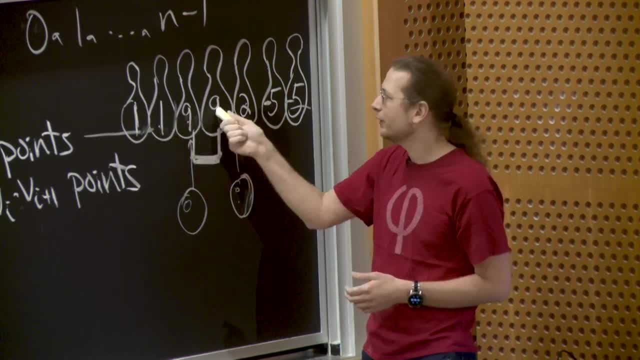 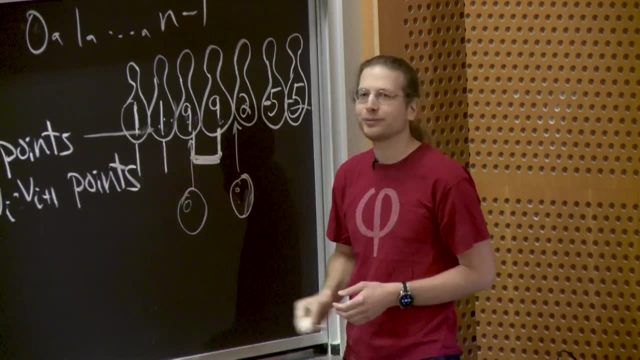 That's really big. much better than hitting them individually or hitting 9 times 1 or 9 times 2.. 1 and 1 is kind of funny because it's actually better to hit them individually. That will give you two points. 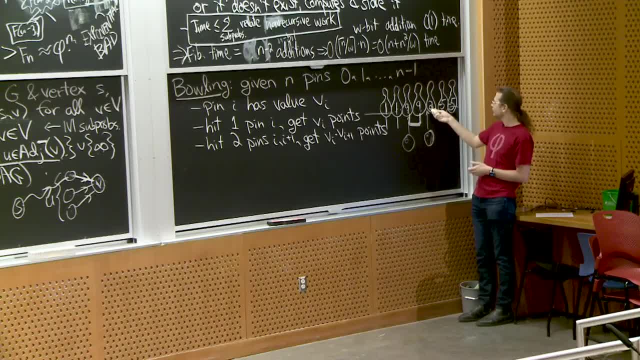 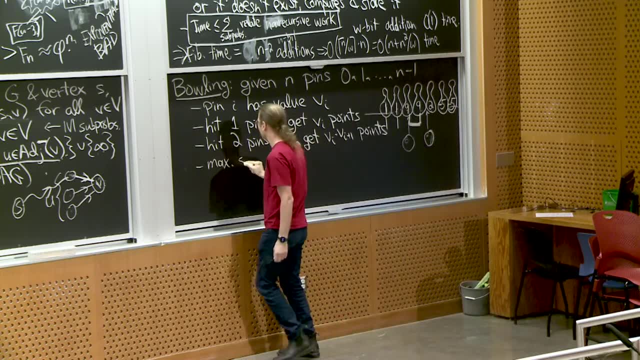 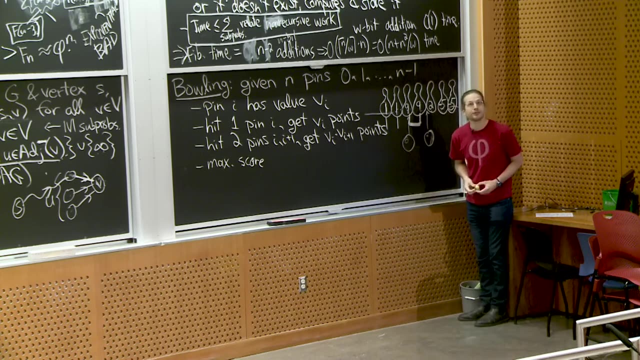 Whereas if I pair them up, I only get one point 2 and minus 5, that seems bad, negative 10 points. My goal is to maximize score. Do you have to hit all the pins? Let's say no, you don't have to hit all the pins. 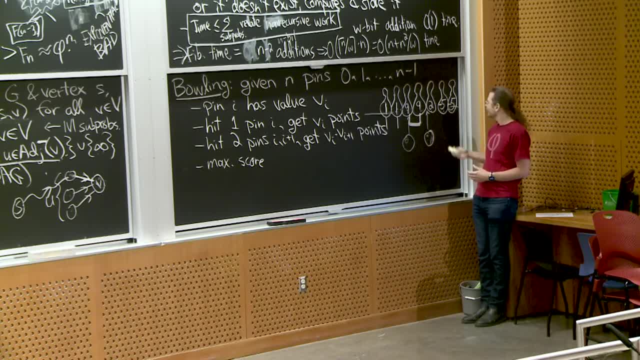 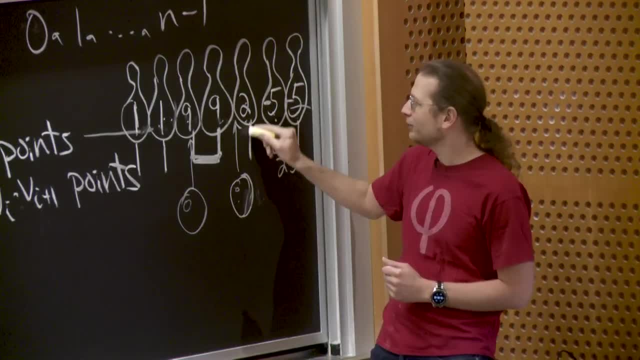 So I could skip the minus 5s. But in fact here, because they're adjacent, minus 5 times minus 5 is good, That's 25 points. So the optimal solution for this particular instance are to hit all the pins, these positive, these together. 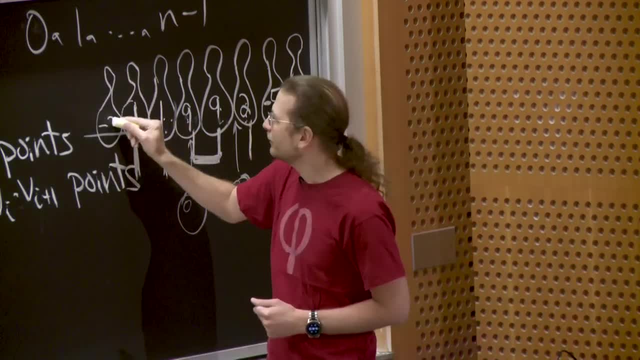 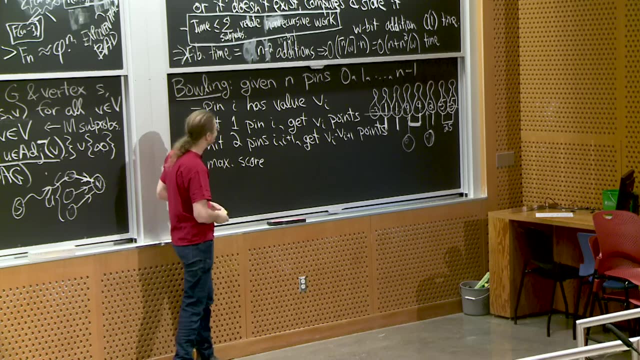 these together. If I added, for example, another pin of minus 3 here, I would choose not to hit that pin. Good question, So you just play until you are tired. When you decide to stop playing, how can I maximize score? 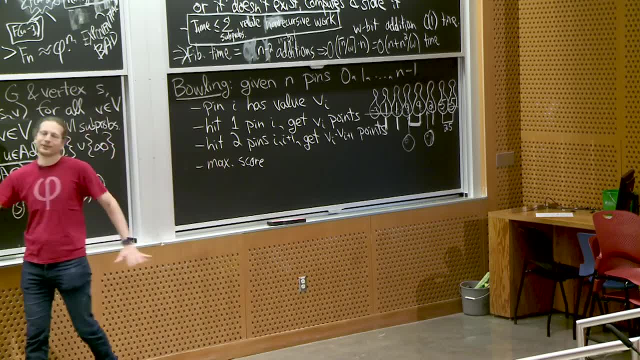 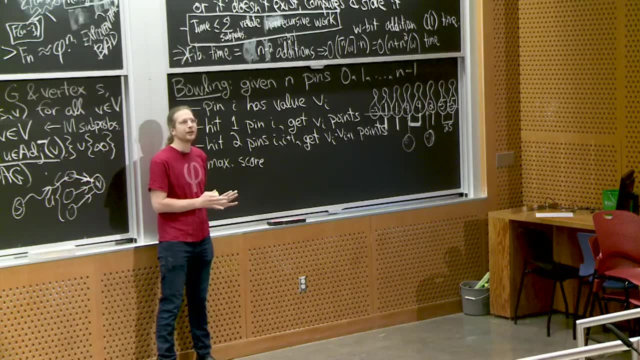 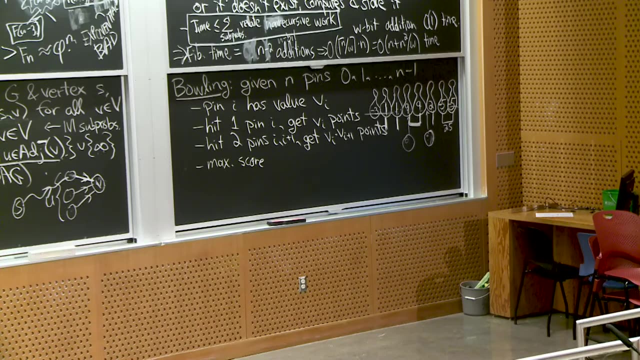 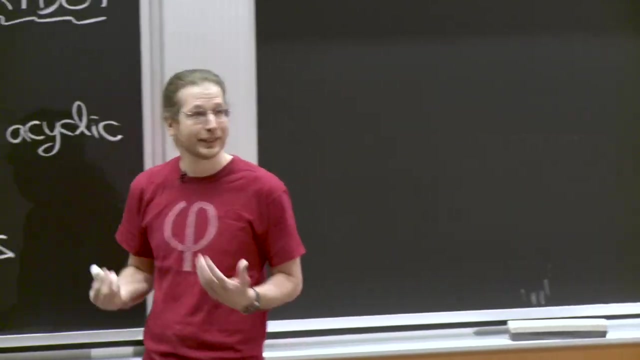 There are many variations in this game. All of them, basically any variation, not literally every variation, but many, many variations of this problem can all be solved quickly with dynamic programming, But let's solve this particular one, OK. So now we're really in algorithmic design mode. 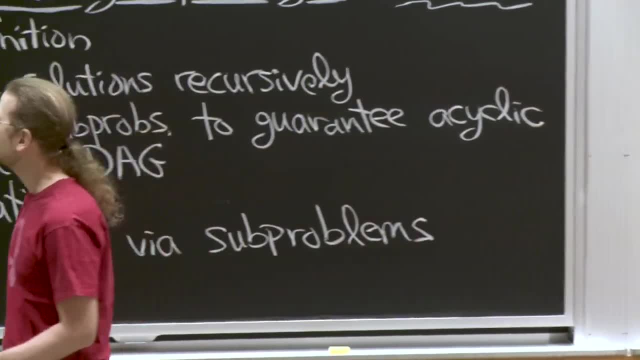 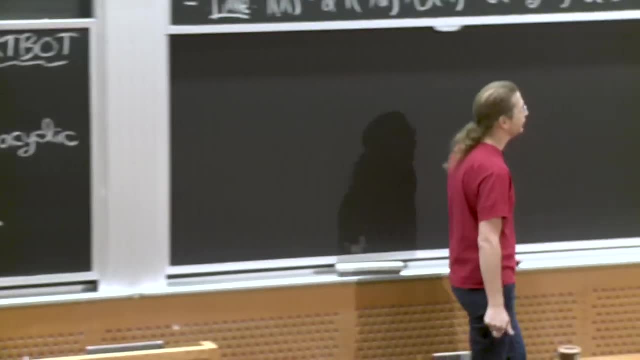 We need to think about sort bot And, in particular, we need to think about what would the subproblems be here And at this point we don't have a lot of help, So I should probably give you some tools If I want to solve a problem like this. 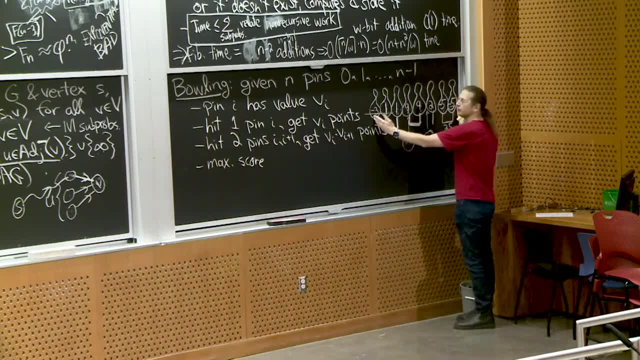 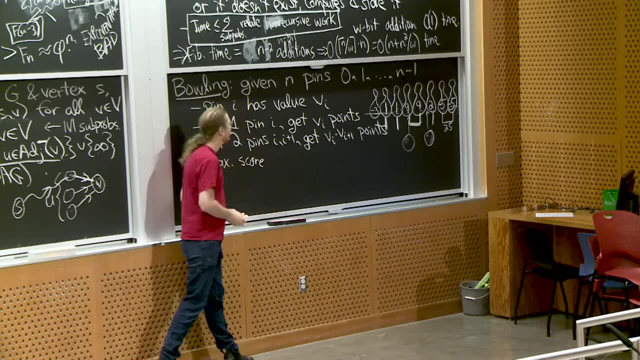 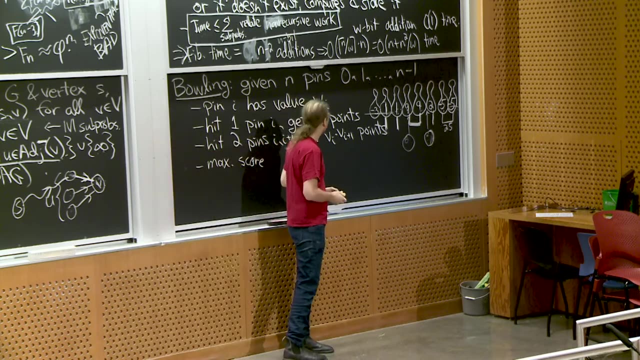 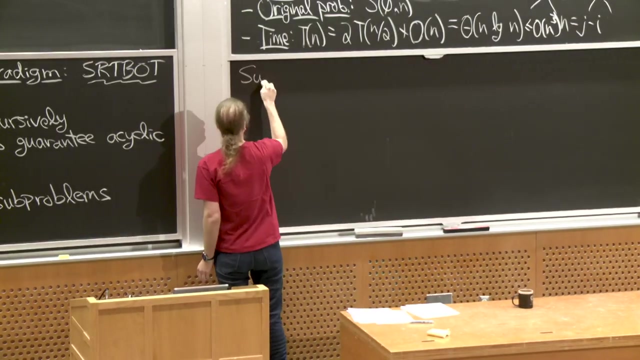 the input is a sequence of numbers, It's a sequence data structure, maybe It's an array of numbers, which is this V array, And let's see A general tool for subproblem design which will cover most of the problems, maybe. 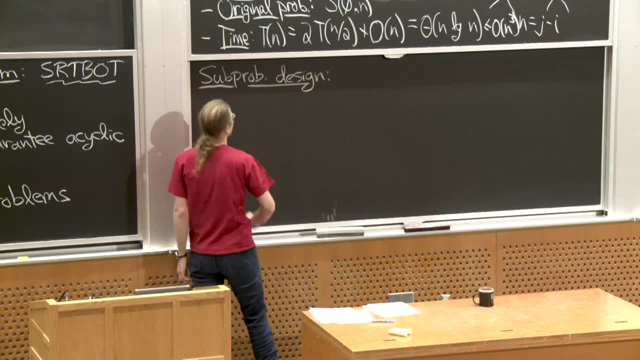 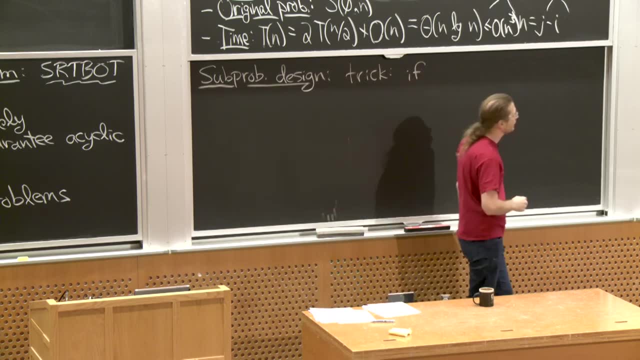 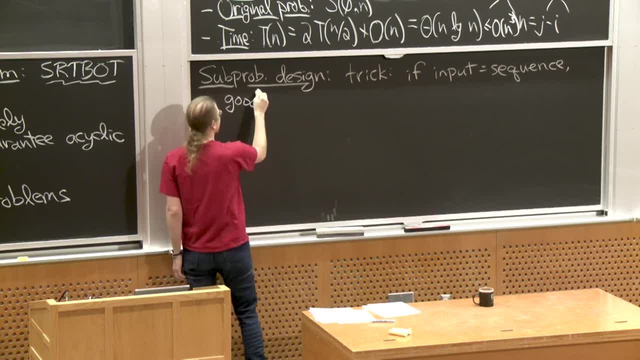 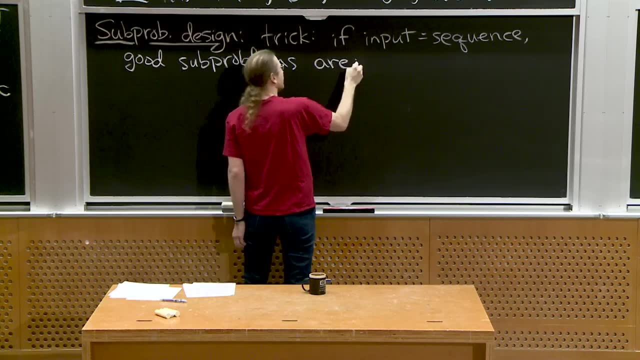 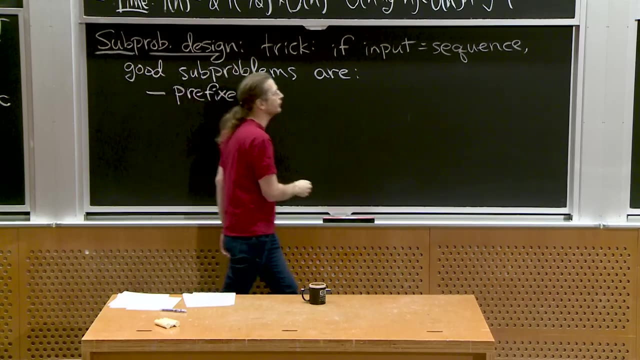 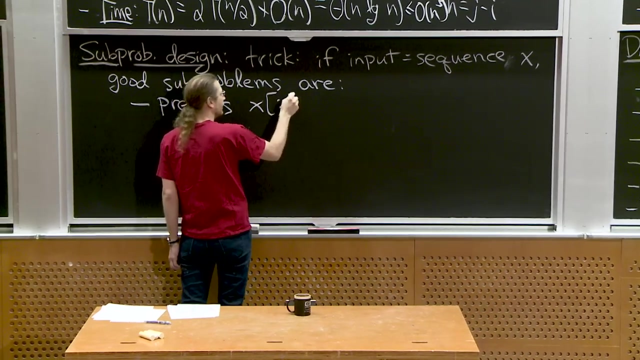 It's a sequence, So here are some good subproblems to consider. We could do all prefixes, So let's call this sequence x, So we could do x. prefix means up to a given i, for all i. We could do all the suffixes. 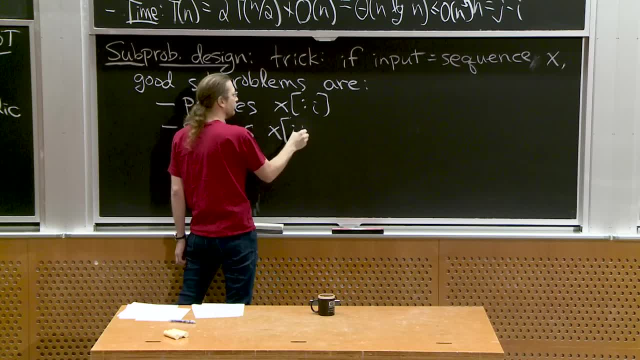 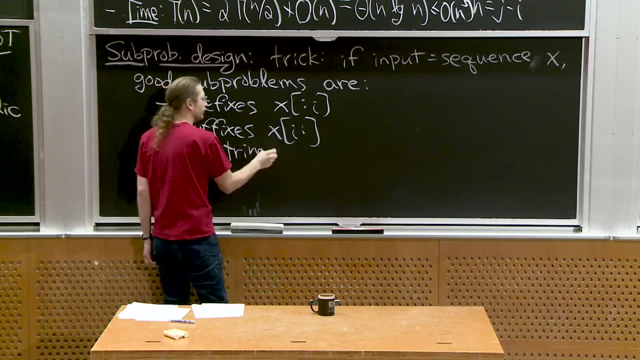 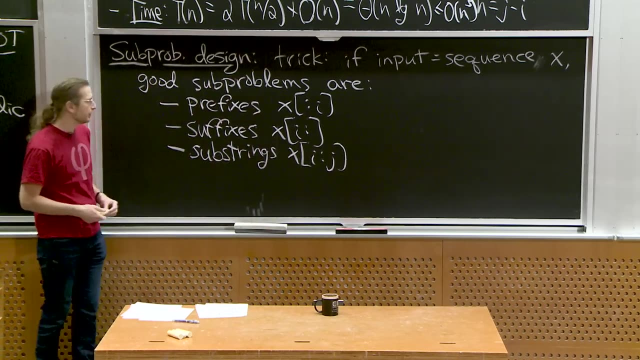 x, from i onward, for all i. Or we could do substrings, which are the consecutive items from i to j. I don't write subsequence here. Subsequence means you can omit items in the middle, So substring. you have to start at some position. 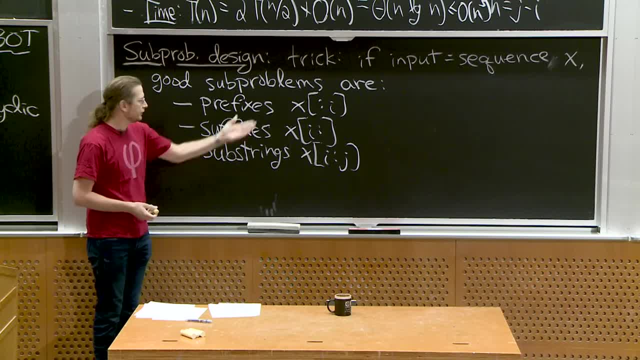 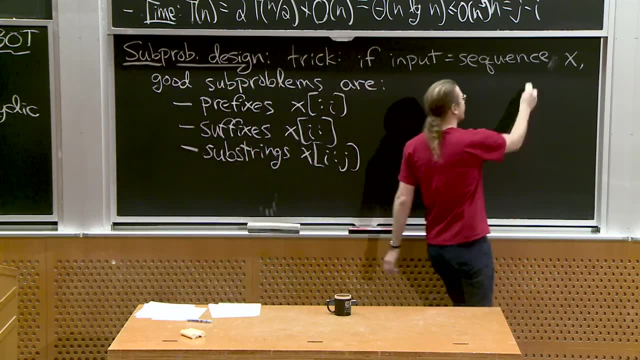 and do all the things up to j. So these are nice easy to express in Python notation And these are great because they're polynomial. If I have n things, if the length of my sequence x is n, then there are n sequences, n prefixes, technically n plus 1.. 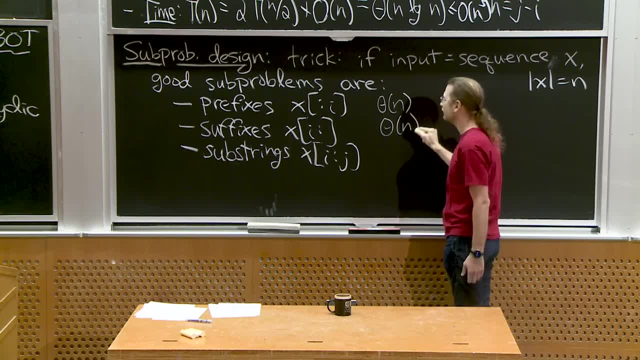 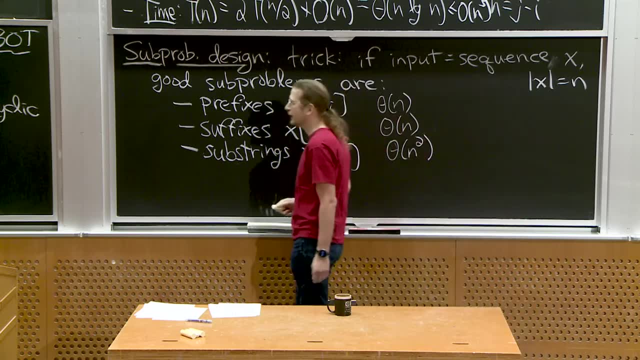 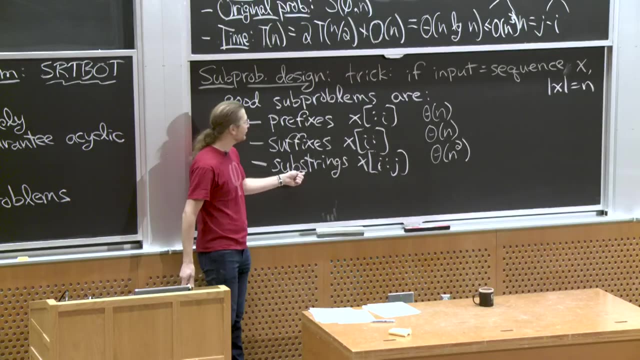 So let's do theta n prefixes. There are theta n suffixes And there are theta n squared substrings, because there's roughly n choices for i and j separately. Sorry, What about subsequences? Subsequences. Good, I didn't write subsequences, because in fact 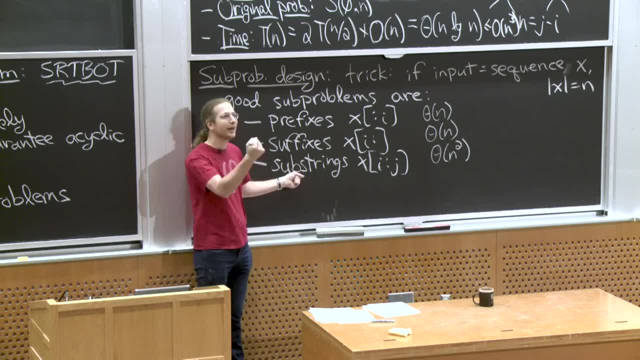 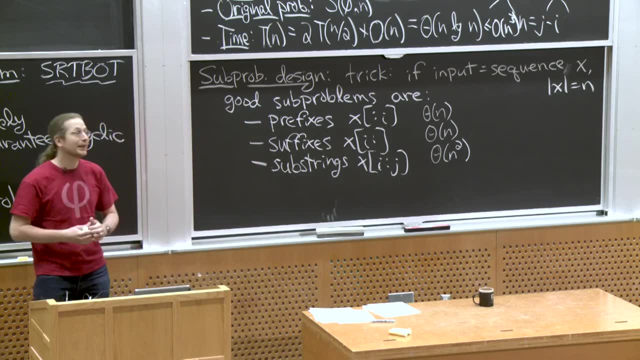 there are exponentially many subsequences. It's 2 to the n For every item. I can choose it or not. So I don't want to parametrize. I don't want my subproblems to be subsequences, because that's guaranteed. 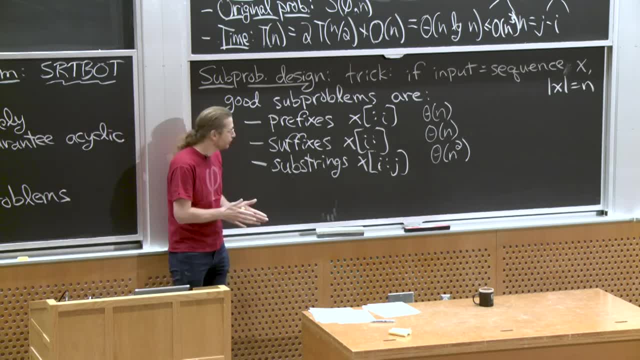 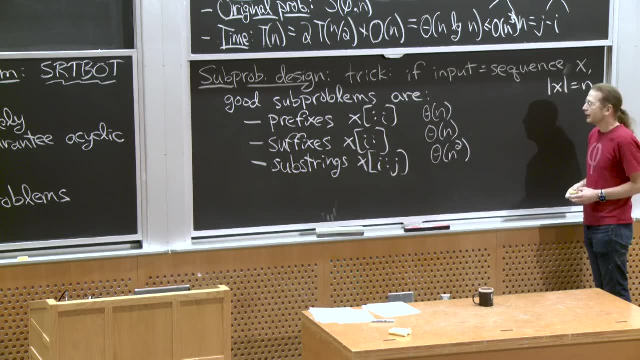 Well then, you're guaranteed to get an exponential number of subproblems, which is bad. We'd like to bound the number of subproblems by a polynomial. So these are three natural ways to get polynomial bounds. Now, prefixes and suffixes are obviously better. 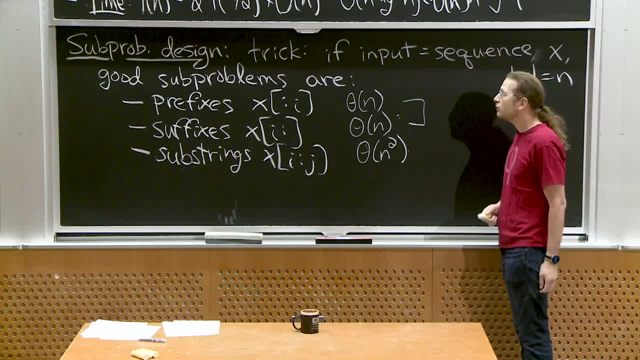 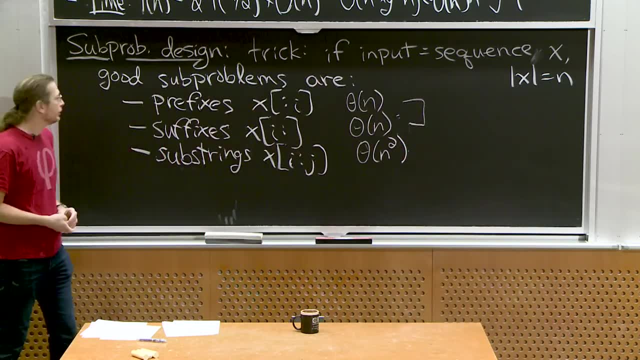 because there's fewer of them- linear instead of quadratic- And usually almost every problem you'll encounter prefixes and suffixes And prefixes are equally good. It doesn't really matter which one you choose. So maybe you like to think of: well, we'll get to it. 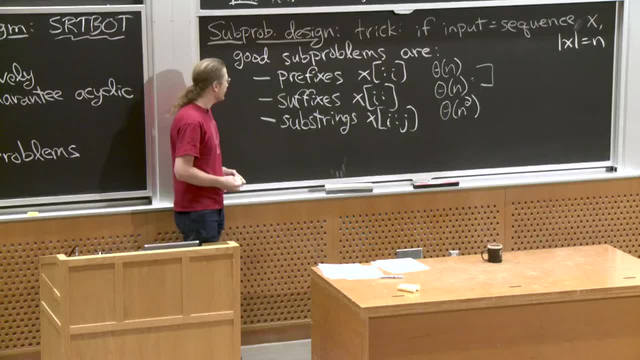 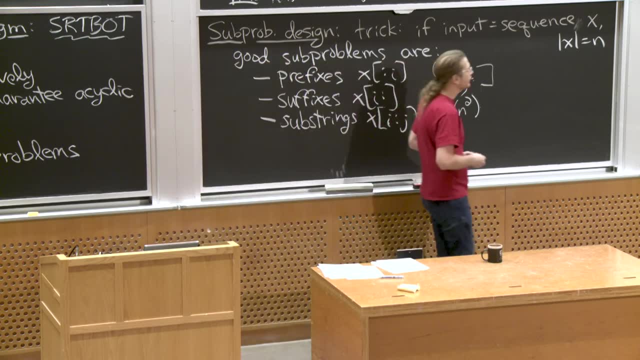 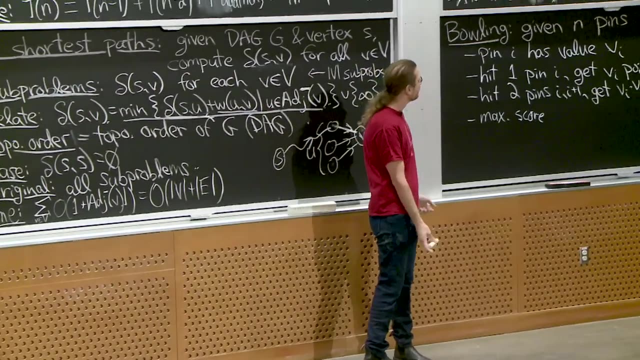 Just choose whichever is more comfortable for you. But sometimes it's not enough and we'll have to go to substrings. That won't be for another lecture or two. Today I claim that prefixes or suffixes are enough to solve the bowling problem. 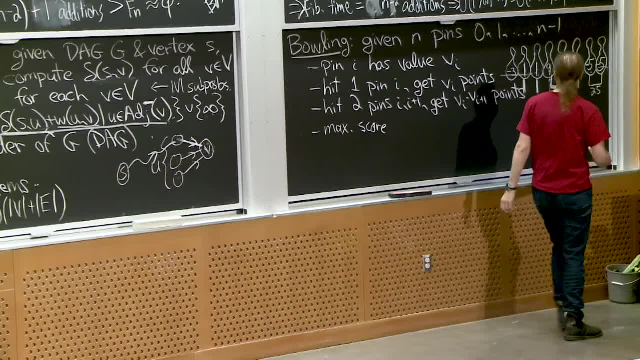 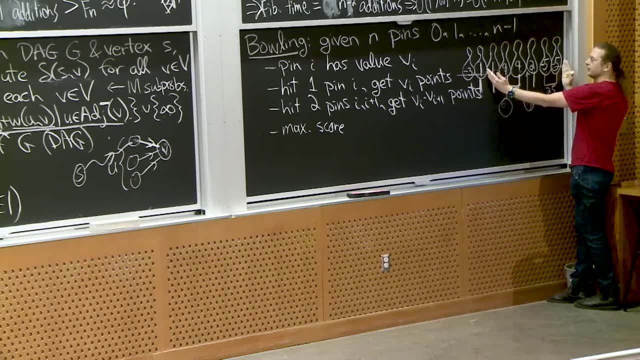 So what we're going to do is think about: I prefer or suffixes, usually because I like to work from left to right, from the beginning to the end. So we're going to think of a suffix of the bowling pins. 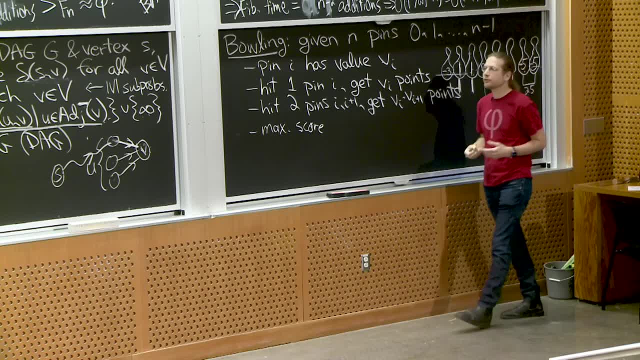 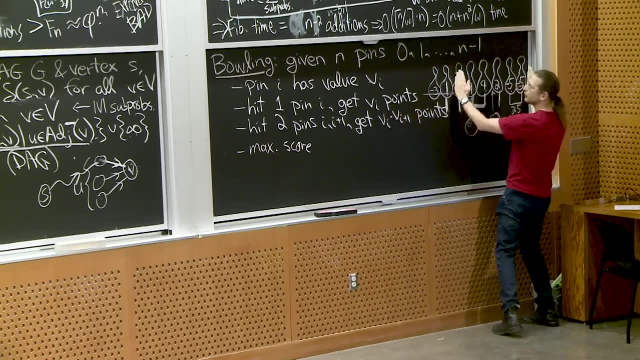 And so what is the subproblem on a suffix? Well, a natural version is just to solve the original problem: bowling. How do I maximize my score if all I were given were these pins? Suppose the pins to the left of i didn't exist. 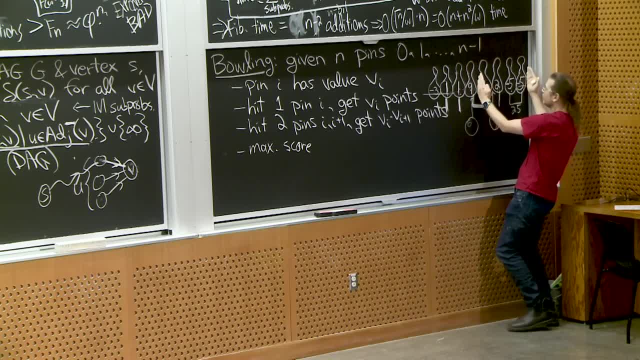 How would I maximize my score on the remaining pins Or for this suffix? given these four pins, what would I do- And there's some weird subproblems here- If I just gave you the last pin? what would you do? Nothing. 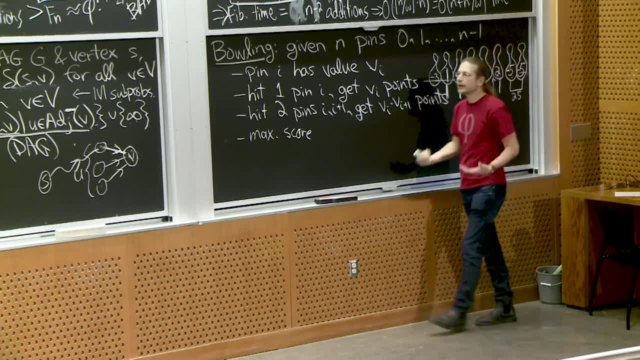 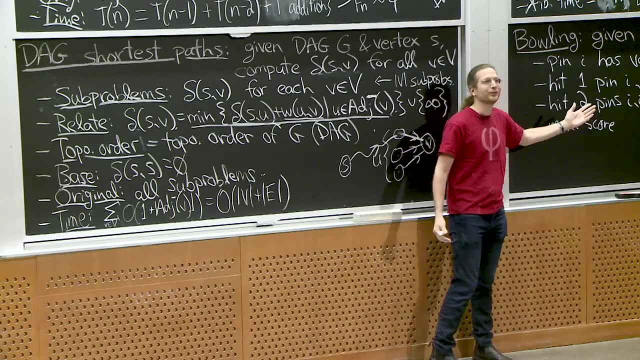 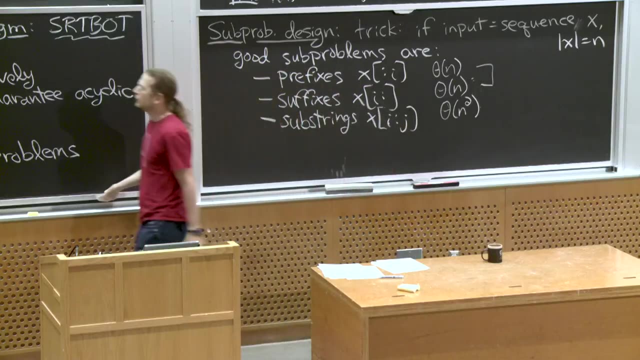 That's clearly different from what I would do globally here. But I claim if I can solve all suffixes, I can solve my original problem, because one of the suffixes is the whole sequence. So let's do it. Sort bot for bowling. 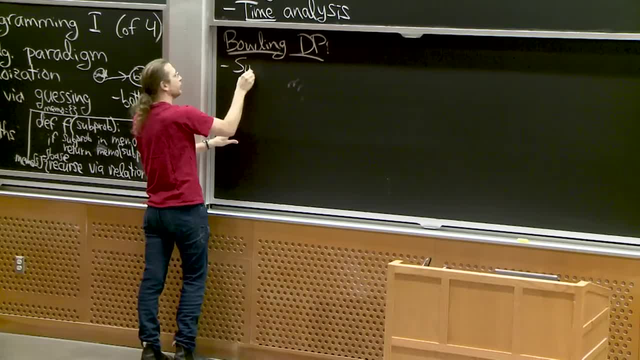 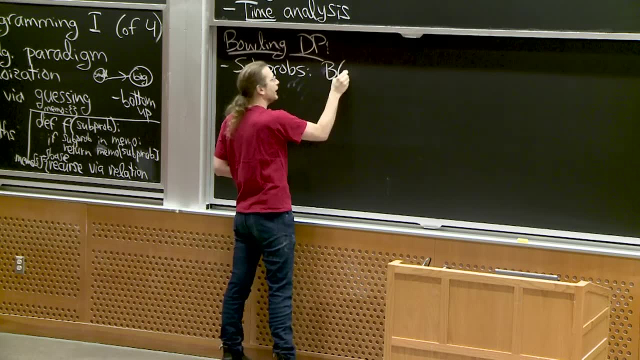 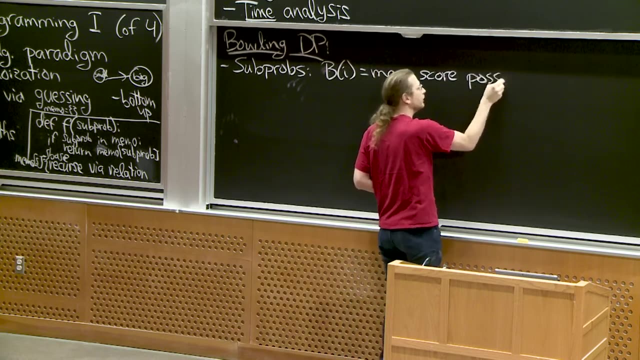 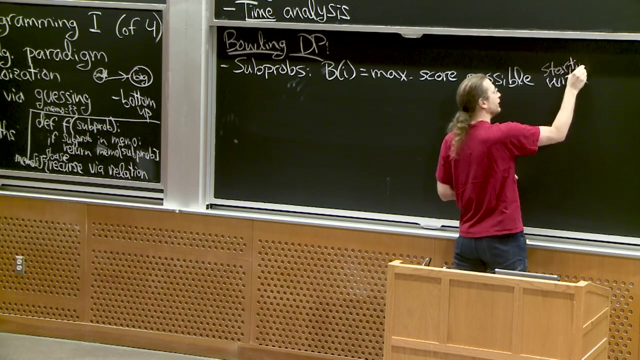 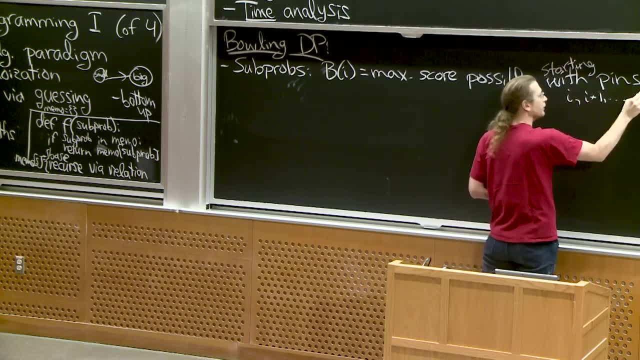 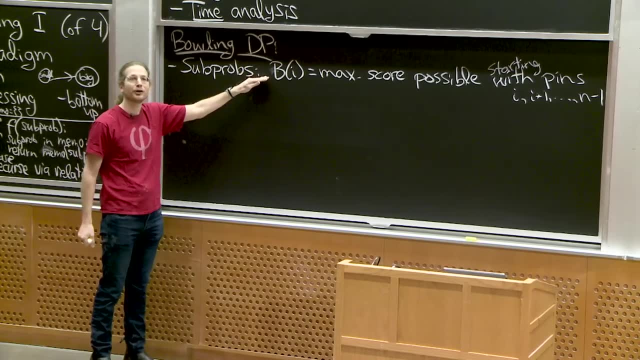 i plus 1.. Up to n minus 1, which is a suffix of the pins. Very important: whenever you write a dynamic program to define what your subproblems are, Don't just say how to compute them, but first say what is the goal of the subproblem. 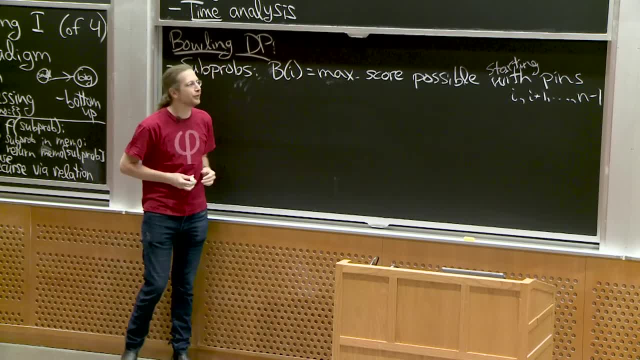 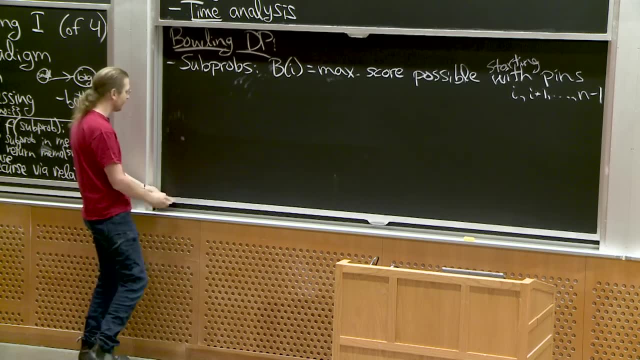 This is a common mistake: to forget to state what you're trying to do. So now I've defined b of i. Now what is the original thing I'm trying to solve? I like to. you can also put in sort bot. you could put the o earlier. 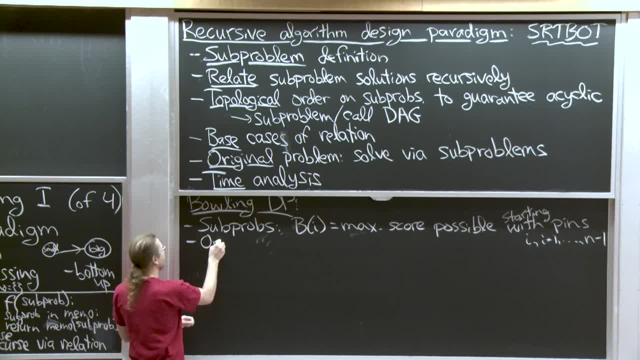 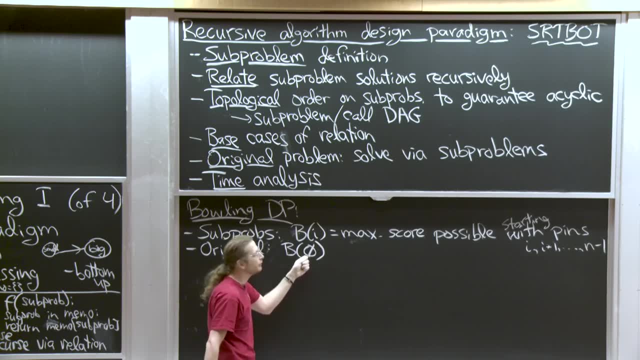 Then it actually spells sort. So why don't I do that for fun? The original problem we're trying to solve is b of 0. Because that is all of the pins. The suffix starting at 0 is everything. So if we can solve that, we're done. 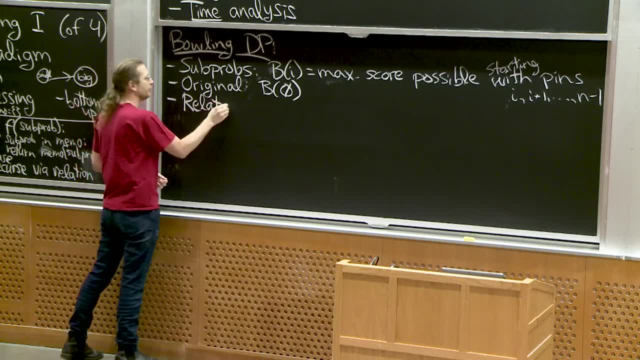 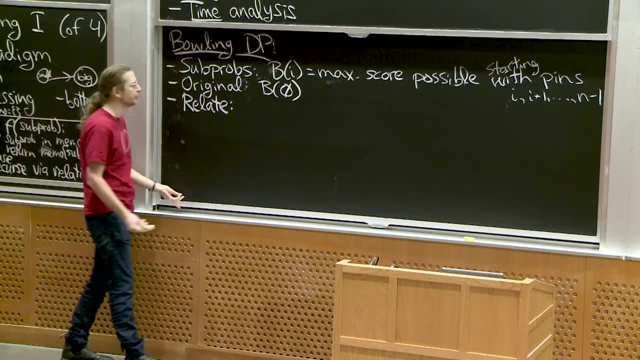 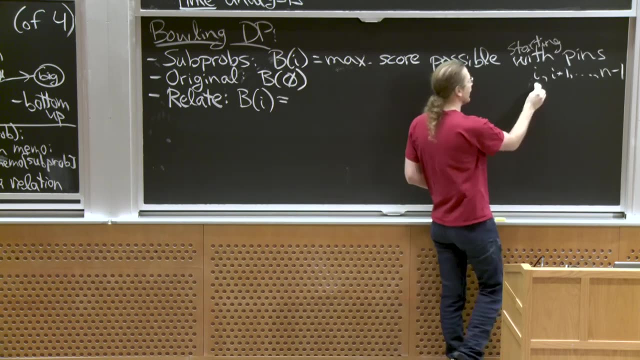 Next is r for relate. This is the test of: did I get the subproblems right is whether I can write a recurrence relation. So let's try to do it. We want to compute b of i, So we have pin i here and then the remaining pins. 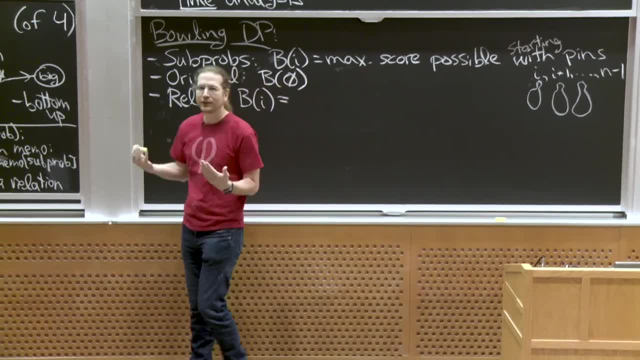 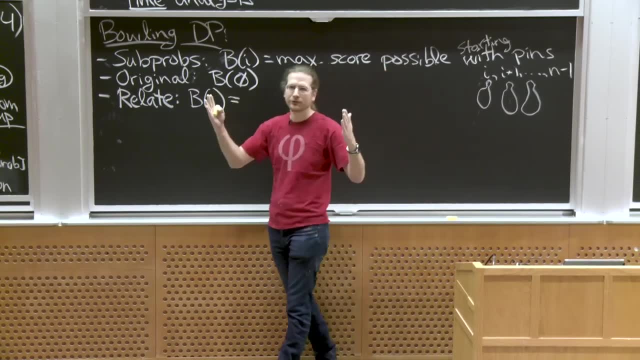 And the big idea here is to just think about the nice thing about suffixes is, if I take off something from the beginning, I still have a suffix. Remember, my goal is to take this subproblem, which is the suffix starting at i, and reduce it. 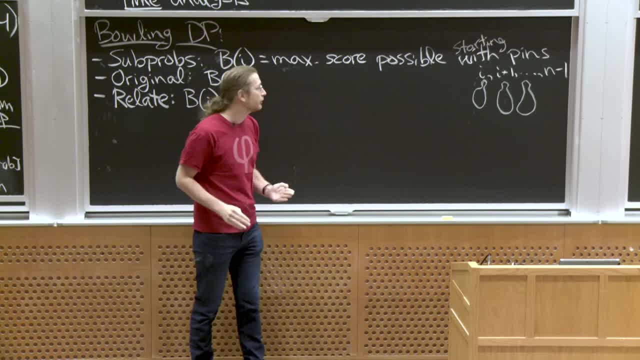 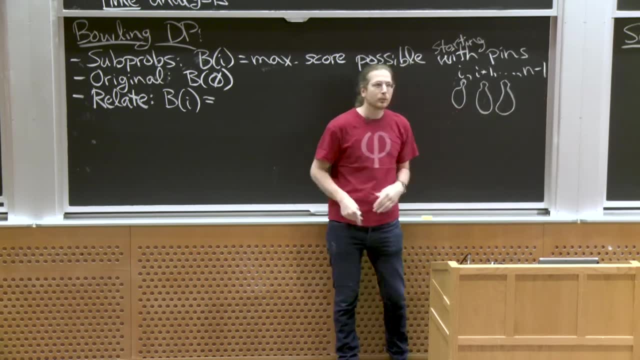 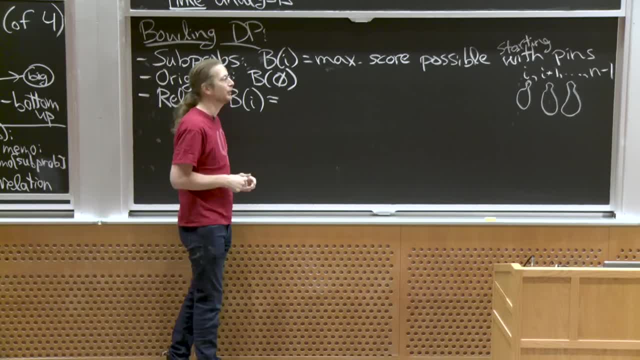 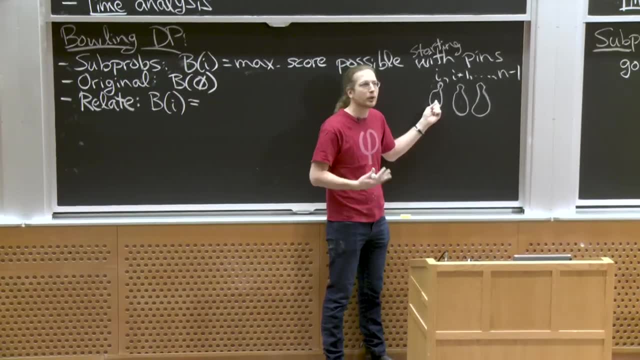 or sorry, b, of something larger than i will be a smaller subsequence because we're starting later. So what could I do? Well, the idea is to just look at pin i and think: well, what could I do to pin i? 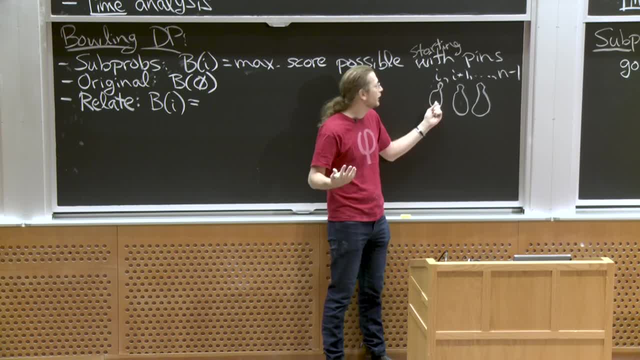 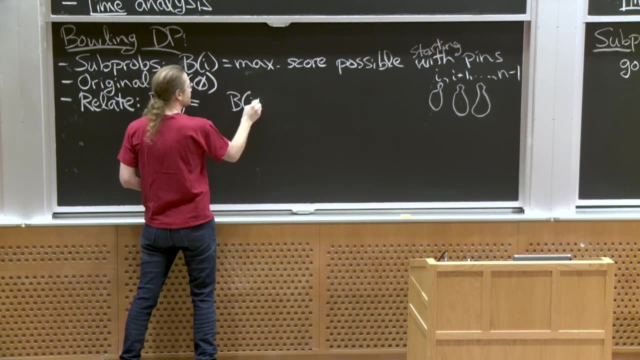 I could not hit it ever with a ball. I could skip it. That's one option. What would be my score Then? well, if I skip pin i, that leaves the remaining pins, which is just a smaller suffix. So that is b of i plus 1.. 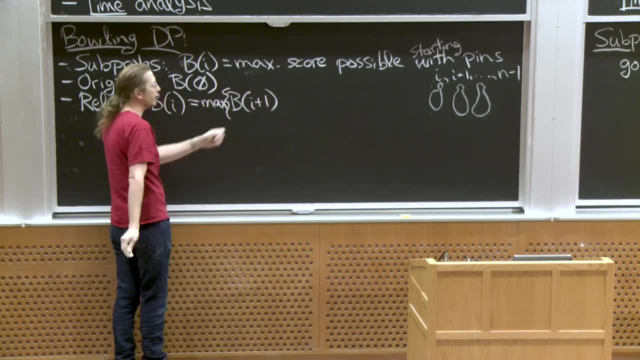 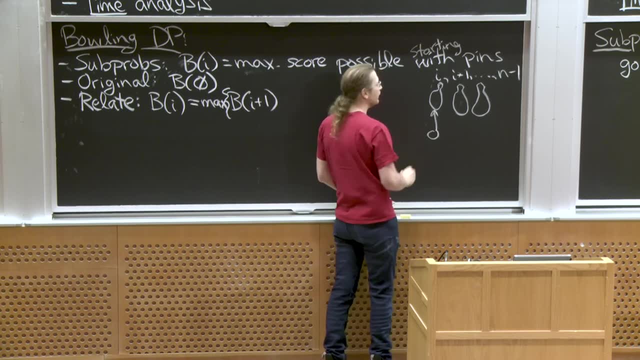 I'm going to write a max out here because I'd like to maximize my score, And one of the options is: forget about pin i, Just solve the rest. Another option is I throw a ball and I exactly hit pin i. That's a thing I could do. 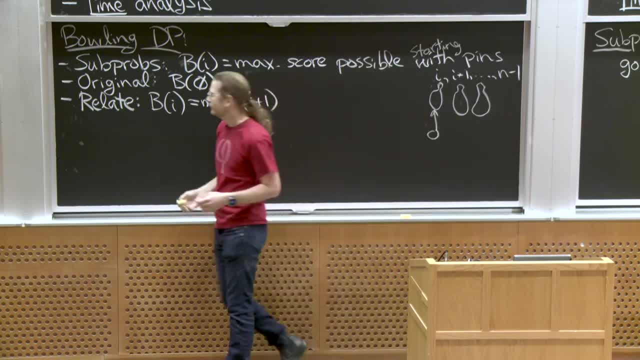 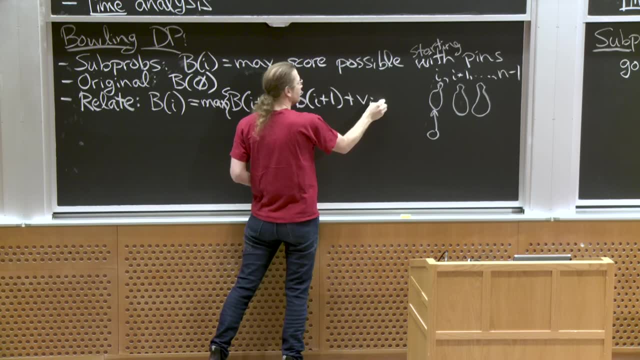 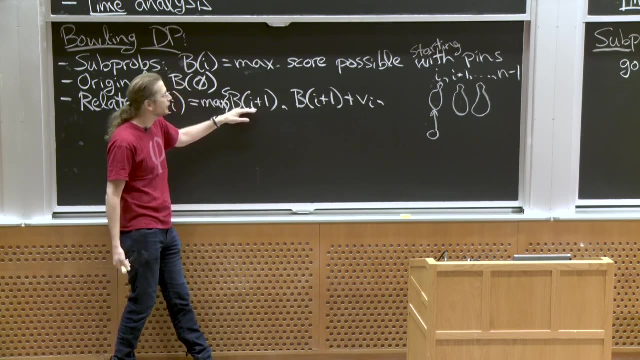 And it would leave exactly the same remainder. So another option is b of i plus 1 plus v i. Why would I prefer this over this? Well, if v i is negative, I'd prefer this, But if v i is positive, I'd actually. 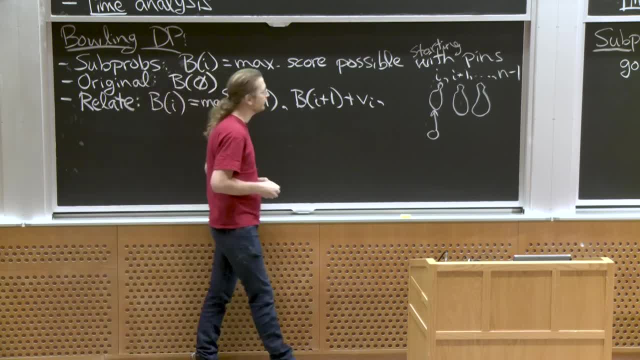 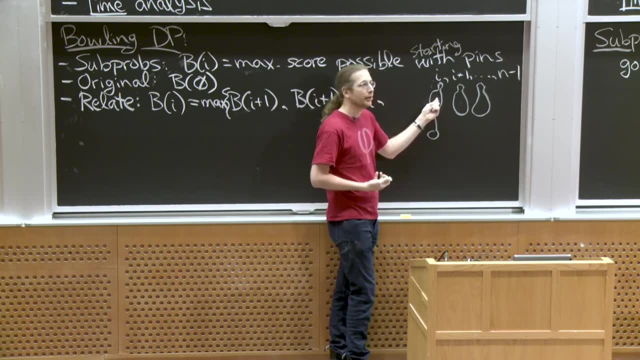 prefer this over that, So you can figure out which is better just locally. But then there's another thing I can do, which is maybe I hit this pin in a pair with some other pin. Now there's no pin to the left of this. 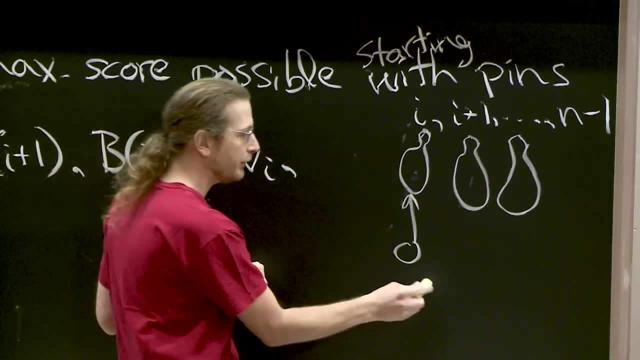 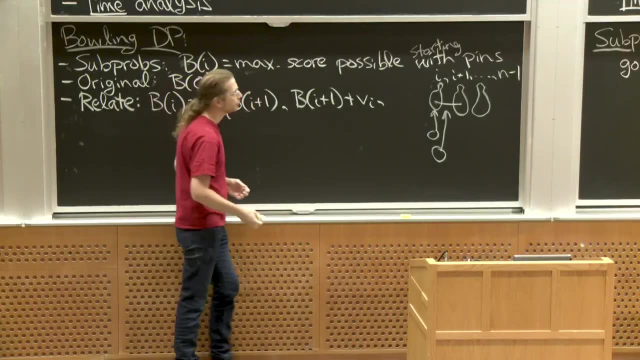 This one, We're assuming we only have the suffix, And so the only other thing I can do is throw a ball and hit i together with i plus 1.. And then I get the product. Now, what pins remain? i plus 2 on. 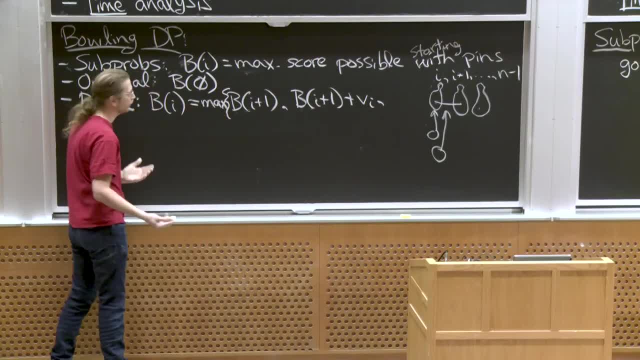 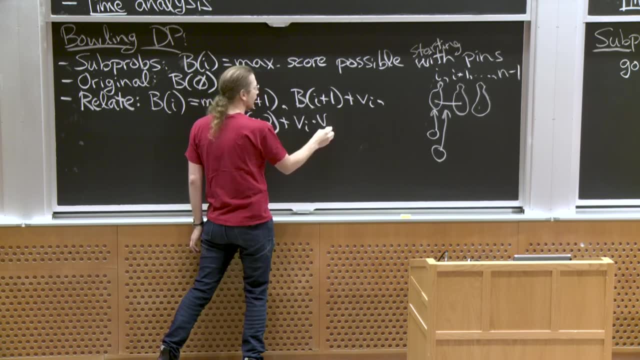 Still a suffix. So if I remove one or two items, of course I still get a suffix, in this case b of i plus 2.. And then the number of points that I add on are v? i times v? i plus 1.. 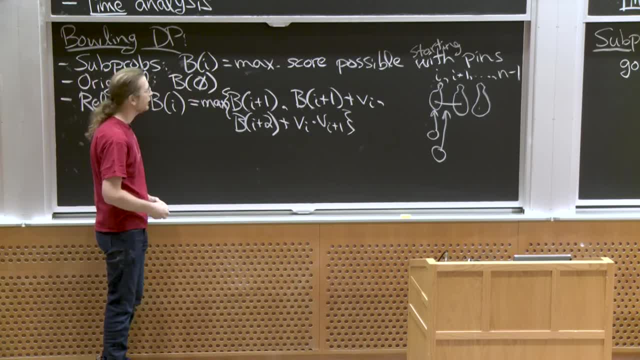 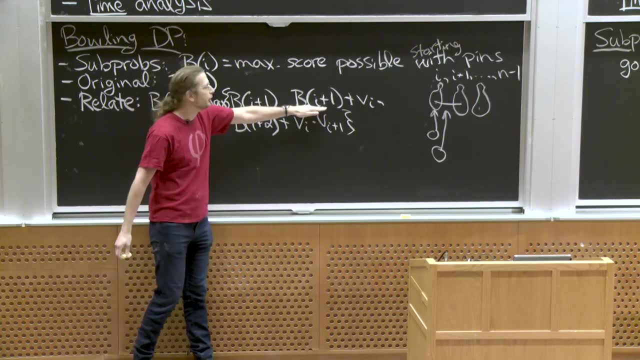 So this is a max of three things. So how long does it take me to compute it? I claim constant time, If I don't count the time it takes to compute these other subproblems which are smaller, because they are smaller suffixes further to the right. 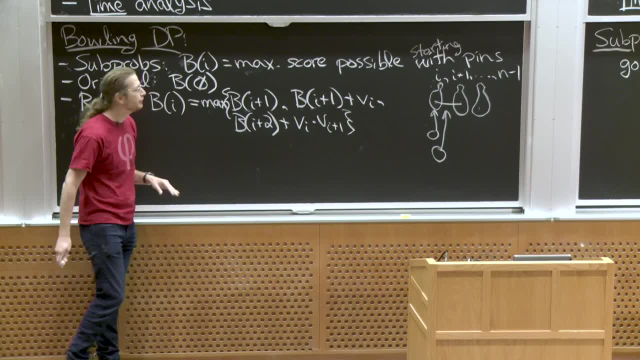 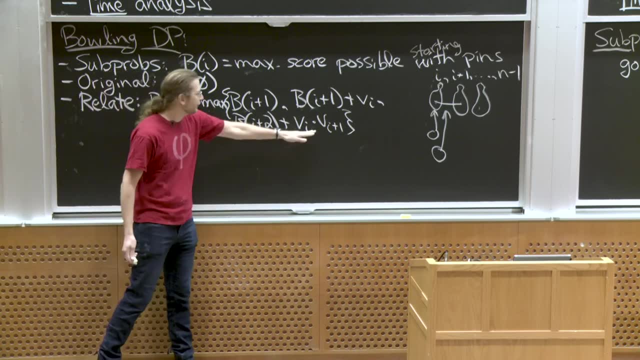 then I'm doing a couple of additions: product max- These are all nice numbers. They will assume that they live in the w-bit word because they were only doing constant size products. That's good. So this takes constant, non-recursive work. 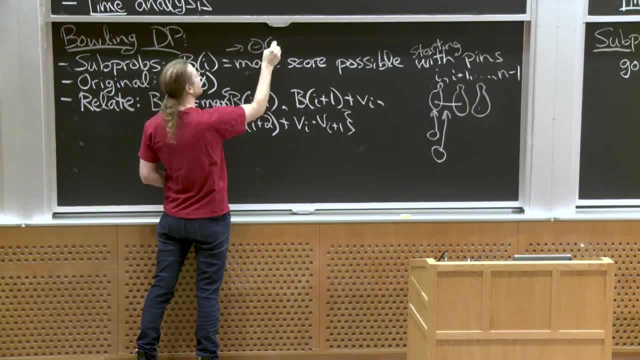 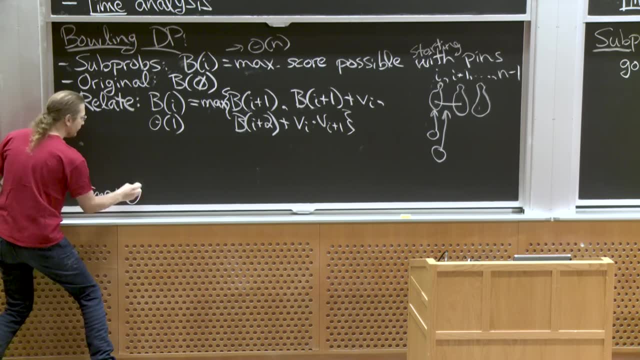 Now how many subproblems are suffixes. So it's a linear number of subproblems, And so the time I'm going to end up meeting is the number of subproblems n times the non-recursive work I do per subproblem, which is constant. 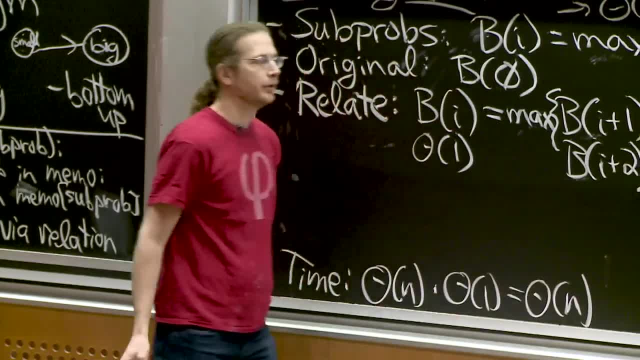 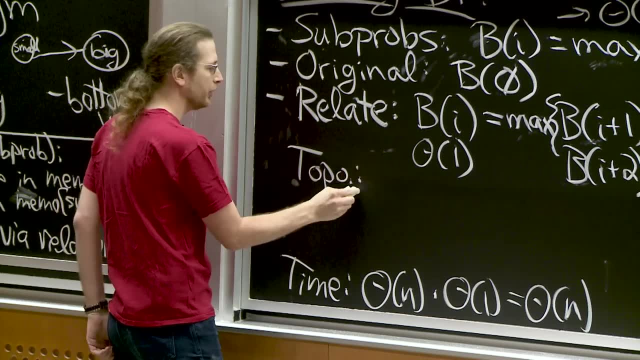 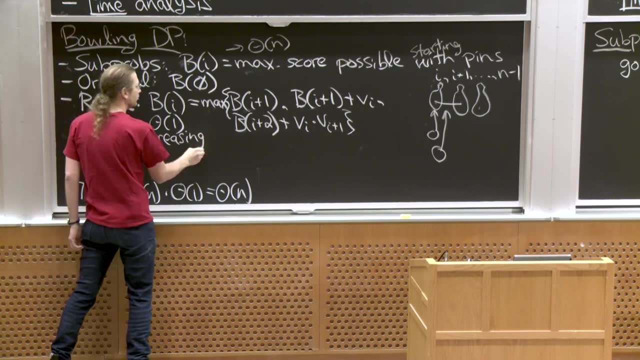 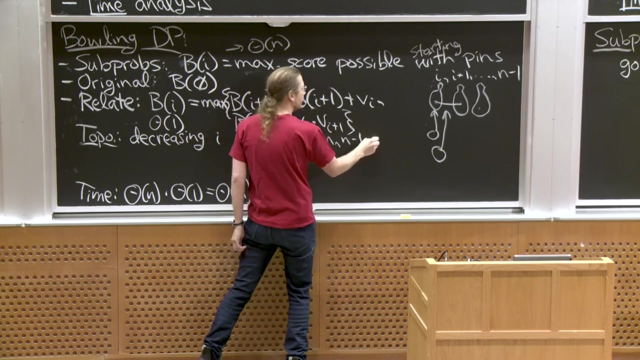 And so this is linear time. Great, Now I didn't finish sort bot. So there's another t, which is to make sure that there is a topological order, And that is in In decreasing i order, Or I might write that as a for loop, for i equals n, n minus 1.. 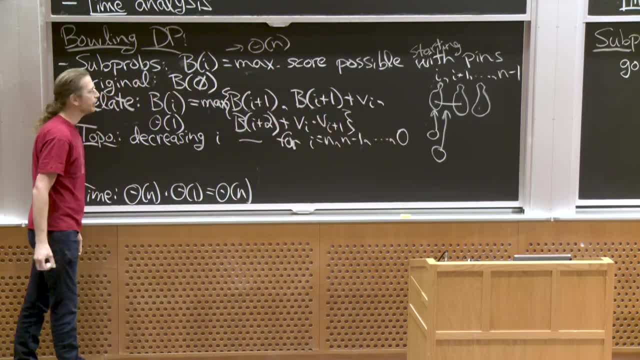 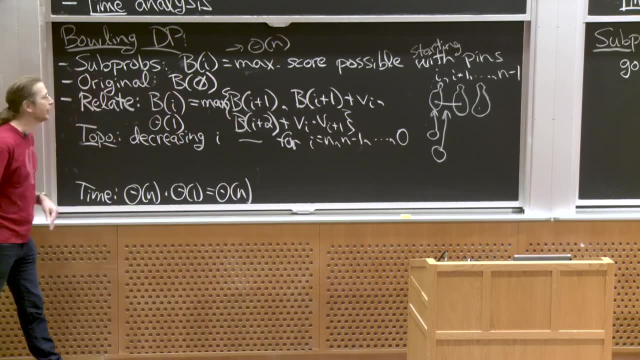 This is the order that I would compute my problems, because the suffix starting at n is the empty suffix, The suffix starting at 0, that's the one I actually want to compute. That's the final suffix I should be computing. And then we have a b for base case, which is 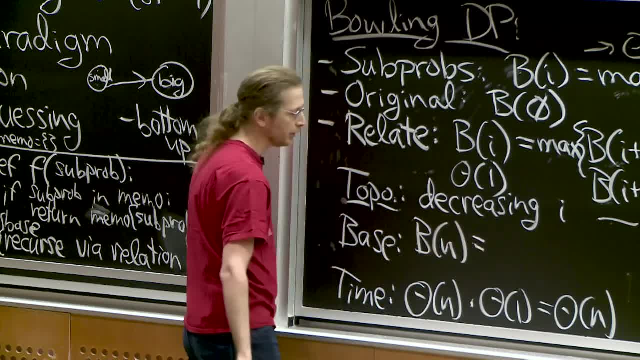 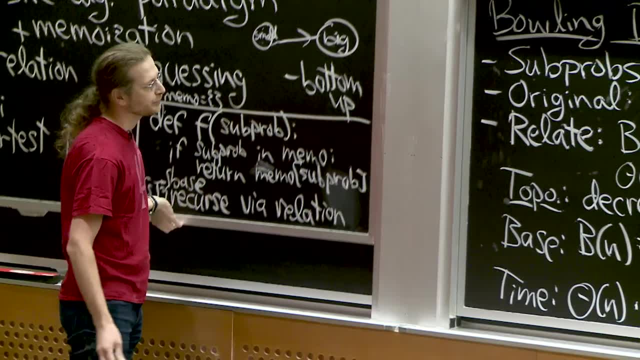 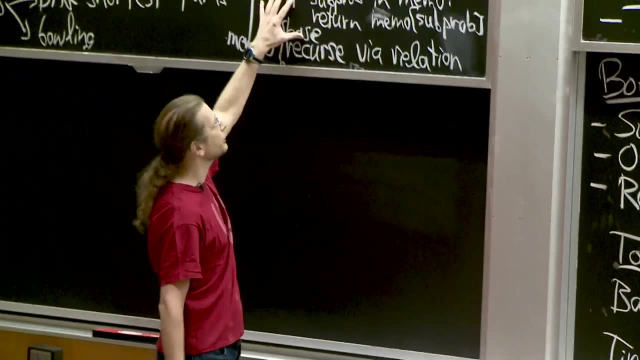 in that first case, b of n equals 0, because there's no pins, so I don't get any points, Sad. So this is it. We just take these components, plug them into this recursive memoized algorithm and we have a linear time algorithm. 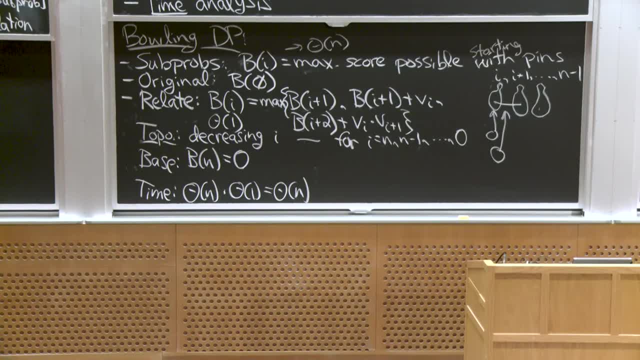 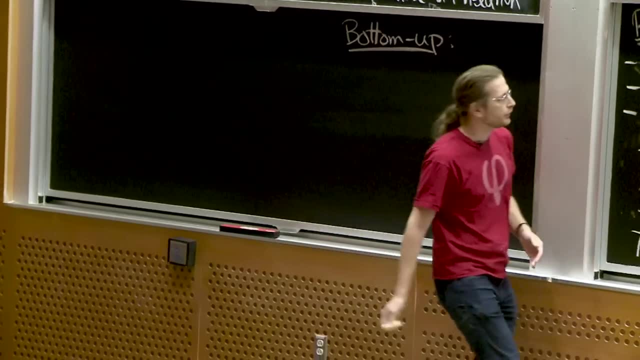 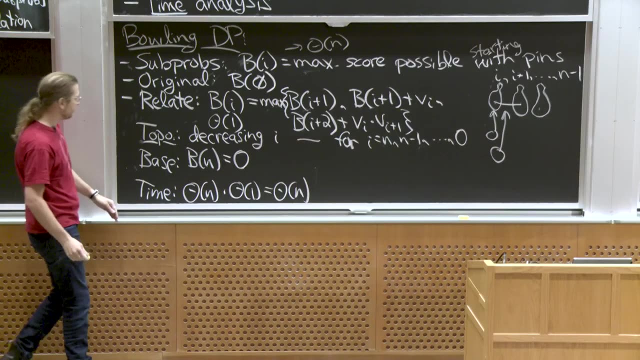 I want to briefly mention a different way you could plug together those pieces which is called bottom up dp, Which is: let's do it for this example. So if I have, let's see. let me start with the base. case b of n equals 0.. 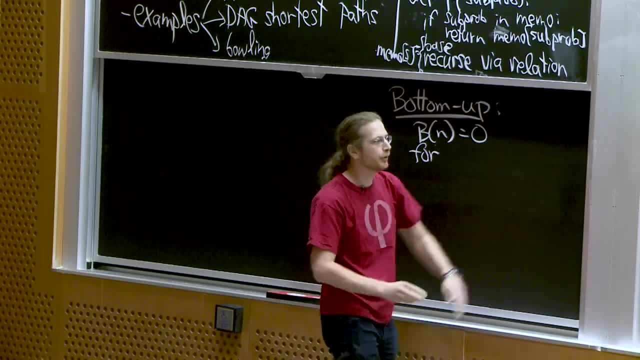 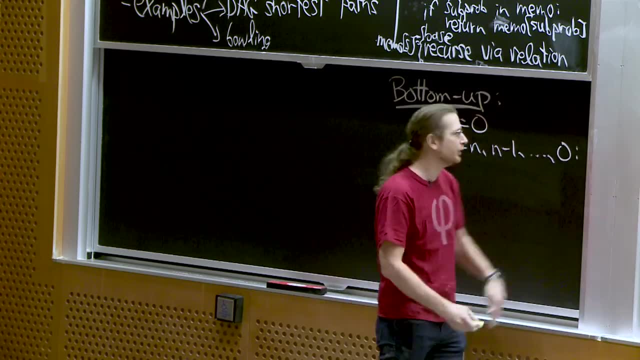 But now it's an assignment And I'm going to do the for loop from the topological order for i equals n, n minus 1 to 0.. Now I'm going to do the relation b of i equals max of. 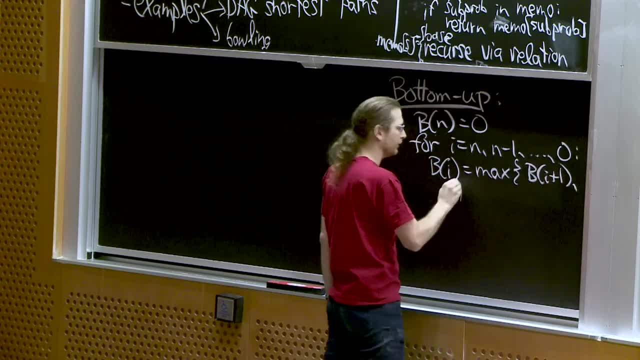 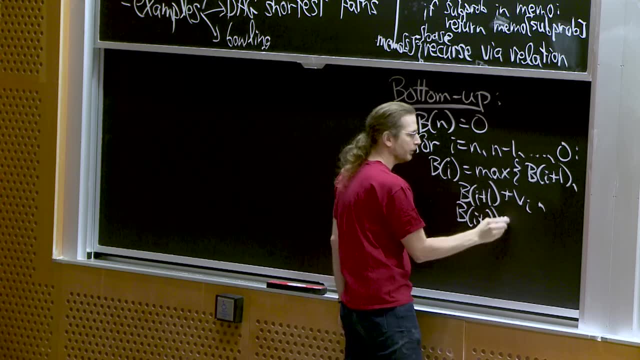 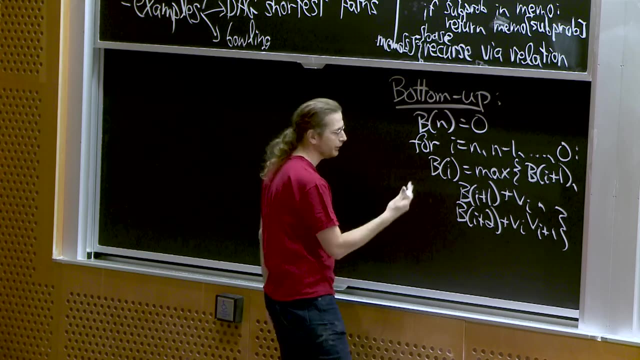 Of b of i plus 1, and b of i plus 1 plus vi and b of i plus 2 plus vi, vi plus 1.. Technically this only works if i is strictly less than n minus 1.. So I should have an if i is less than n minus 1. 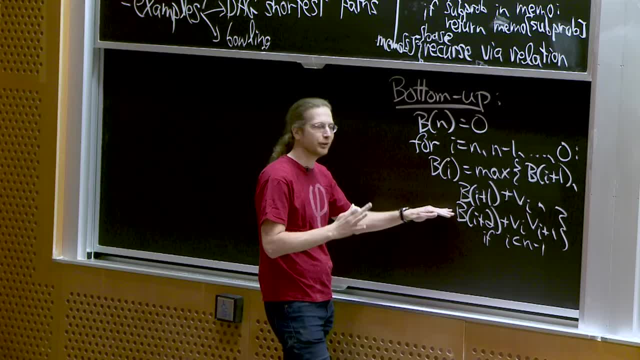 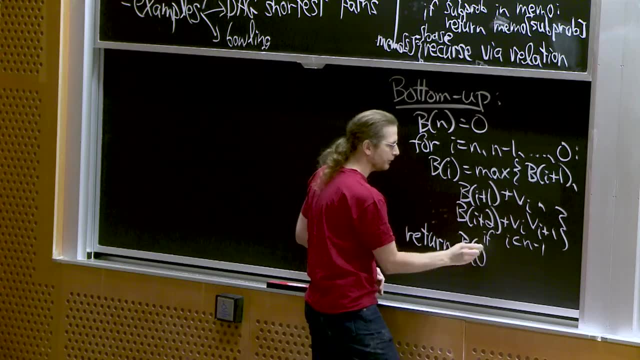 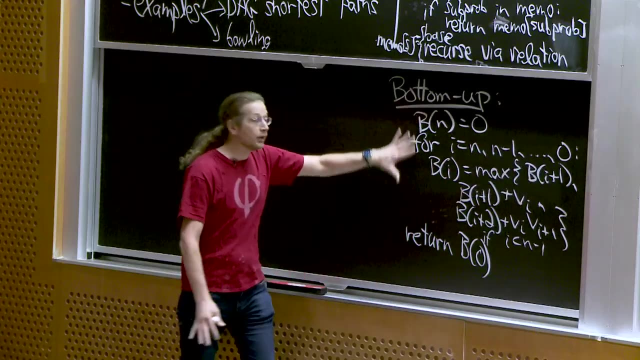 for that last part, because I can only hit two pins if there's at least two pins left, And then return, Return, Return, Return b of 0.. So what I just did is a transformation from this sort bot template into a non-recursive algorithm. 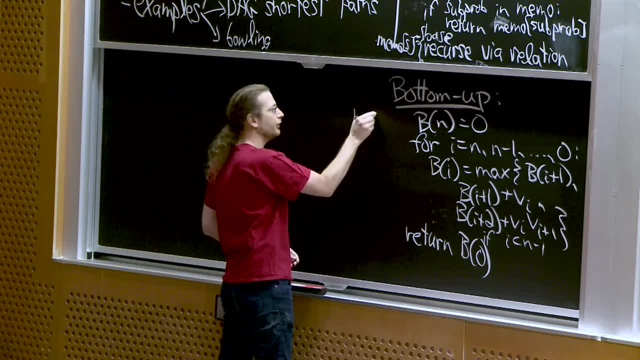 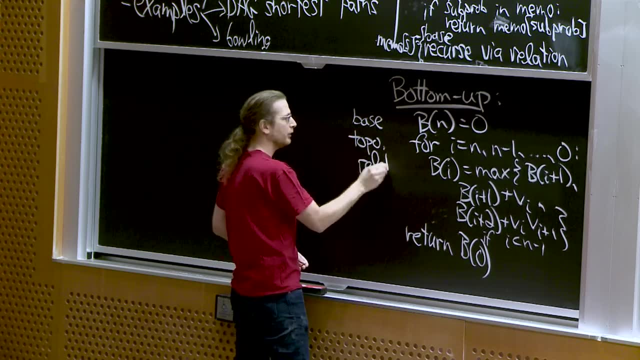 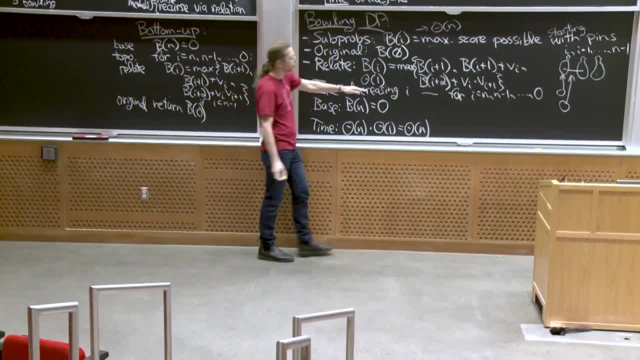 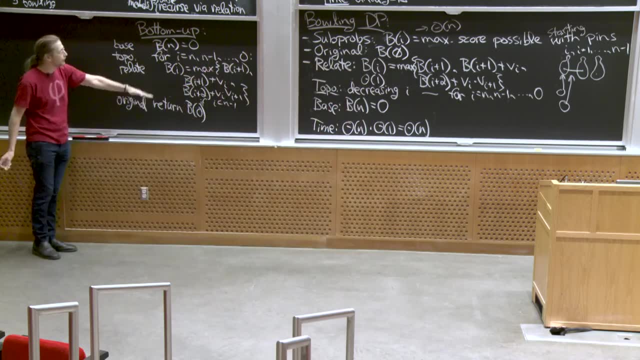 The original problem And it provides a solution And, provided you can write your topological order as some for loops, this is actually a great way to write down a DP as code. If I were going to implement this algorithm, I would write it this way, because this is super fast. 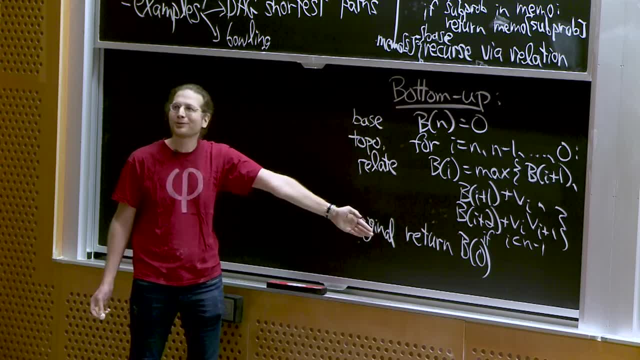 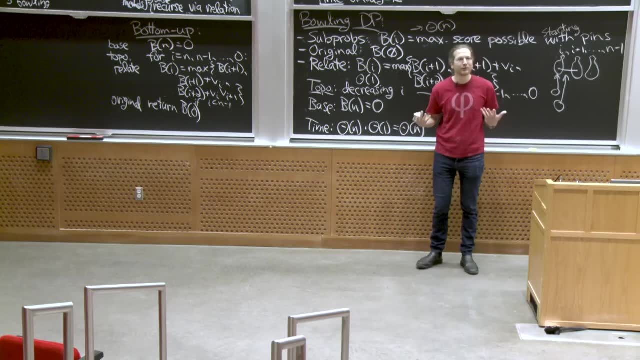 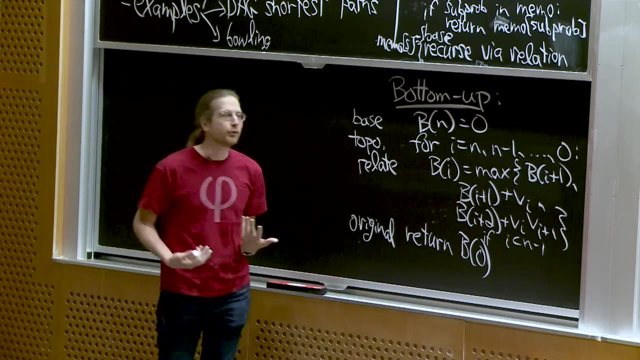 No recursive calls, just one for loop. In fact, this is almost a trivial algorithm. It's amazing that this solves the bowling problem. It's in some sense, considering every possible strategy I could for bowling these pins. What we're using is what we like to call local brute force, where, when we think about pin, 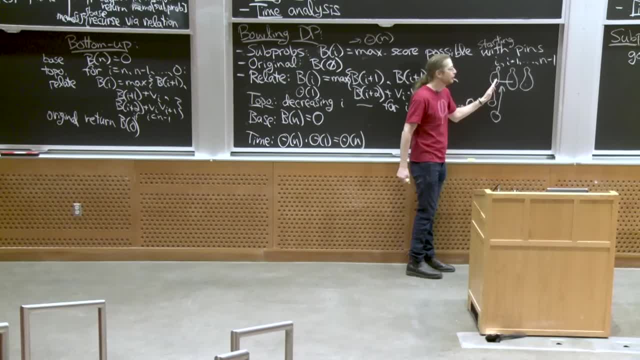 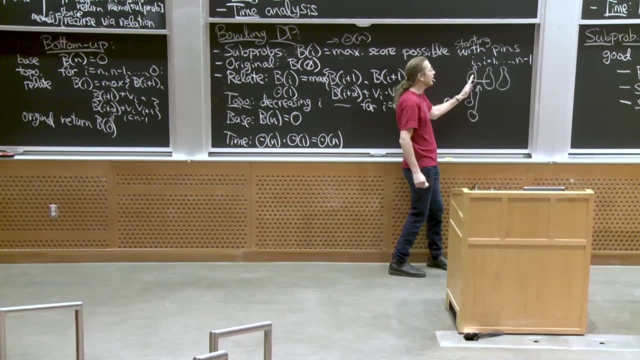 we think about pin i, we look at all of the possible things I could do to pin i. Here there's really only three options of what I could do Now normally if I tried all the options for pin i and then all the options for i plus 1, and i plus 2, and so on. 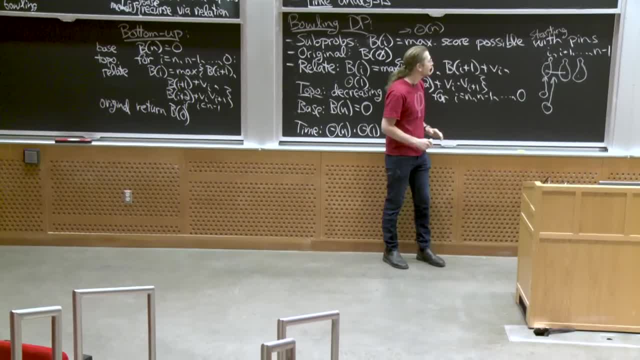 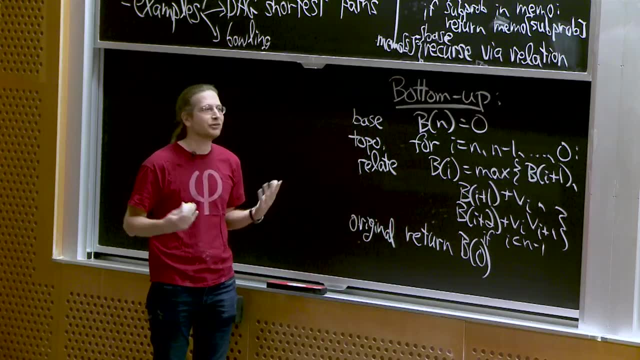 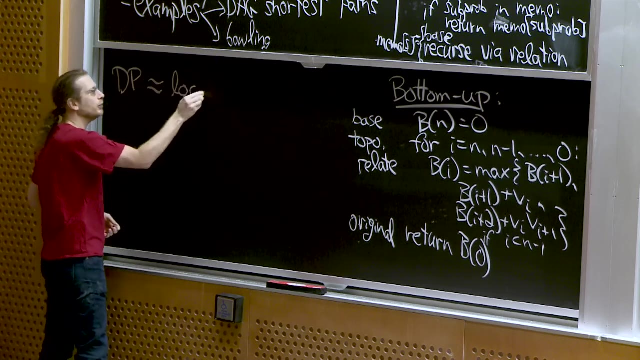 that would be exponential. It'd be 3 times 3 times 3.. That's bad, But because I can reuse these subproblems, it turns out to only be linear time. It's almost like magic. dp is essentially an idea of using local brute force. 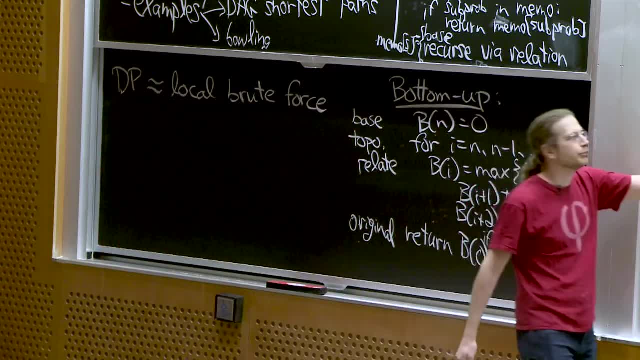 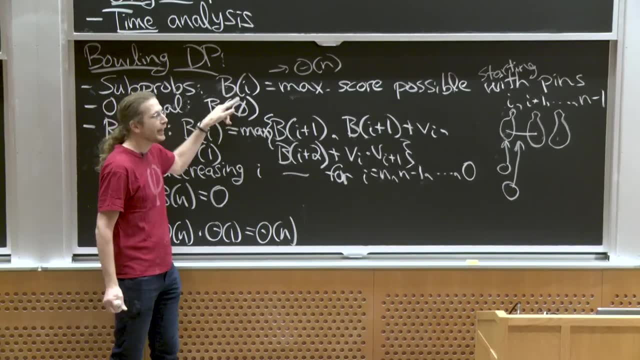 And by defining a small number of subproblems up front, and as long as I stay within those subproblems, as long as I'm always recursing into this polynomial space, I end up only doing polynomial work, even though I'm in some sense exploring exponentially. 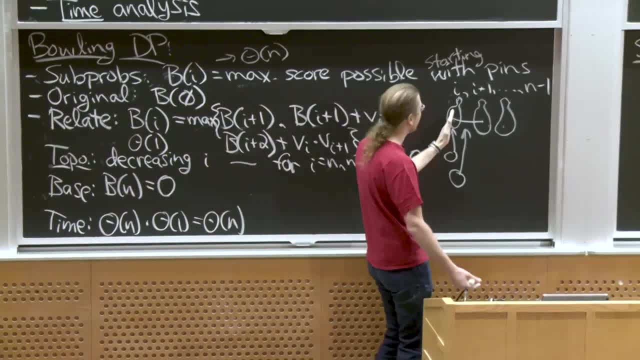 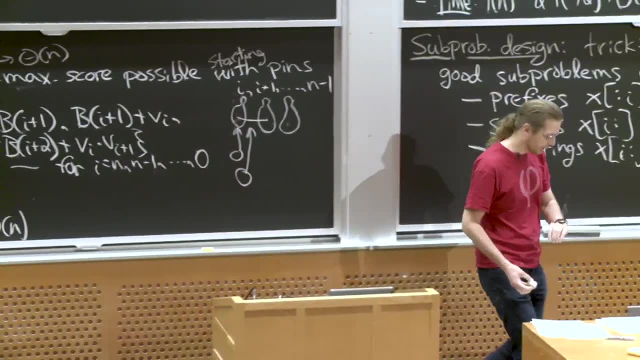 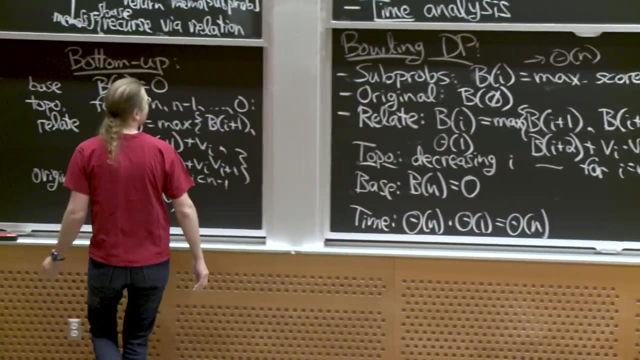 many options, And it's because what I do to this pin doesn't depend too much to what I do to a pin much later, And there's a lot of intuition going on here for when dp works. But we're going to see a lot more examples of that coming up. 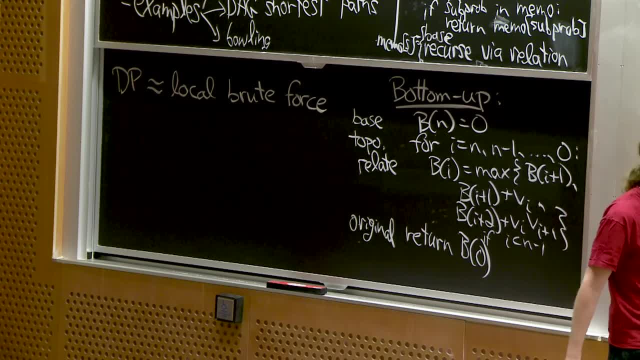 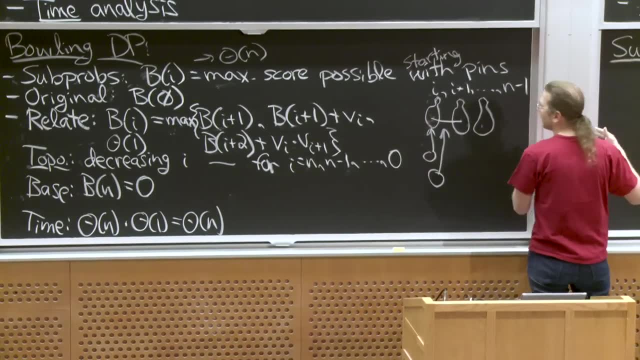 And I just want to mention that the intuition for how to write a recurrence like this is to think about. in the case of suffixes, you always want to think about the first item, or maybe the first couple items. In the case of prefixes, you always think about the last item. 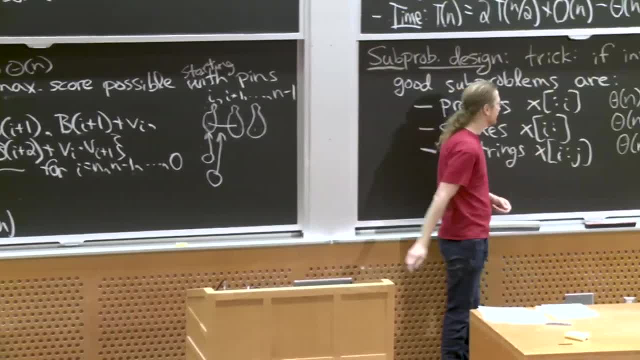 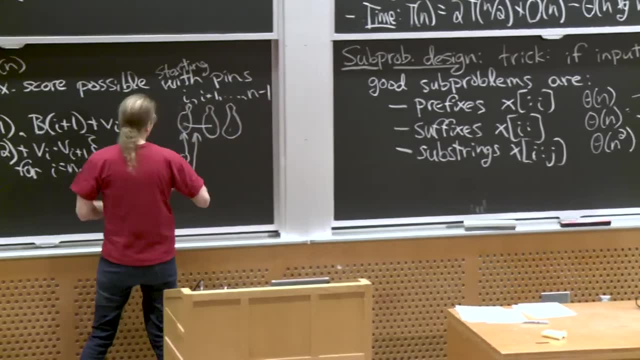 last item And for substrings it could be any item, maybe in the middle. If I remove an item from the middle of a substring I get two substrings. so I can recurse Here or in general what we want to do. 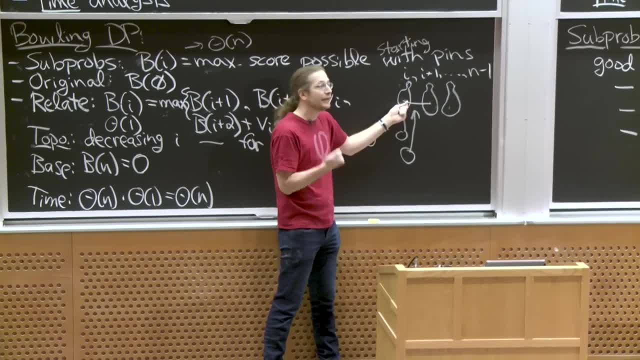 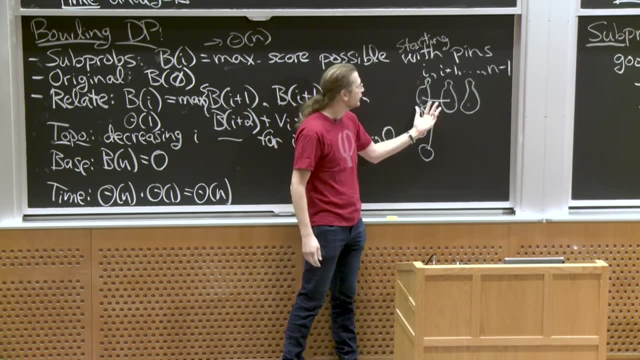 is identify some feature of the solution that if we knew that feature we would be done, We would reduce to a smaller subproblem. In this case we just say: well, what are the possible things I could do? to the first pin.